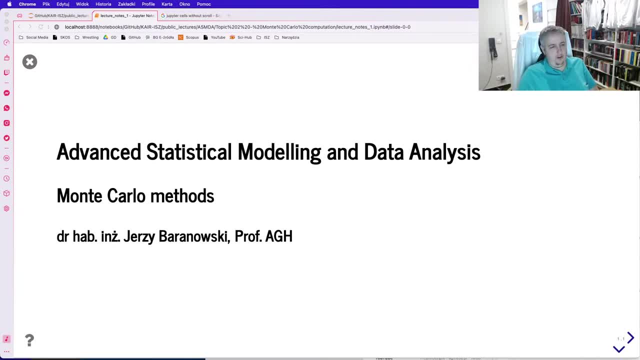 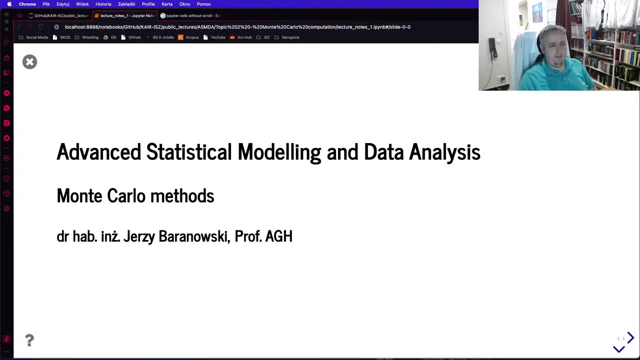 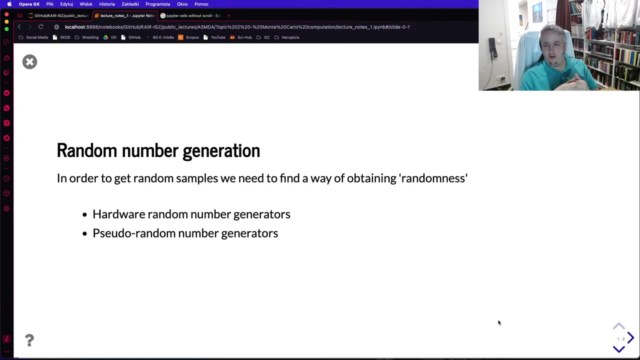 I intended to fit also the Hamiltonian Monte Carlo here, but probably it will be on the next week lecture. So without further ado, let's move to the topic. Generally, as we've said on the previous lecture, we had an issue that if we wanted to do a random number generation, 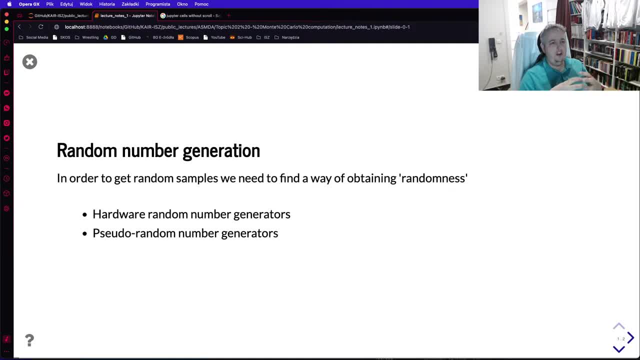 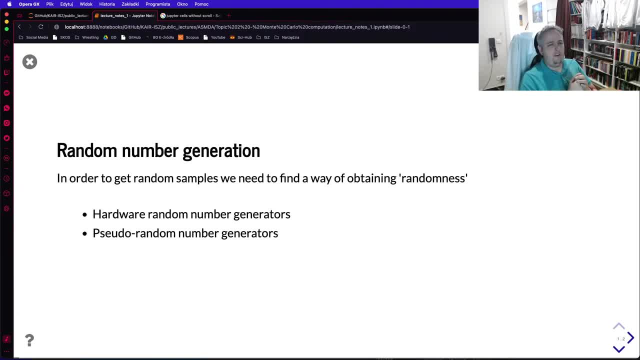 And there are two options really that we have, And there are two options really that we have In current state of technology of obtaining random numbers is either through hardware random number generators or pseudo random number generators. Hardware random number generators are: 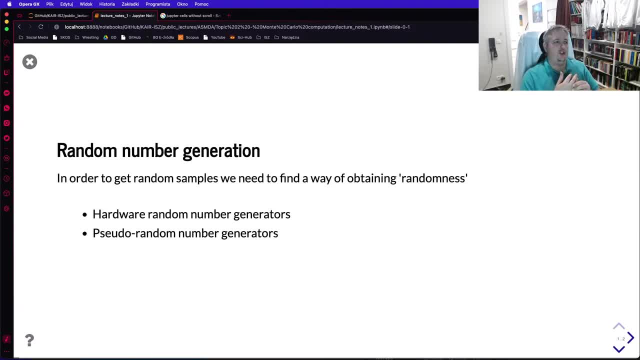 periphery cards or electronic devices which can generally, for example, a noisy diode, which is then sampled through the digital converter, and then you get those values of noisy voltage as a random number which you can then transform to a different way. 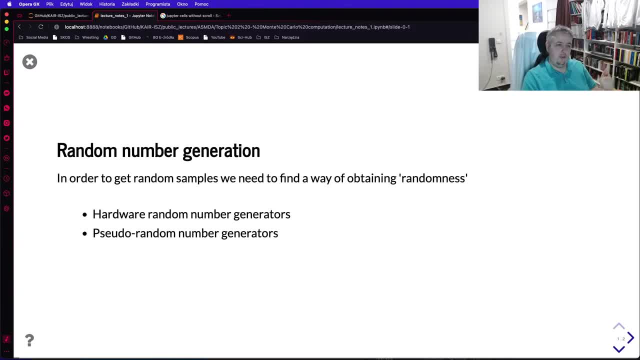 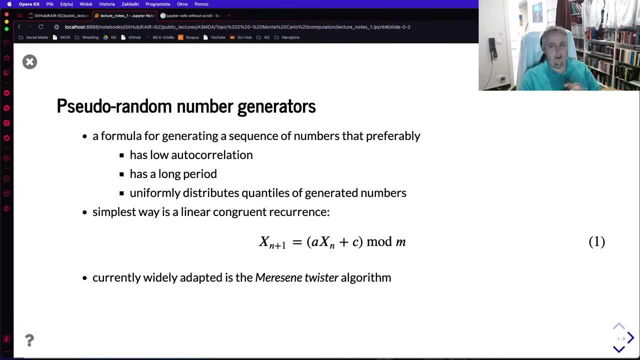 Pseudo random numbers, on the other hand, are software solutions allowing for computation, And generally practicality of hardware random number generators is limited. That is why the most popular option is a pseudo random number generator, And pseudo random number generator is generally a mathematical formula that generates a sequence of numbers which should have low autocorrelation. 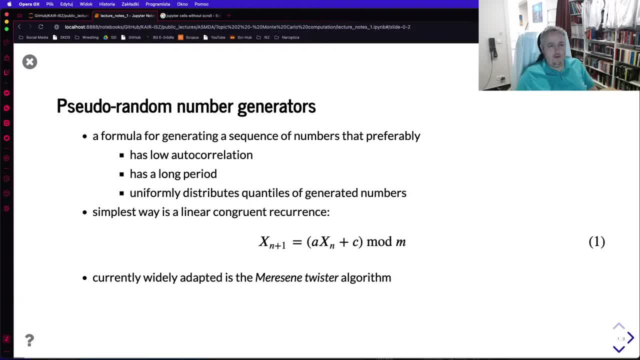 have a long period and should distribute the quantiles of generated numbers uniformly. So generally get uniformly sampled numbers. And the simplest way to generate random numbers is so-called linear recurrence, Which uses the non-linear operation which generates you the randomized integers, Because, starting with numbers, you multiply axn plus c, so you have two parameters, a and c. 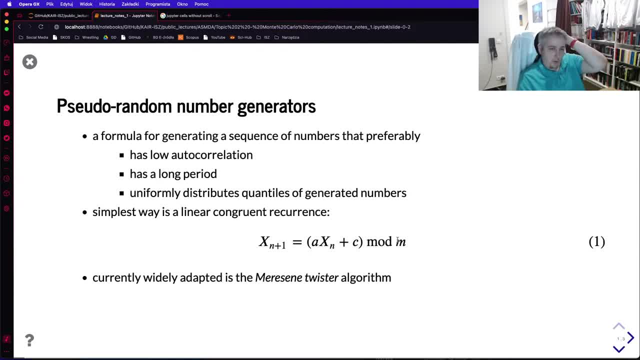 You have a starting number, xn, and you have the m, which is the integer you compute modulo of. If you choose the parameters a plus c correctly, or l with m, your sequence will behave properly. Of course, this is a very basic algorithm which is not really used now. 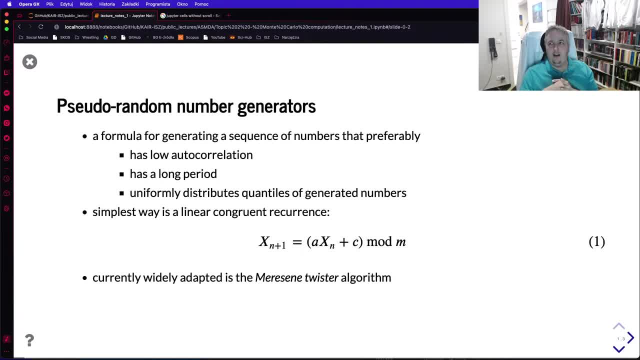 because it was very simple to generate, get information about initial seed from that estimating its parameters. So generally remove the randomness from it. Currently the widely adapted algorithm is the Marison-Twister algorithm, which is being updated sometimes. There is an interesting article on Wikipedia on that. 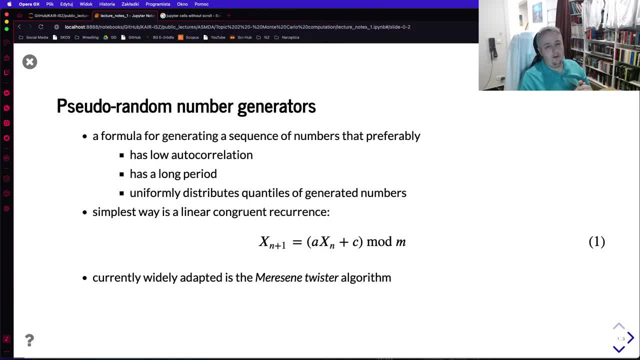 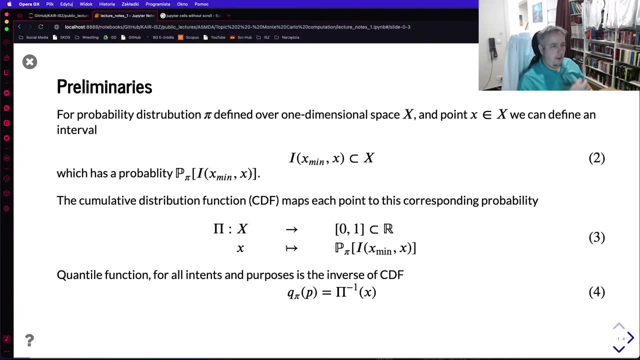 If you are interested, you can read it. It's implemented in Python and in multiple other places. It's a very complicated method to generate random numbers with low autocorrelation, So let's start with some preliminaries. Let's focus first on the one-dimensional spaces. 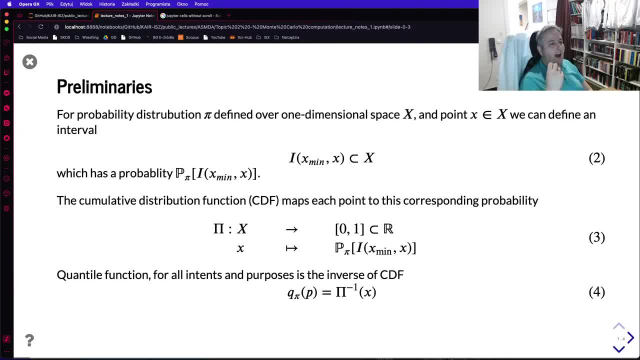 and then we can generalize more naturally: For probability distribution, pi defined over one-dimensional space and one point of x, x belonging to that space. we can define an interval between the minimum possible value of x and this value of x. This is an interval of all x's less than x. 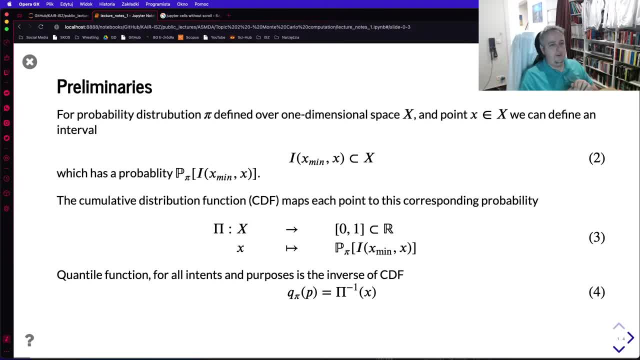 And the probability of x belonging to that set is generally defined as the probability of that set. So, having the probability distribution function, we can then compute the probability of x belonging to a set. Remember, in case especially of continuous probability distribution functions, it is not possible to 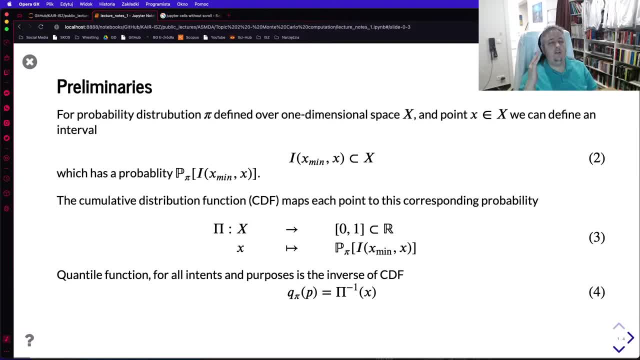 In other words, the probability of x having a single value is zero. However, we can discuss interval probabilities. The cumulative distribution function, which you already should know, is a function that maps each point to this corresponding probability. So for each x, it gives you the probability of a random variable belonging to the interval between x minimal and x. 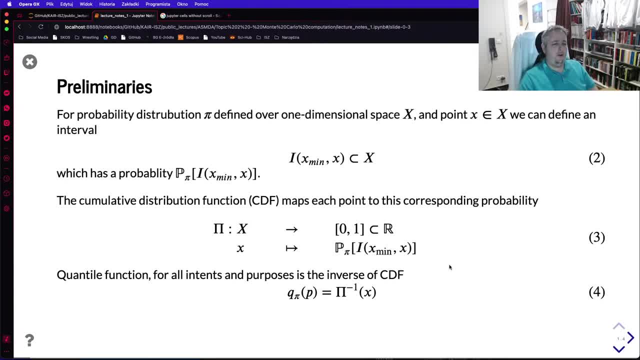 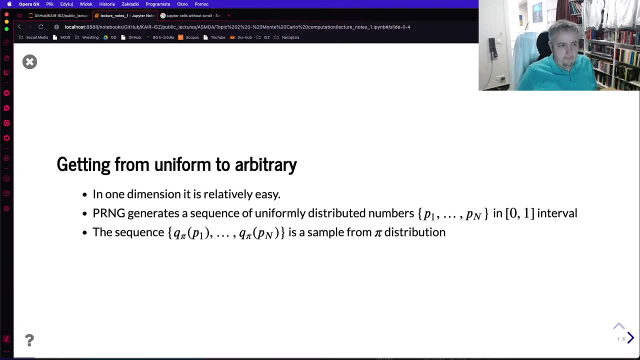 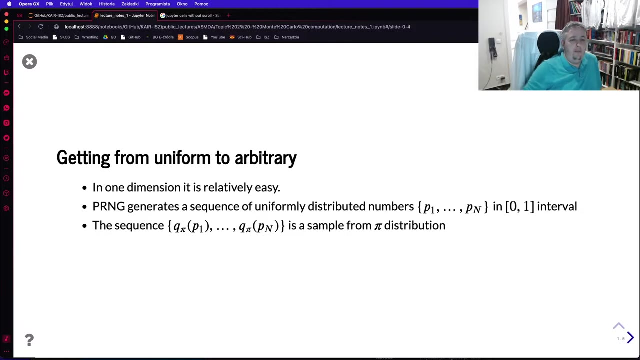 And there is also a function called quantile function which is generally, for all the purposes that can be used, an inverse of cumulative distribution function. So generally Simple parameters. Generally, if we have uniform redistributive functions, then in one-dimensional dimension. 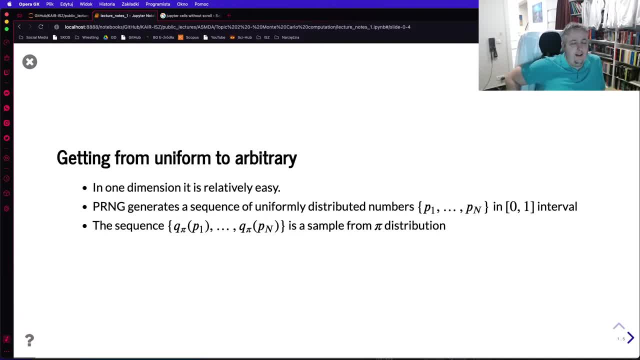 it is very easy to generate samples from such one-dimensional distributions. Why? Because we can easily generate a sequence of uniform distributed numbers from 0, 1 interval using some kind of pseudo-random number generator, And then we can get a sequence of values of the quantile function using the computed values. 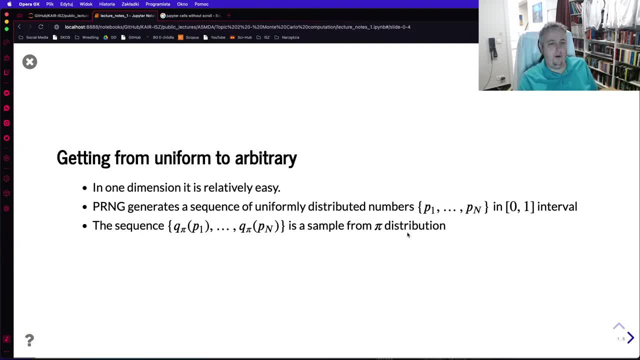 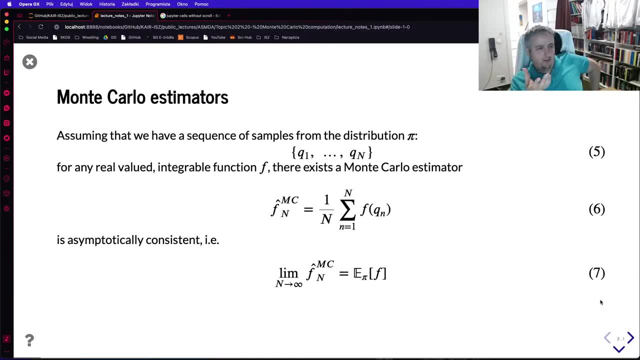 Those values will be a sample from the pi distribution, Assuming that we have a sequence of samples from the distribution pi. this sequence, In other words, if we have a sequence of samples from the distribution pi, then for any real-valued integrable function, x. 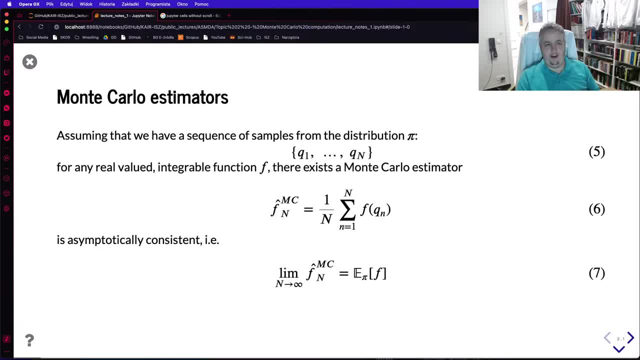 for any integrable function f, there exists a so-called Monte Carlo estimator And this Monte Carlo estimator is an average of values of that function in these points. So if we have samples from the distribution pi, then this estimator is asymptotically consistent. 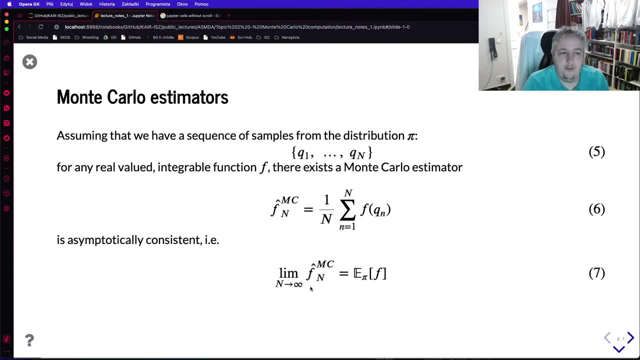 This means that as long as number of samples grows to infinity, the value of this average is equal to the expected value of function f using samples from the distribution pi. Or in other words, a push forward of function f through a distribution pi. So in other words: 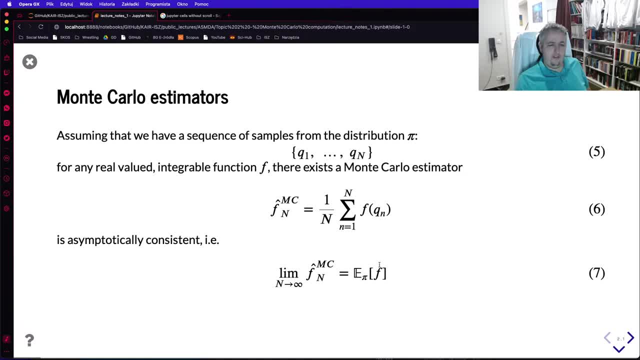 if we want to know what is the expected value of certain function f, of probability distribution pi, of the random variable pi, then this expected value is asymptotically equal to the average of those function values, if there are samples from the distribution pi. So, moreover, 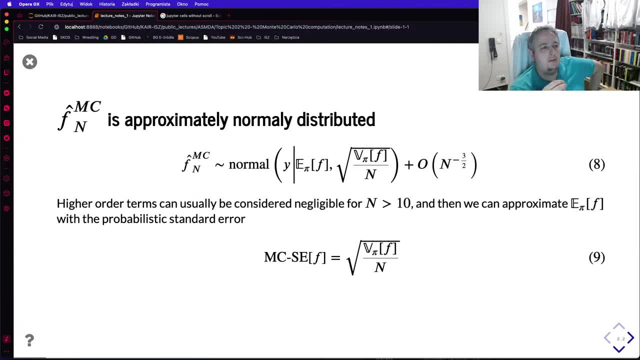 Monte Carlo estimator is approximately normally distributed. That means that its distribution is normal, with difference of order n to up to minus one and a half. So in practice higher order terms can be considered negligible, or n greater than ten, And then we can approximate the expectation. 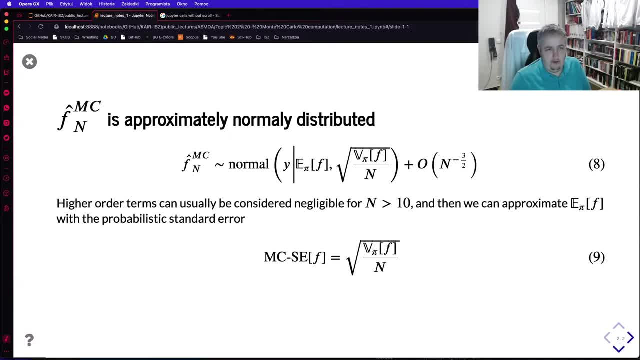 with a probabilistic standard error. So generally if we have samples from the distribution, we get an estimator that says that its expected value of an f is equal to the average of samples and the standard error is given by the variance of the sample divided by n. 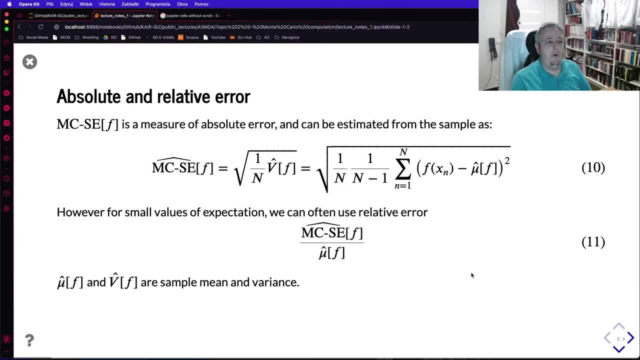 So this value is called Monte Carlo standard error and can be estimated from the sample as an average, using average of f. This is the sample mean, this is the sample variance. So differences of values, like the standard error estimator, from the expected value of the differences between values and sample mean. 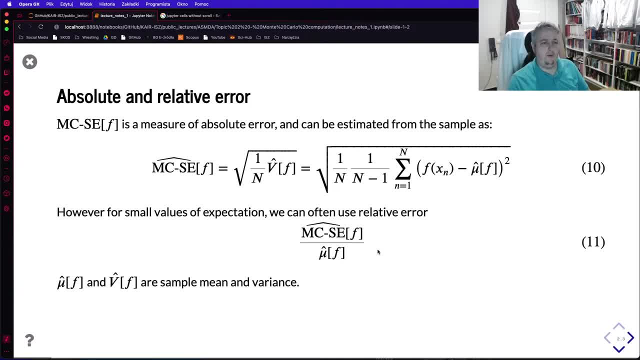 And in case of absolute values of expectation, this is a typical value to use. However, for small values of mean, generally for situations where the expected value is small, we often use the relative error. so the division between Monte Carlo standard error divided by the sample mean. 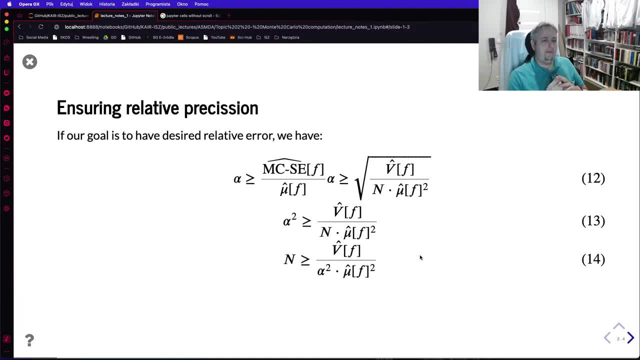 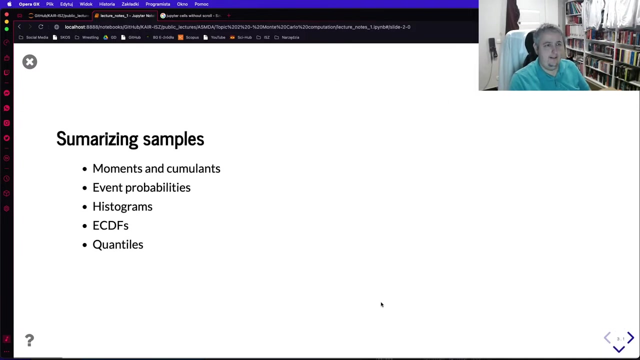 And if our goal is to have a desired relative error, we can compute that our number of samples n should be greater than the sample variance divided by our relative error. squared times squared, This is the third mean value. Generally, from our samples we want to use different kinds of functions. 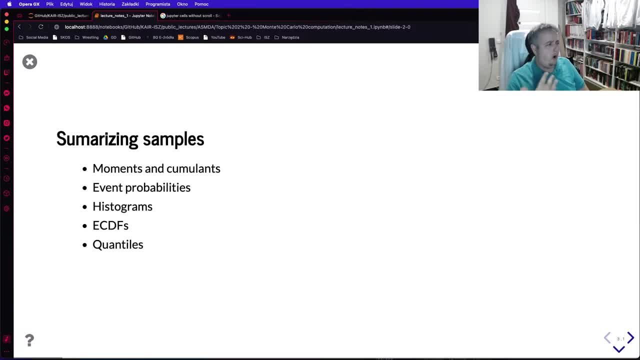 in order to get information about the distribution, or to get or to analyze how the values of function are being distributed. Often we are just interested in identity functions, so just f of x equal to x, But in some cases we might be interested. 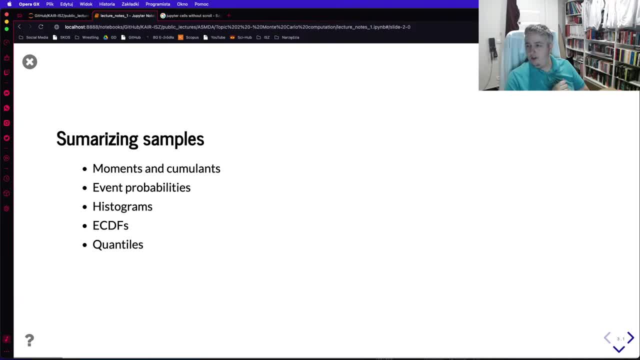 in more complicated functions, For example, if we want to get the values of. I see that in the chat that you have some problems with slides. Unfortunately, I cannot see that. something else is going wrong. I am transmitting in full HD, so the matter of fact is. 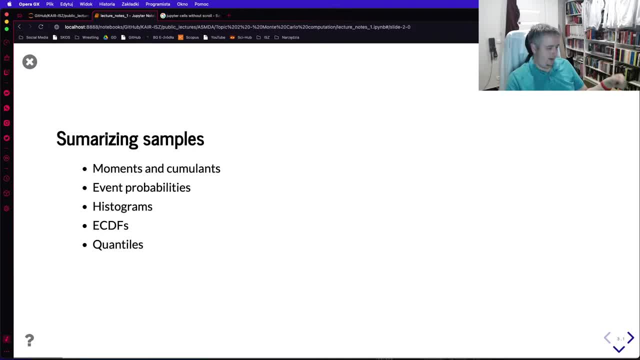 how Internet behaves with that. If maybe you can adjust the quality and it doesn't help, then maybe I'll just resubmit it, because I'm also recording the presentation. So hopefully it won't be an issue Either way. having that. 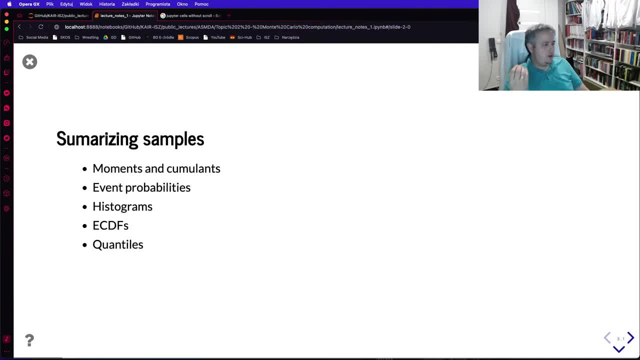 if we have samples of that function which one might be interested. for example, if we want to estimate, use our model to estimate probability or something like that, so we get the function of some kind of transformation of variables, we might want to compute certain values. 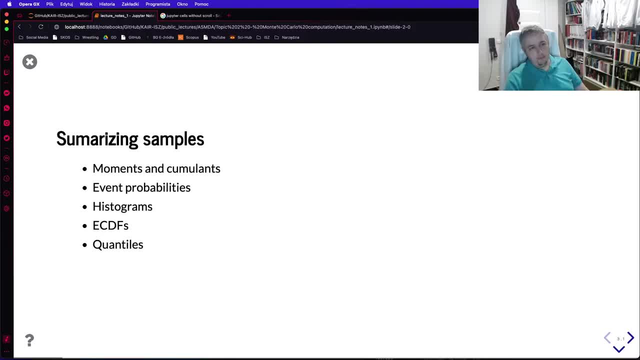 from those samples, like moments and cumulants, probabilities of certain events, histograms, empirical cumulative distribution, functions or quantiles. In a sense, moments are the most typical values of summarization of distribution. Of course, the most known are mean variance. 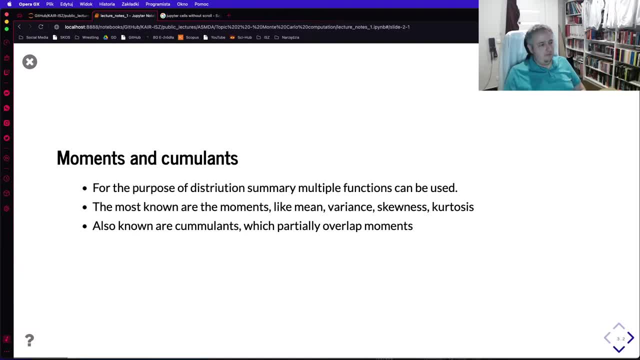 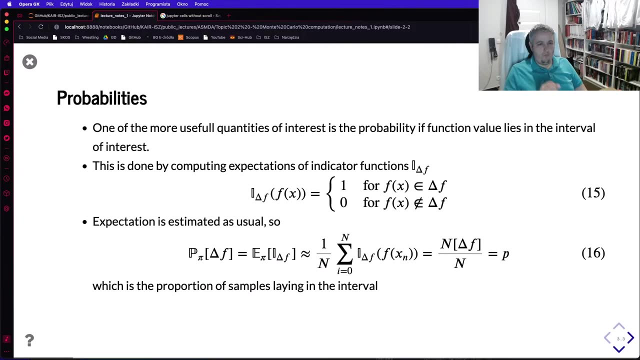 skewness courtesies, so those typically used in classical statistics to characterize a distribution shape. There's also cumulant functions which are very similar to moments with slight differences, which might be used in specialized applications. In case of probability, this is much more specific case. 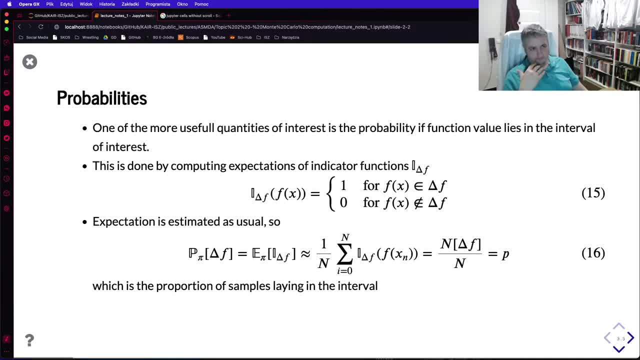 because in generally, in very practical applications, we often want to know what is the probability that the function value will lie in the interval of interest. For example, if our model is predicting is giving the risk of illness, we want to know what is the probability. 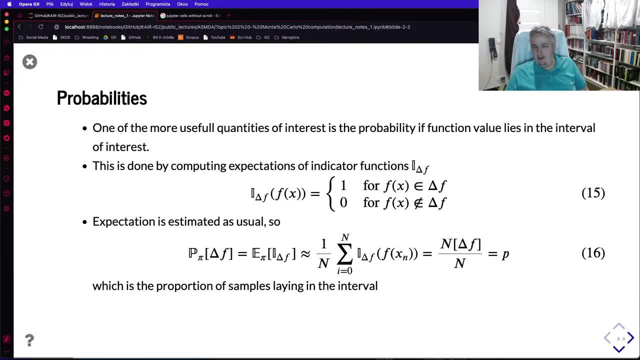 that the risk will be given. What is the probability that the risk will be greater than, let's say, 60%? So, in order to do so, we want to create an indicator function that will assign one for values of f belonging to the interval of interest. 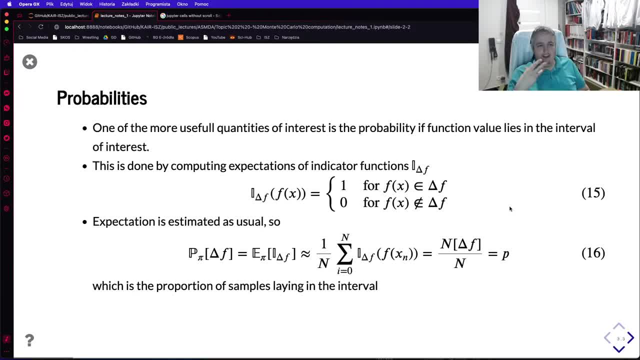 and zero to other samples, And expectation is estimated exactly in the same way. So we use the function. As you remember, there was not very, not too many requirements regarding the function f. It was to be integrable, which this one is. 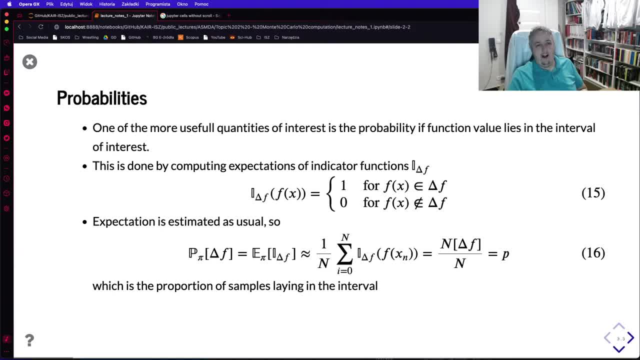 and it needs to be real value, which is also this: one is So the expectation that the probability of the probability that f belongs to the interval delta f is the expectation of the is belonging to, of this integral function, which is then: 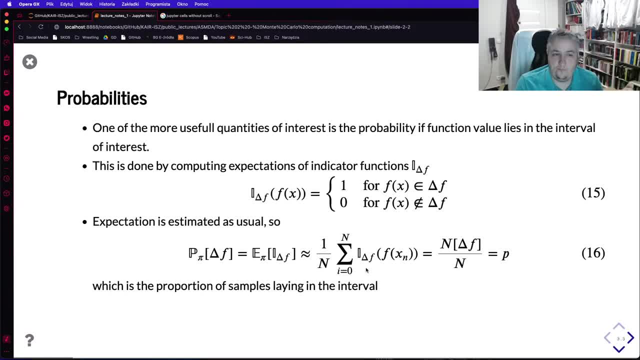 average of values, of the, of sum of values of the indicator function, which generally reduces to the number of samples in the interval divided by the number of samples in total. So that gives us the probability, the probability p. So this is the proportion. 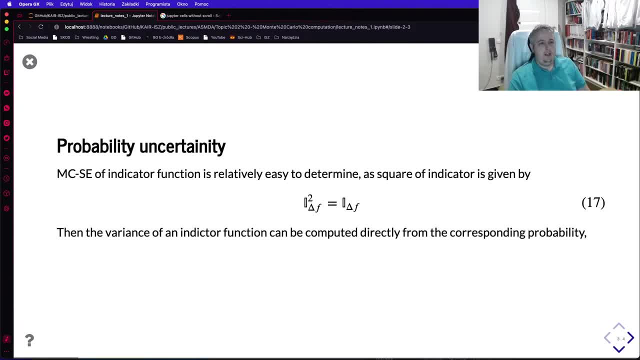 of samples lying inside the interval. In case of the indicator function, it is relatively easy to determine the Monte Carlo standard error because squaring does not happen in this case, because square of integral indicator function is equal to the indicator function And the variance can be computed directly. 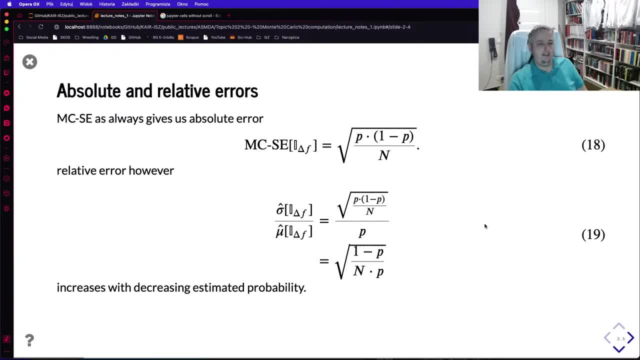 from the corresponding probability. So Monte Carlo standard errors of this, of this estimator, is given by a square root of of p times 1, minus p divided by n. However, what is important, the relative error, is a bit more complicated. 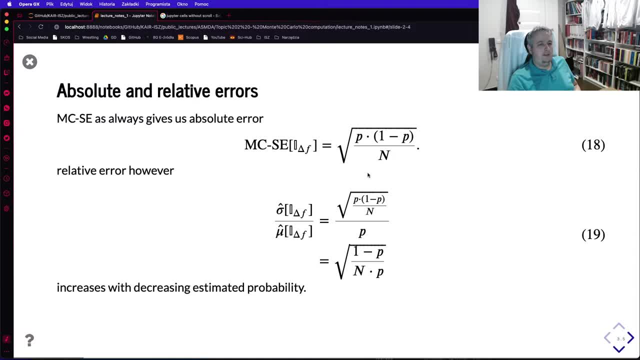 because this is standard. this is standard standard. standard error of beta distribution, However relative standard error. So situation: we are interested especially for small values of p. then it is 1 minus p over n times p. So if p is very small, 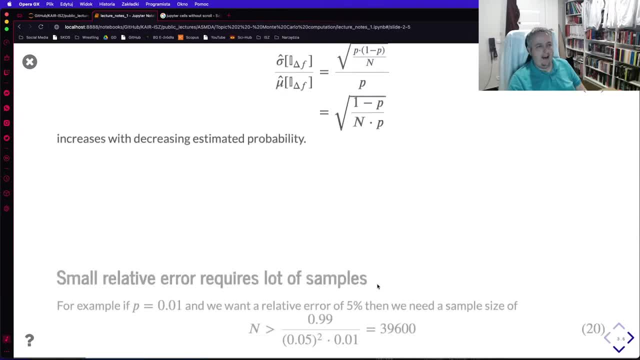 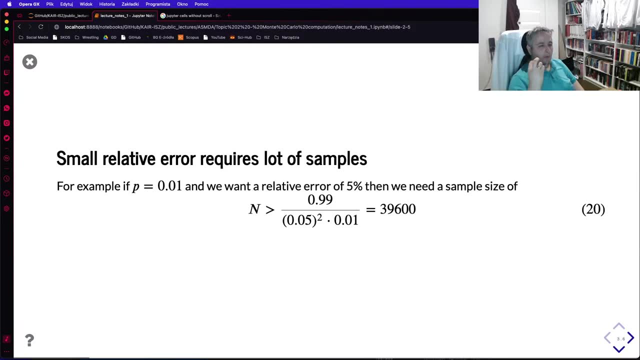 the relative error can be very large depending on the n. So if we want a small relative error for small probabilities, we need a lot of samples. So, for example, if our we want to have a tight estimate on the probability of 1%. 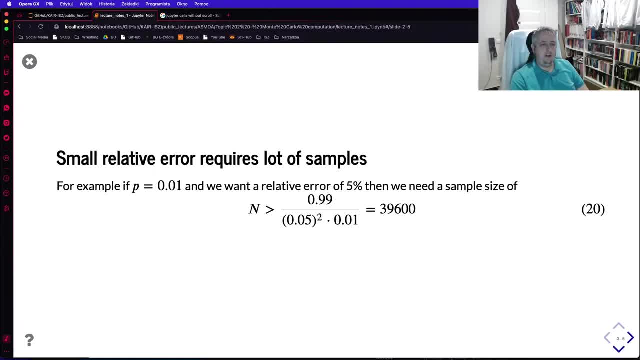 that we are sure that we are not. this probability is not not exceeding exceeding that than more than 5% by its own. So we want to have a very tight estimate of this, this estimate with a tight confidence interval. 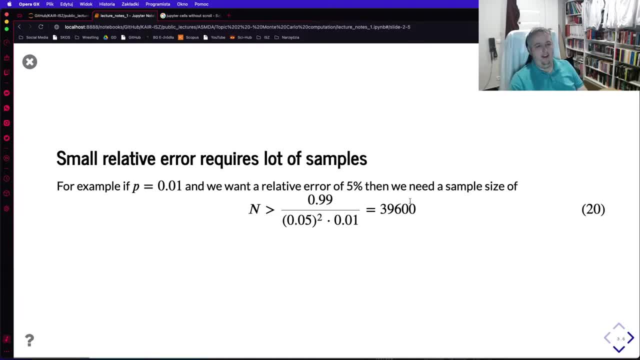 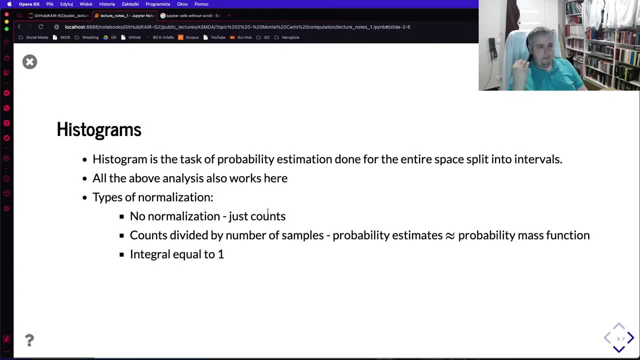 then n? n should be greater than 49,000.. So that's a lot of samples. Different by optimization is the histogram, And histogram you should you know generally from multiple applications as a method of graphic functions. However, 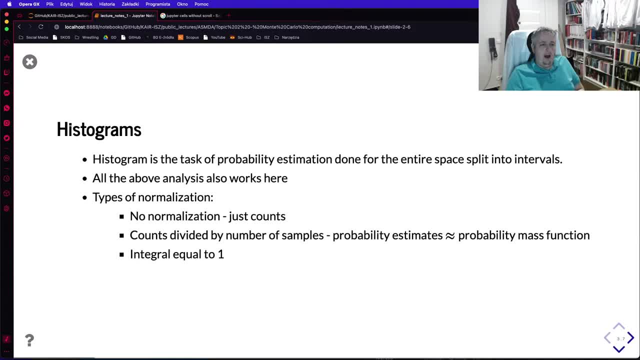 it should be necessary to know that this is. it should be noted that it's it can be considered an estimator of the probability, probability density And generally it is a sum of, it is a joint estimation of probability in collection of intervals. 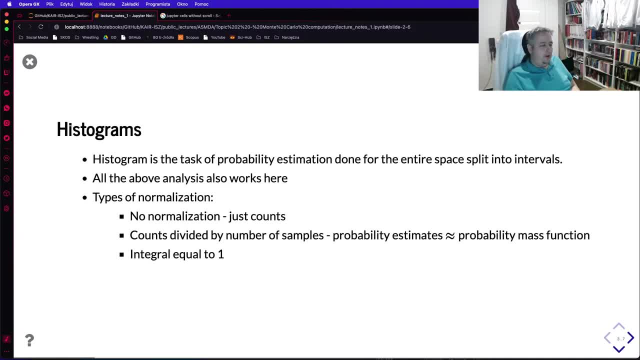 So the entire space we want to estimate the probability of is located here, So we can extend the analysis of interval probability into the interval probability analysis of histogram, because histogram, as an estimate of the density function, also has some standard errors. So 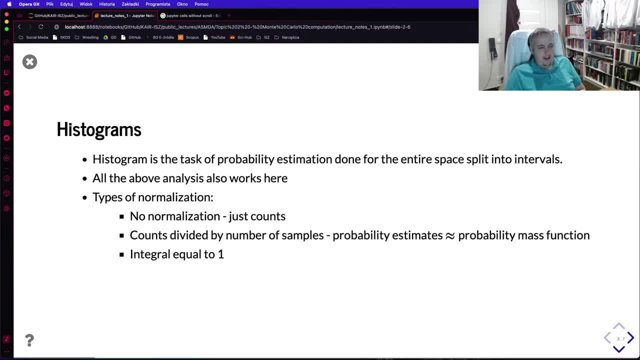 histogram as an analysis of a sample of numbers of data. it's just counts. However, if we want to, from that sample, infer about the distribution, then we need to consider some uncertainty, And this uncertainty comes from the, from the probability function. 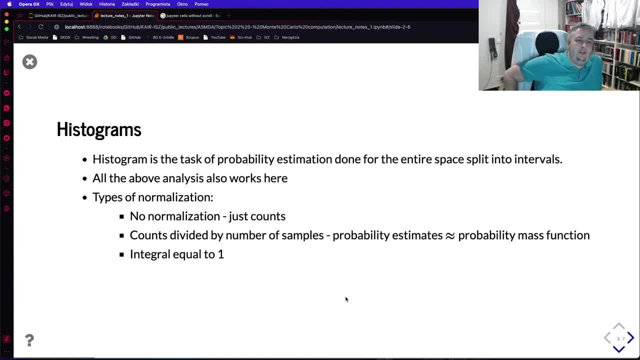 So we also should know that we have multiple times of types of normalization of histograms. So generally either we don't normalize histogram and we just provide counts, or we get number of counts divided by number of samples. So generally we approximate. 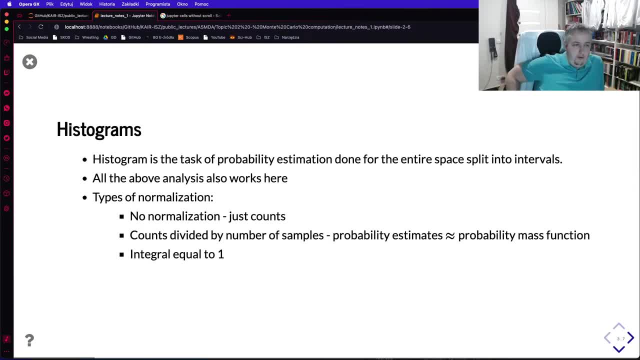 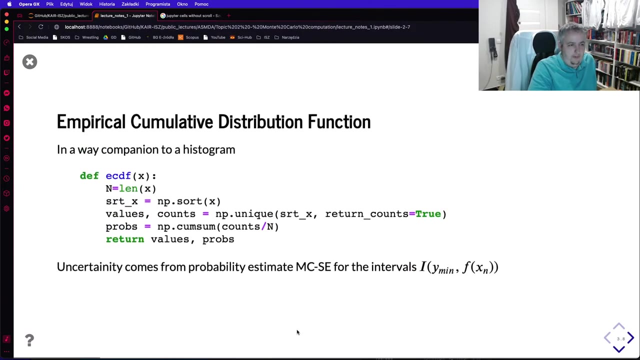 just assigns the values to, probably to each of the intervals, Or you, you normalize the histogram so it will approximate the integral. it approximates the integral representation of continuous distribution. So you just want to have the integral of the entire. 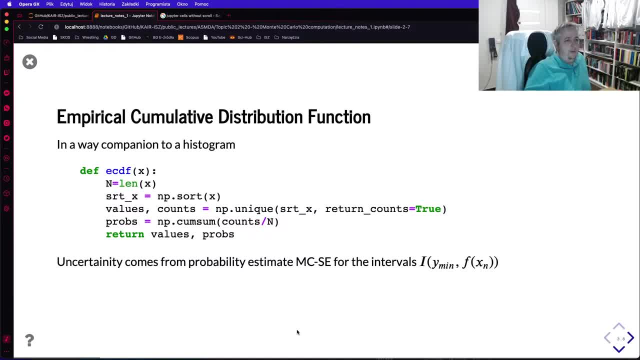 histogram equal to one And different histogram is the empirical cumulative distribution function, which is the function that is the expresses the probability, like the probability of f, of x being greater than minimal possible value, And the uncertainty in this case comes from. 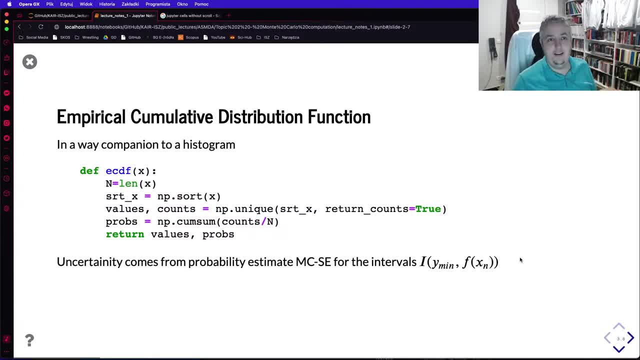 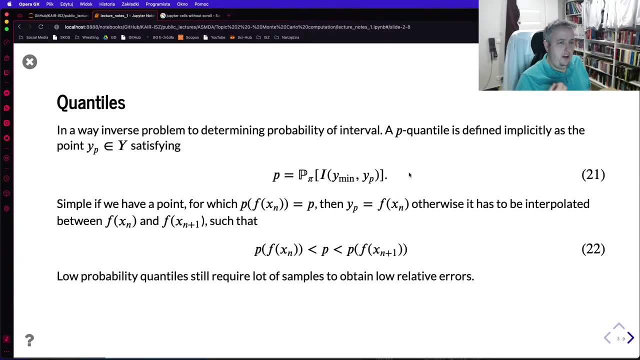 the estimates for the expanding of histogram. each interval has individual uncertainty. In case of ECDF, the uncertainty intervals are growing. Finally, the inverse problem of determining probability of interval is our quantiles, And of course the quantile is defined. 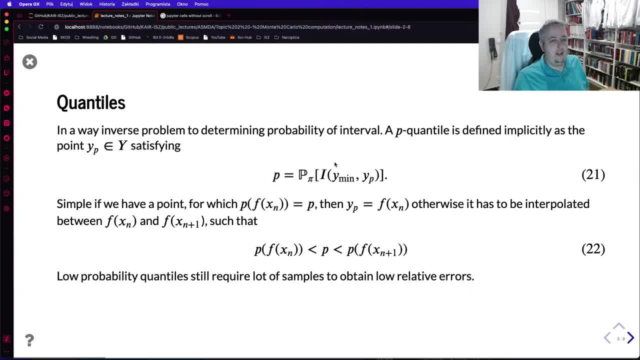 implicitly as the probability of the interval of y belonging to interval between y minimal to y p. So generally finding values that constitute between minimal and p value constitute the p percent of the interval interval. So if we have a data point that corresponds, 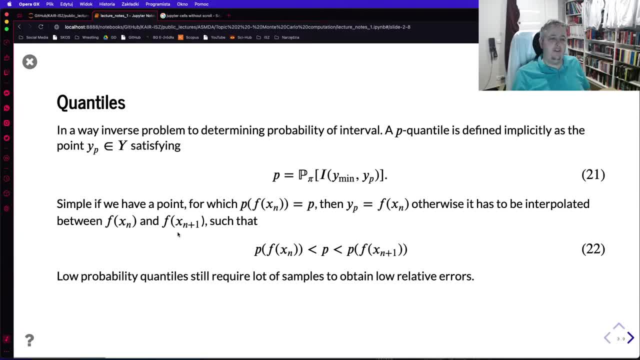 to this situation, then of course we can get the y p equal to the proper value. Otherwise, if we either use linear interpolation or some more ambitious scheme, depending on the goals and of course the low probability quantiles also will, 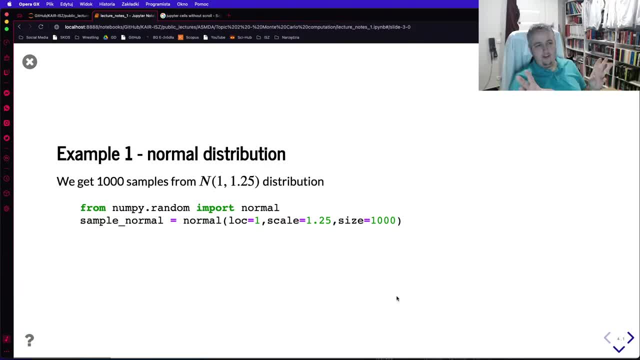 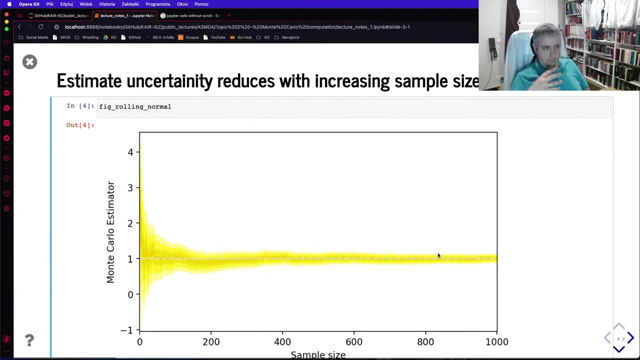 require a lot of samples to obtain low relative errors. Let's see some examples to get. Let's get a closer look at this case. As we generate samples, we can see that our uncertainty regarding the mean, so the expectation of this function. 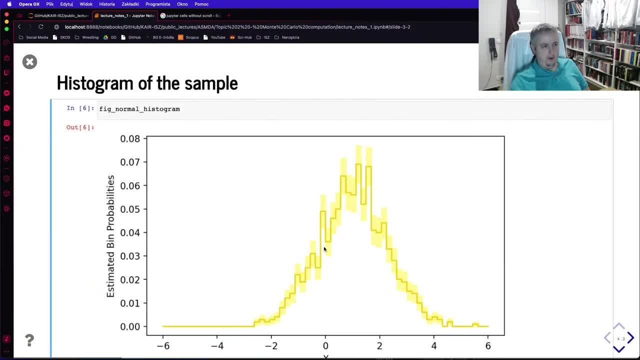 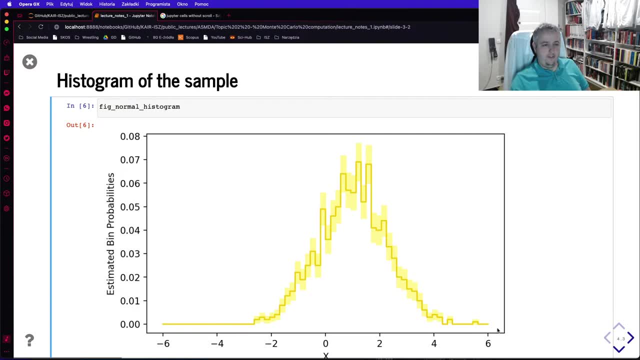 is of course reducing over time. So with increasing samples the uncertainty can be rather significant in some cases because depending on those values, we can get larger values of uncertainty of Monte Carlo standard error, which you can see in this. 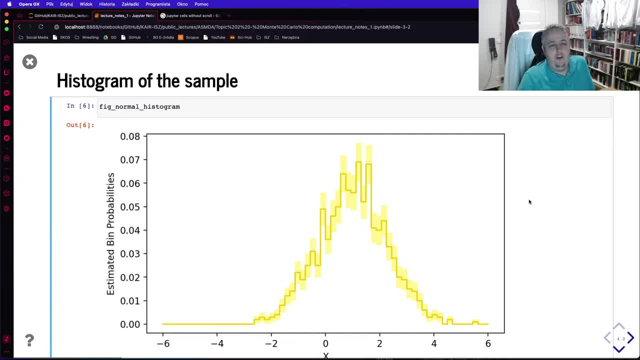 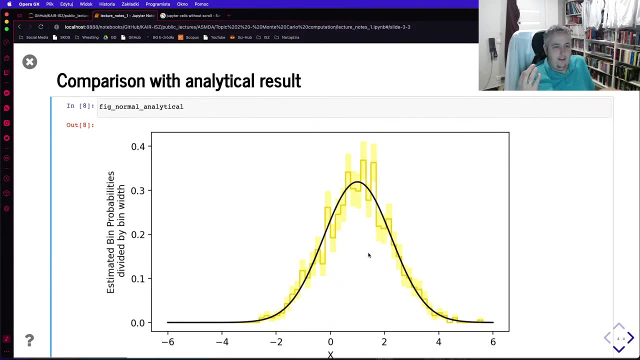 distribution that we have a lot of jumps. so, as you can see, this is a histogram with uncertainty. The uncertainty is more significant in the middle of the interval When you compare it with the analytical result, so with our normal model. 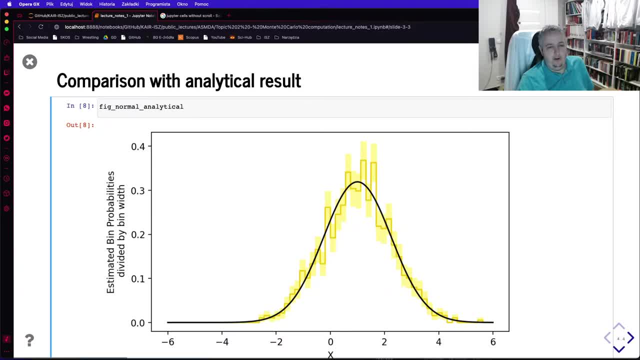 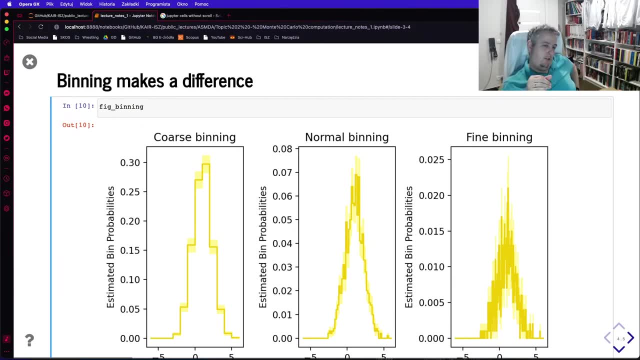 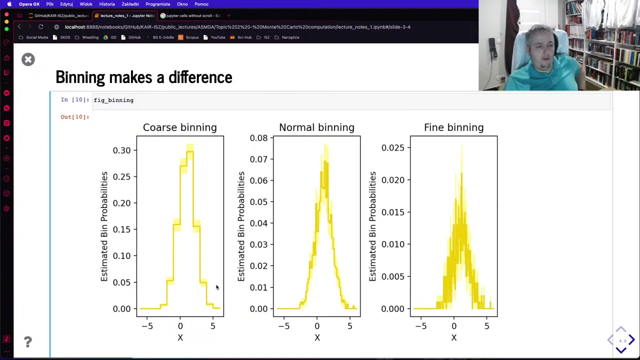 you can see that the uncertainty is much lower than the uncertainty of Monte Carlo standard error. However, what is important is that binning in the histogram creation is taking a lot of effect from the analysis of the figure. So if you have large intervals, 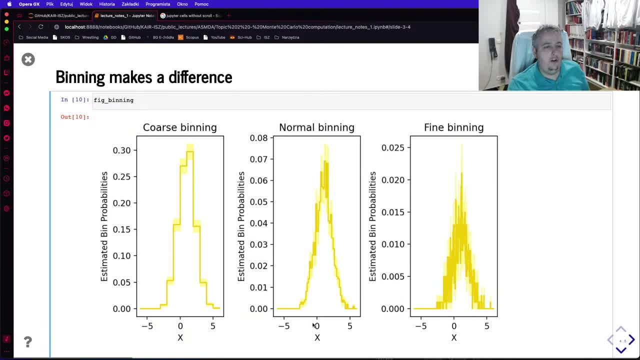 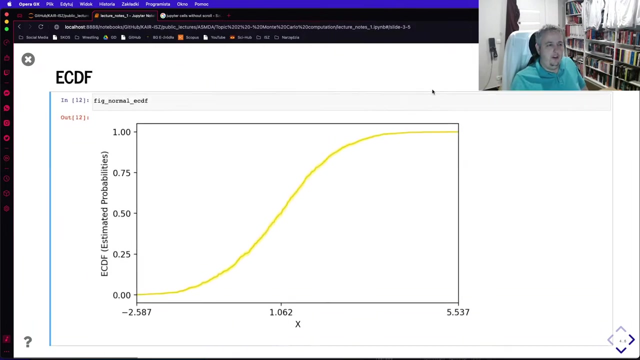 then you lose the shape of distribution. If you go to find you get a lot of noise because you don't know where the noise is coming from. So if you have a lot of noise, then you have a lot of noise in the 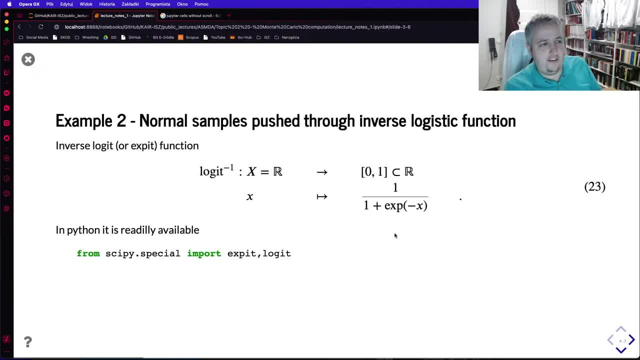 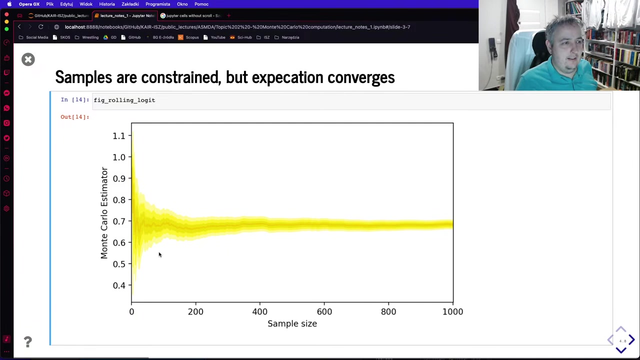 histogram creation. So if you have a lot of noise, then you lose the shape of distribution. So if you have a lot of noise, then you lose the shape of distribution. As you can see, such change doesn't mean much, because 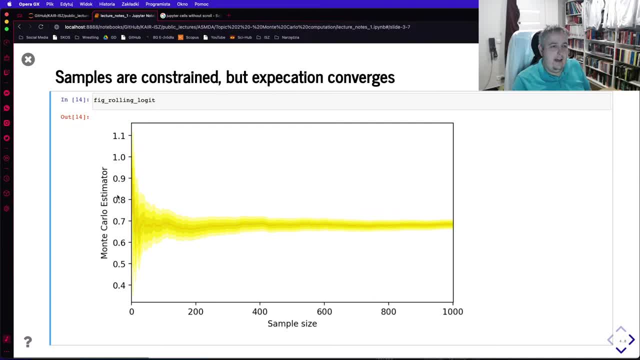 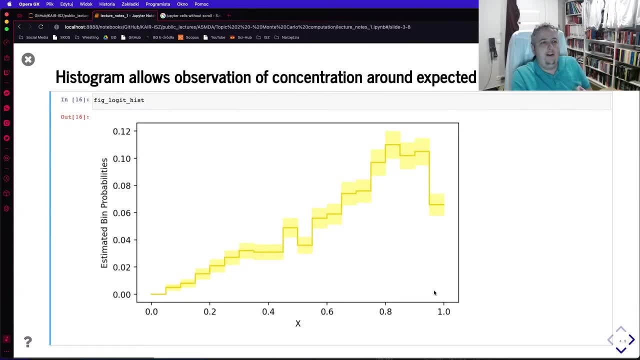 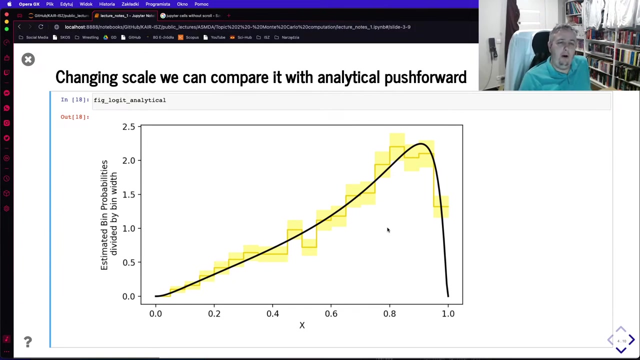 our samples are generally constrained to our interval, but the expectation converges to a concrete value And also we can see that in the case where we have more concentration and the uncertainty is given here, And of course we can compare it with. 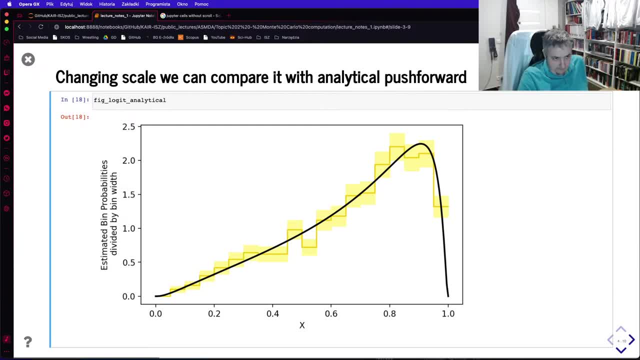 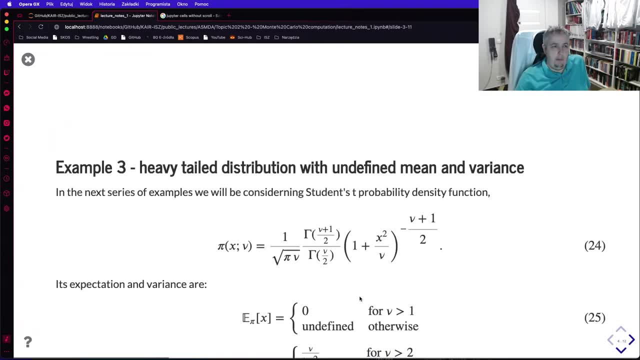 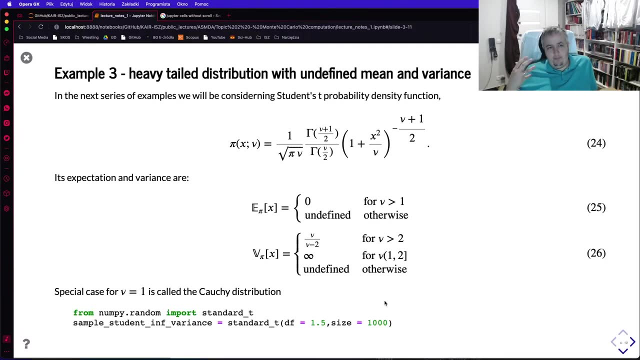 analytical push forward and we get this situation, This histogram, in such a very complex way. Finally, we will get the more complicated distribution, especially complicated in a way that it samples much more difficult, Because we will consider a student t? ers of a specific. 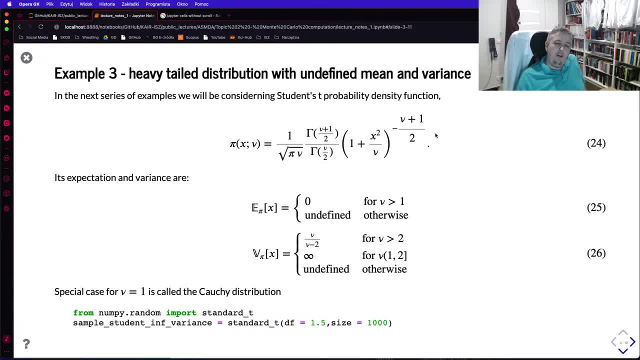 situation, that is, a parameter called the degree of freedom And this parameter is called the number of degrees of freedom. However, this is a historical situation corresponding to the specific situation because, And what is important, the expectation of this distribution, as long as knee is greater than 1, is 0.. 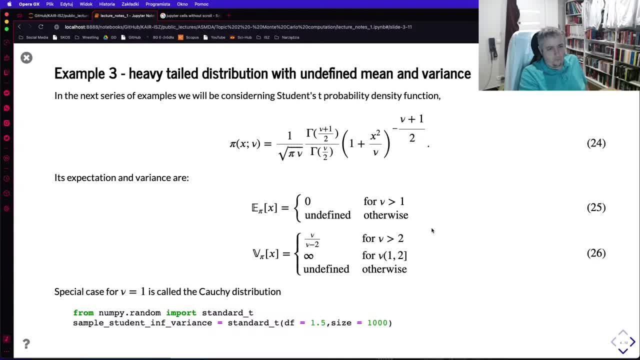 However, for cases of smaller knee, it is undefined. In case of variance for small knee less than 1, we have, of course, with undefined mean, we also have undefined variance. However, even if variance is defined for knee between 1 and 2, the variance is equal to the infinity. 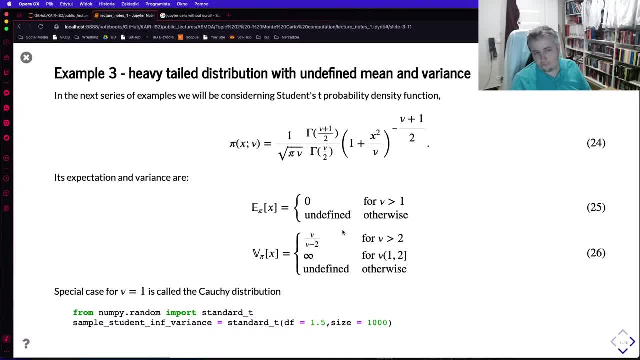 Finally, when knee is greater than 2,, then we can get values of variance And what can be observed here? When knee tends to infinity, our variance tends to 1, and generally student distribution tends to a standard normal distribution with 0 mean and 1 standard deviation. 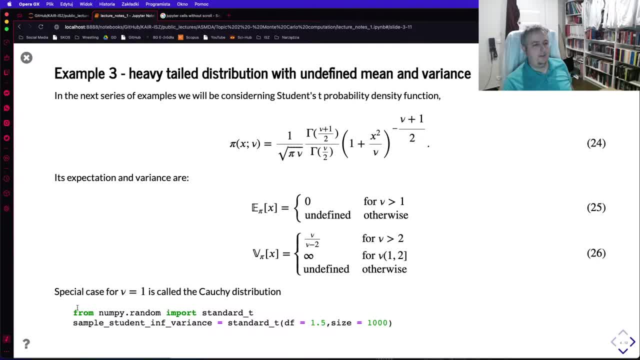 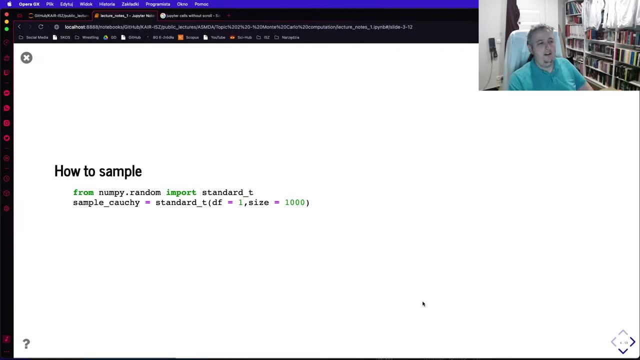 And of course we can use it with the standard libraries. And a special case for 1, which, as you can see, is difficult because it doesn't have neither mean nor variance- is called Cauchy distribution. So in order to sample it, we of course get the values from the standard t function from NumPy. 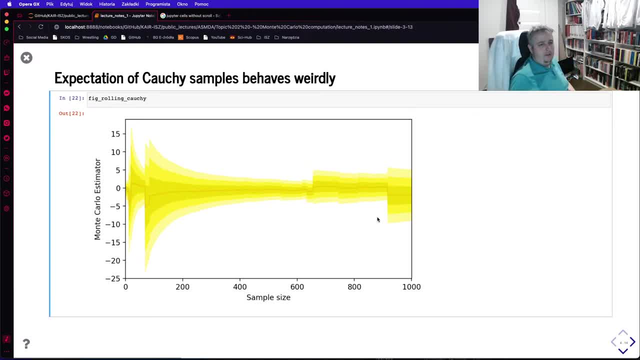 And, as we can see, sample expectation of samples behaves weirdly, Because it first starts normally, then this is the effect of so-called heavy tails. This is a heavy tails distribution. This means that it is rather likely to get large, This sample. the condition for heavy tails given for example, by Taleb, is that the probability of getting two samples greater than x is less than getting one sample greater than 2x. 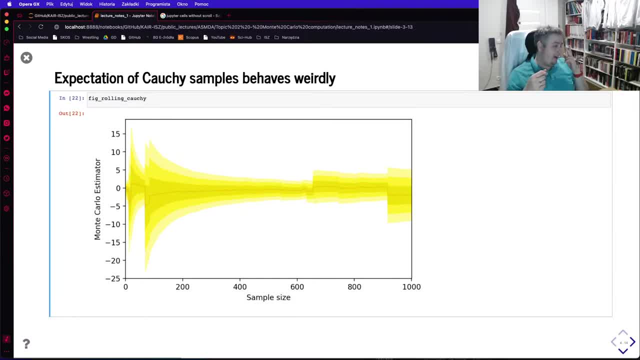 So it's more likely to get one big sample than to get two small samples of the similar magnitude. And heavy tails distributions express a situation that everything can behave normally, but then sometimes, bing, something happens and the event. This is popular in the theory of antifragility or the black swan idea that something can happen and is difficult. 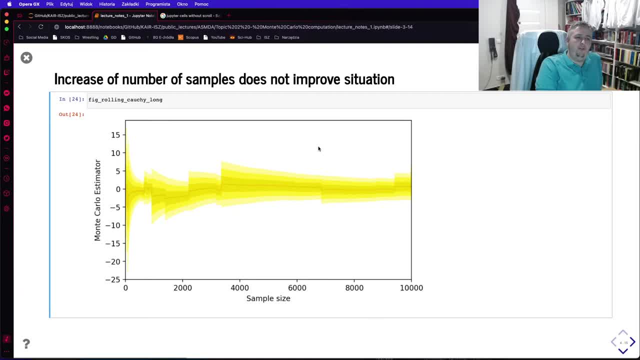 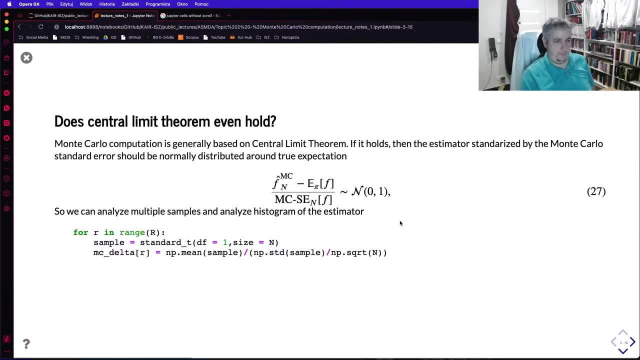 And increasing the number of samples unfortunately does not help because still after some time you get those jumps that Even if there is some drop in an uncertainty, then again it rises significantly And we come back to the problem of: does central limit theorem hold? 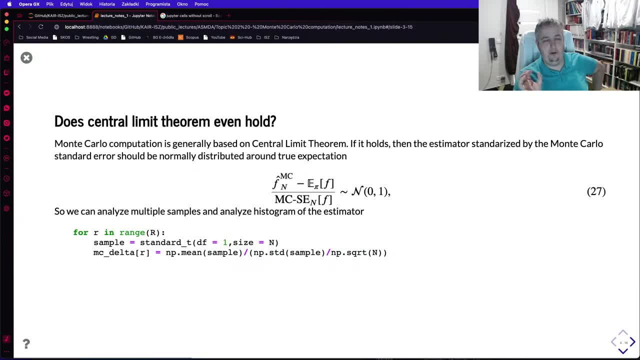 Because Monte Carlo computation is generally based on central limit theorem. Why? Because Monte Carlo estimator is an average of random variables, And average of random variables follows central limit theorem. But in this case we have a problem that this happens if our samples make some kind of sense. 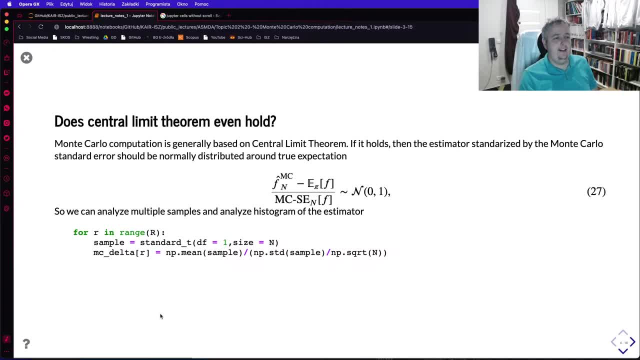 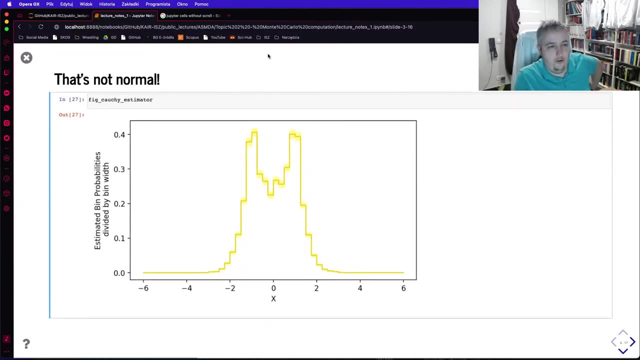 And in this case we have. Let's consider what happens in the case of our standard, In case of histogram, of our estimator And, as you can see, this is obviously not normal, Because you have Two significant spikes here happening regarding the estimator. 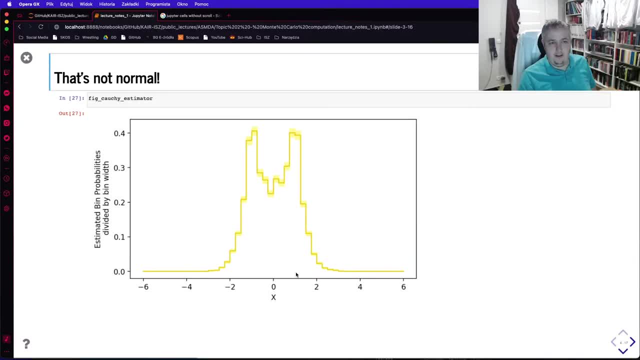 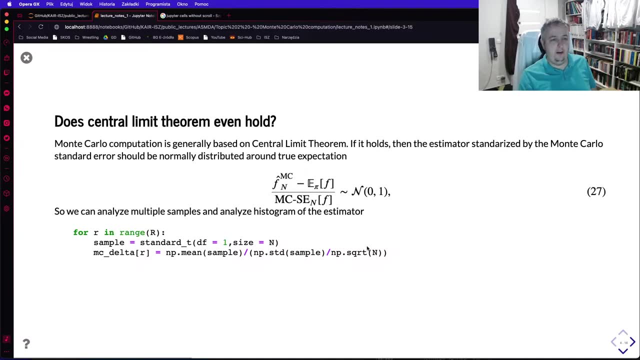 Again, we are considering the, We are considering the difference, The normalized mean divided by the square root of n. So we are generally considering how behaves the difference mean between samples. So the error of this, Because expectation we assume to be zero. 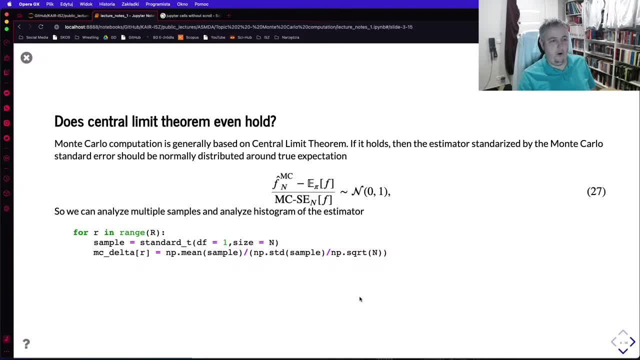 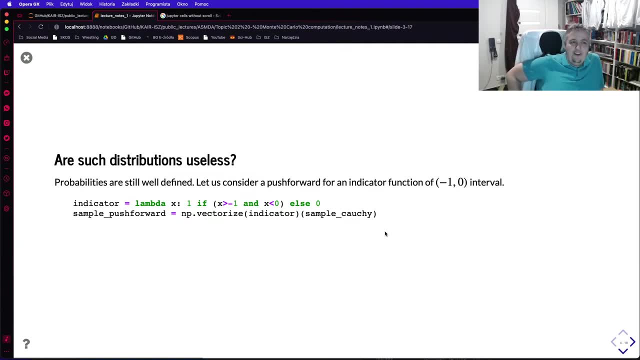 And we compare it to the standard, To our normal distribution. So obviously this is not normal. But are heavy tail distribution in this way useless? No, Because certain probabilities, Certain quantities are still very well defined. Histogram is well defined. 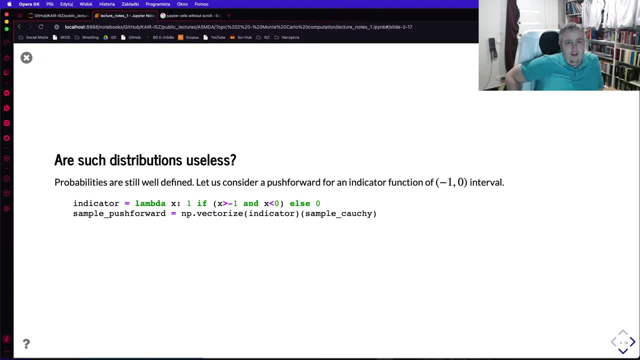 And generally probabilities are well defined. So for example, if we take an indicator function of the interval minus one and zero, We can easily compute the sample, push forward So we can get from our indicator function We can get the values if x belong to the interval of interest. 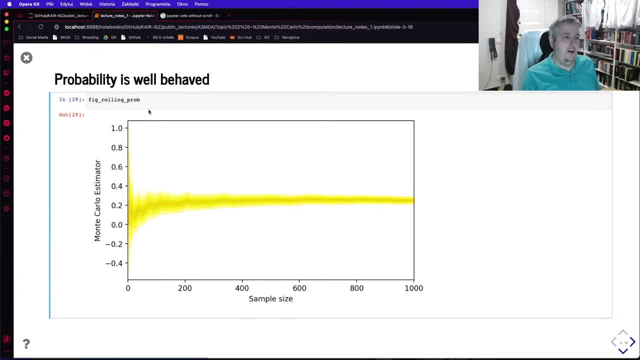 And using such function we can again consider how the probability behaves And in this situation the expectation of probability. So again We analyze the expectation of what is the expected probability of value belonging to the certain interval, Then this situation has no problem. 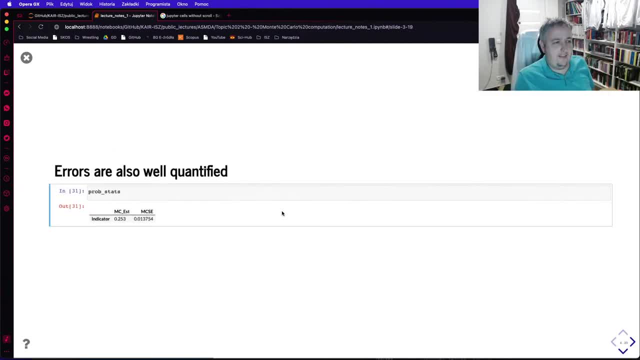 Increasing number of samples reduces the sample size And, as we can see, errors are well quantified. We can get the Monte Carlo estimate given of the indicator as 0.215.. With Monte Carlo standard error of 1. Or of 0.01 with it. 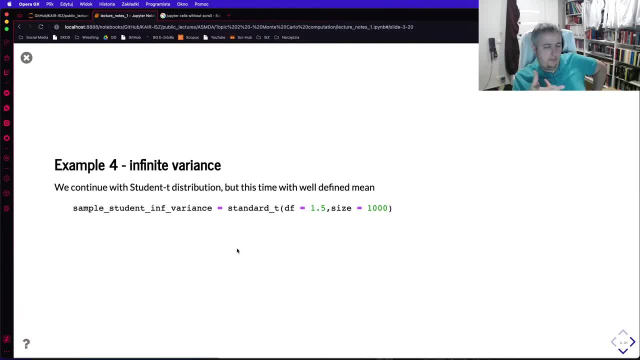 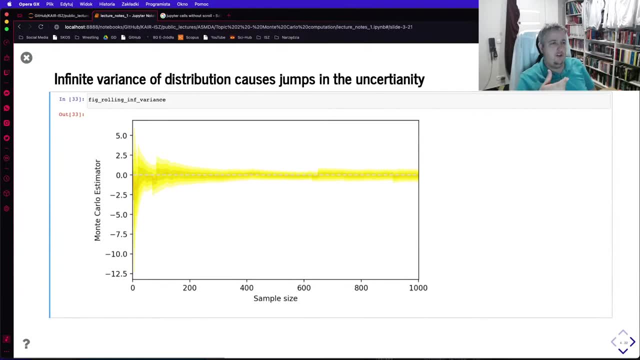 And if we move to the finite and existing mean, but infinite variance? The similar situation can be observed Because we have a convergence to the expected value, But the uncertainty is behaving specifically And again Because we do not have the normality. 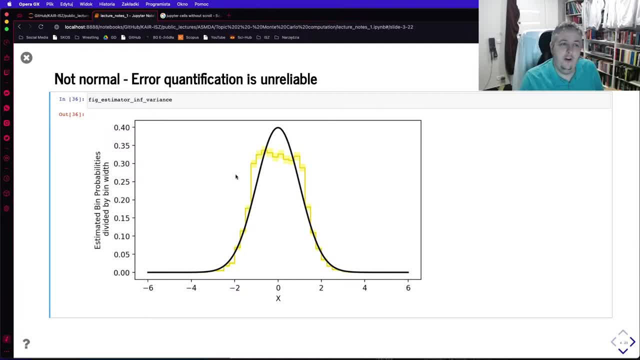 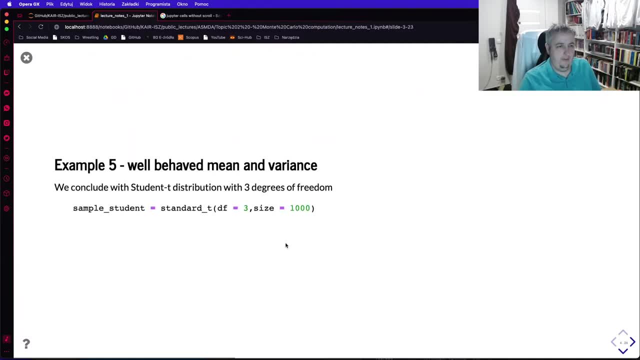 We do not have infinite variance of our samples, Then our error does not follow the normal distribution. Of course probabilities will work, And if we move to the student distribution which has a normal mean and variance, Then there is no problem. 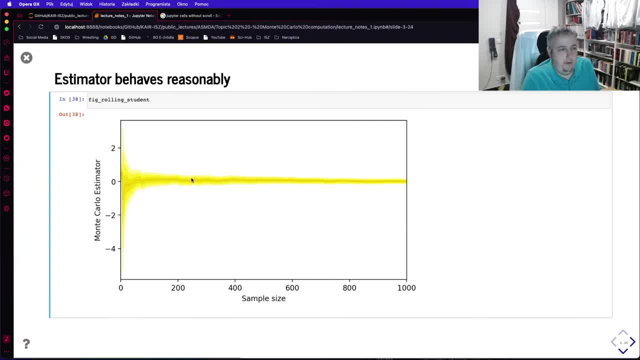 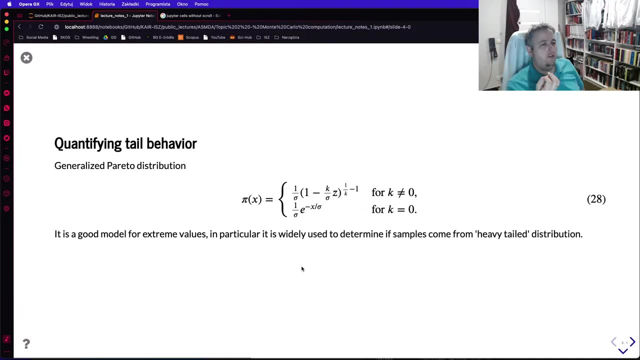 The probability estimate is very reliable And the error is normally distributed. Again, this is a plot of error, Not a histogram, But an error of our predictions, And this gives us the reason to do some analysis, How to verify if our estimators make sense or not. 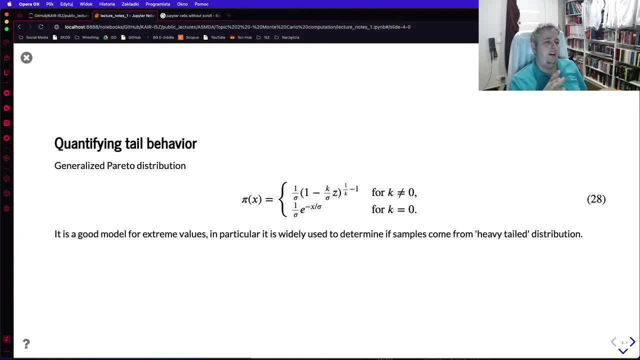 And for this point, Generally We often use a thought called generalized Pareto distribution, And this is a distribution that is used to quantify the tail behavior, Because this is a heavy-tailed distribution. So in case it gives you heaviness of the tails, 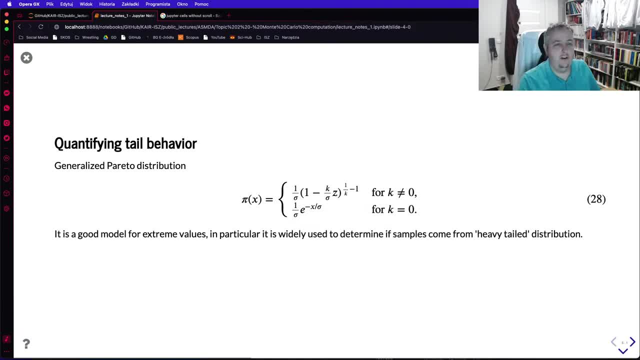 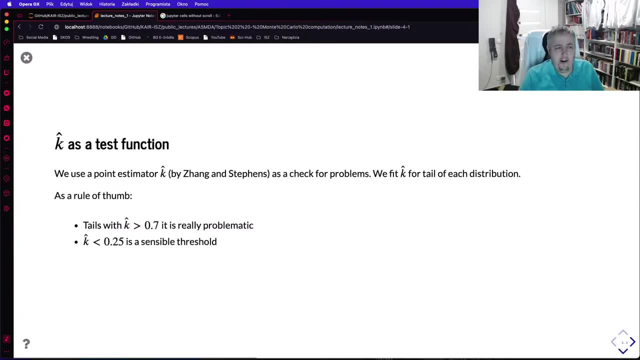 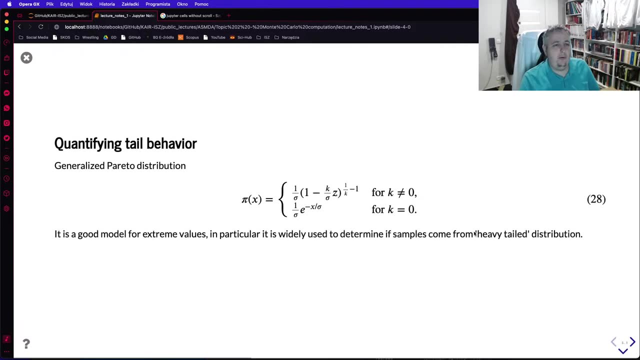 Then your tails get the And then you get an information that okay. There will be problems with variance And generally Problem of estimating parameters of the distribution. This can be formalized in the Bayesian problem, But we don't do it here. 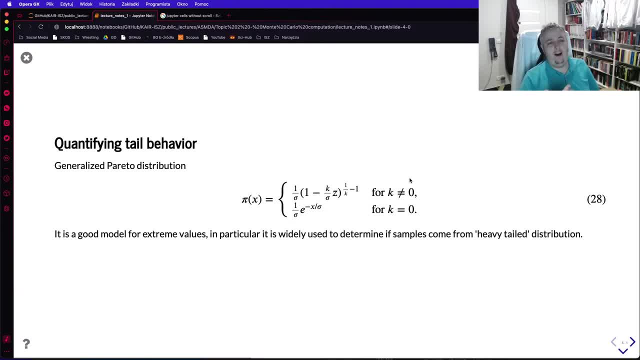 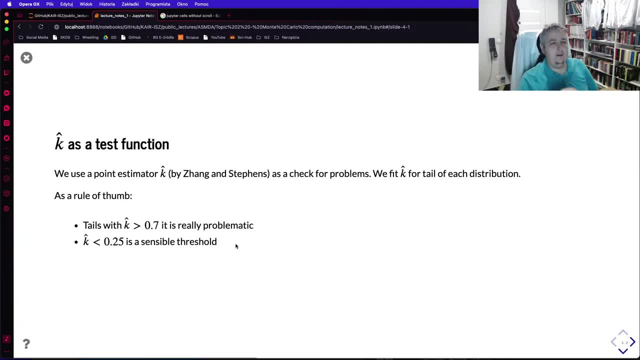 Because we are not really want to use it as a model of our distribution. We want to use it as a test. Is there a? There are reasons to have a, To expect the heavy-tail distribution And we can use the point estimator. 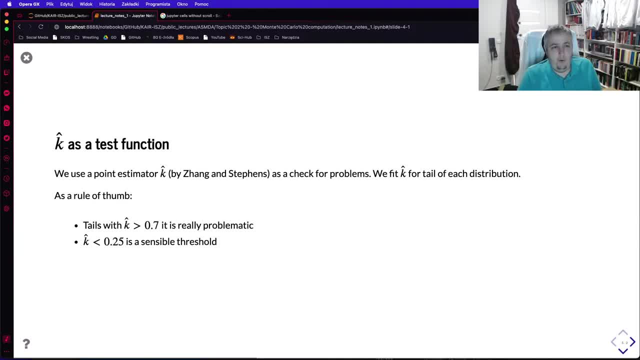 K hat by Zhang and Stevens, Which is An Useful diagnostic for that, And We do it by fitting K for tail of the distribution And generally If K hat is greater than 0.7. There will be problems. 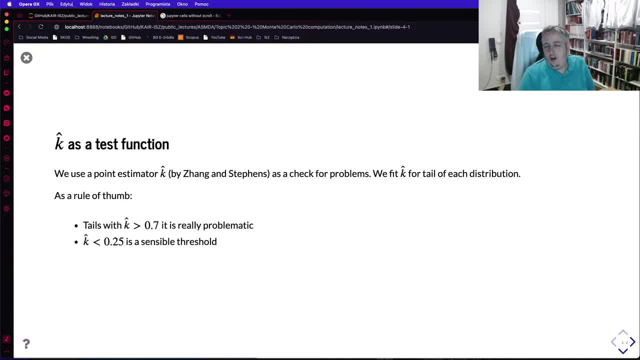 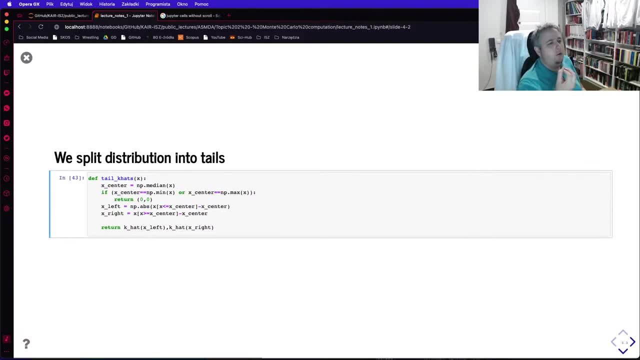 And Generally K hat less than 0.25.. Is a safe situation And it works like this: That you just You need to split the function into Bulk and tails And you do it by getting the samples that are. 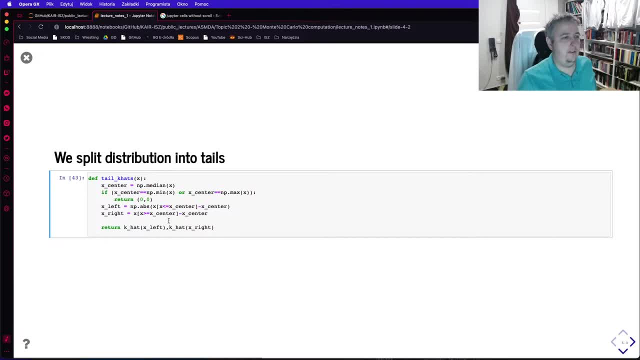 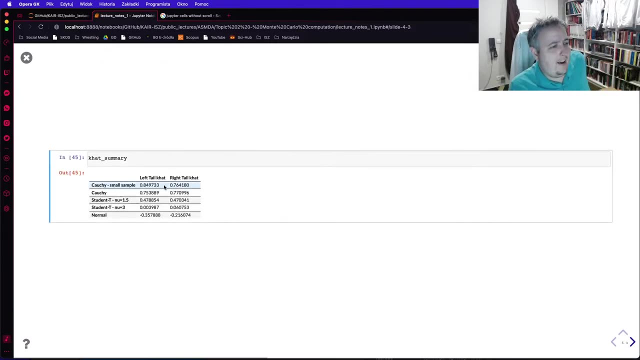 On the left of Of Of median by An appropriate value, So like One million away from the From the median, And you can then use the K hat function to estimate And, in case of Koshi, Distribution, Either. 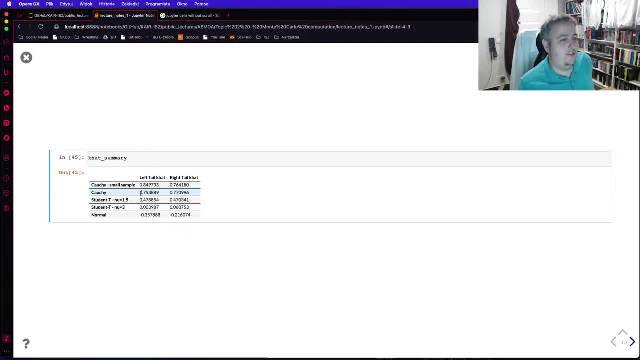 For small Or for large samples, We can see that we have A distribution Significantly Above 0.7.. So In this case It is, It will be, It's a Heavy tail distribution Which it is. 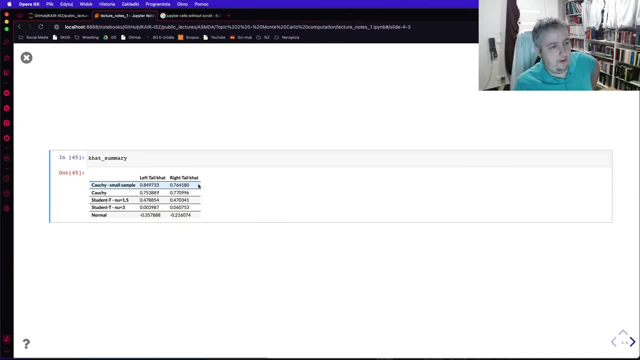 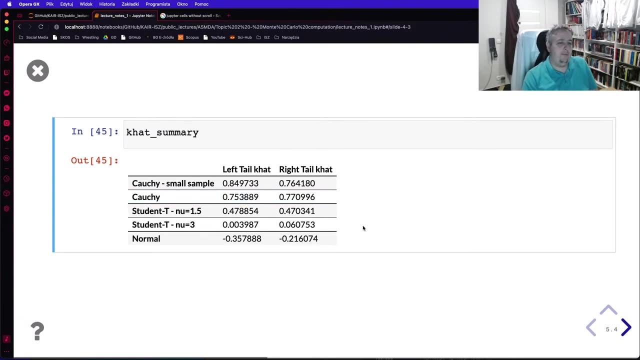 In case of The T student, With Infinite variance. But Finite mean We Have an issue That there is A larger value Of K hat, But We have Larger values Of K hat. 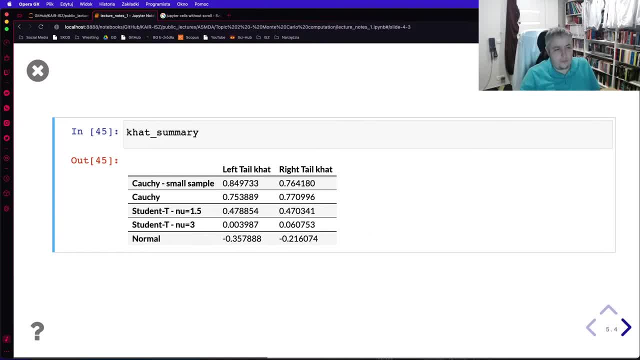 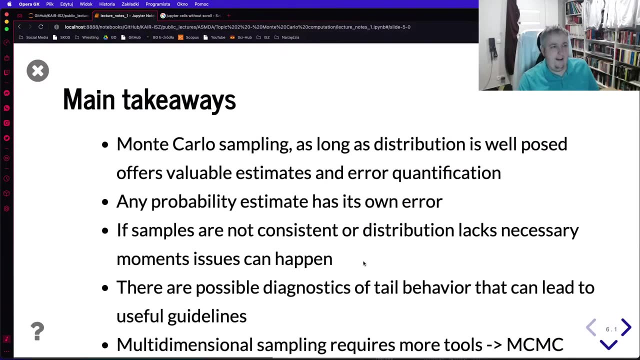 So We can expect There will be Some problems, And In case of Student T, With Three degrees Of Freedom, The K hat Is Very Small, So It's Non-problematic. 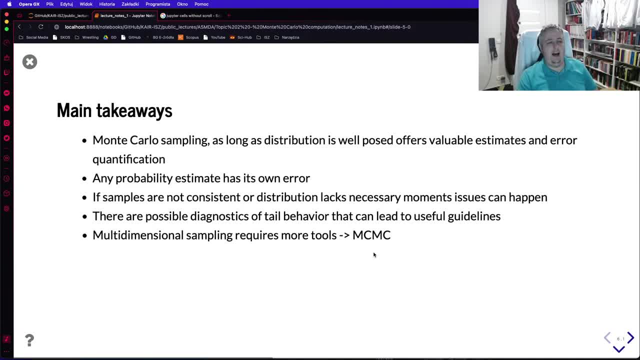 And In case Of Normal Distribution Of Valuable Estimates And Our Quantification Provoke Each Property Estimate Made, Either It's a histogram Or Interval Estimate, Or 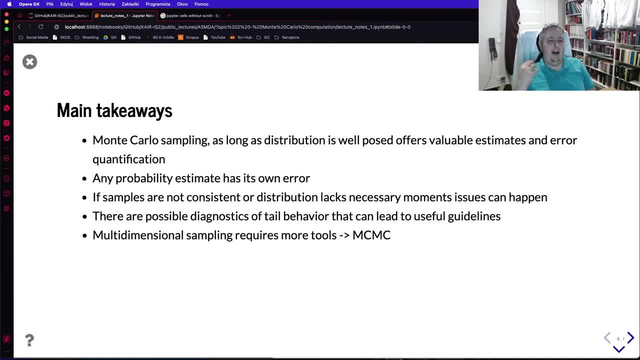 Quantism Has Its Own Error If Samples Are Not Consistent With The, The Issues. And You Can And Using Tile, Tile Diagnostic, You Can Get. 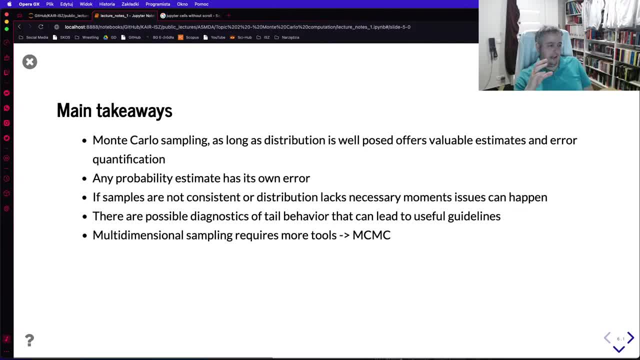 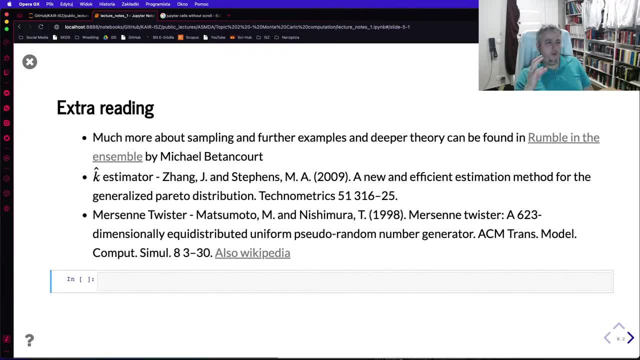 Some Kind Of Information About Your Distribution, What Is Happening? But The Issue Is That Generally, I Strongly Recommend Michael Betancourt's Website, Which 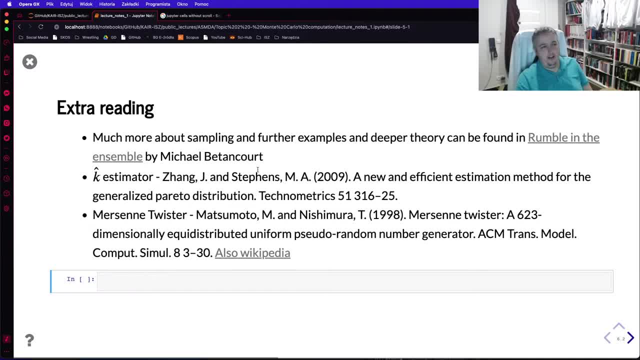 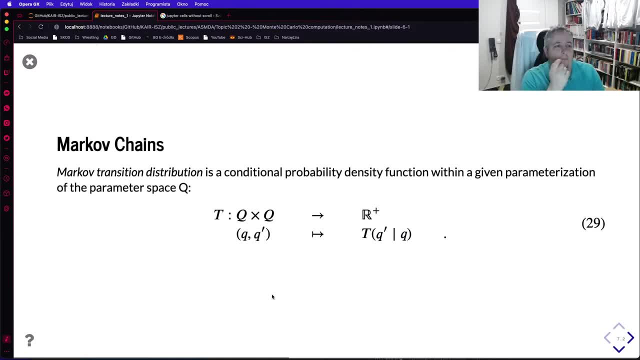 Discusses The Sampling Theory Significantly Well And Some Information About Merson Twister And K Hat Estimator. So Let's Move To The Mark Of. 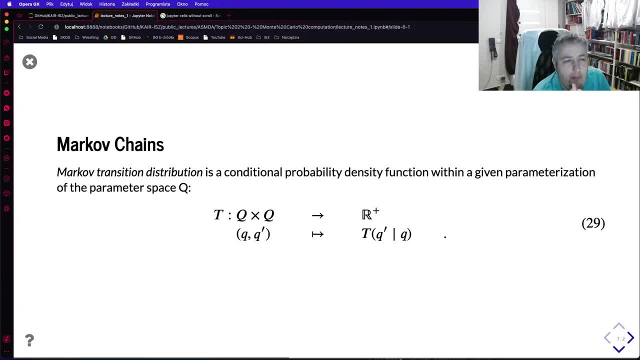 The Probability Of Moving From Point Q To Point Q With A Hat. So It Goes From One Point, So It's For Given Two Points. 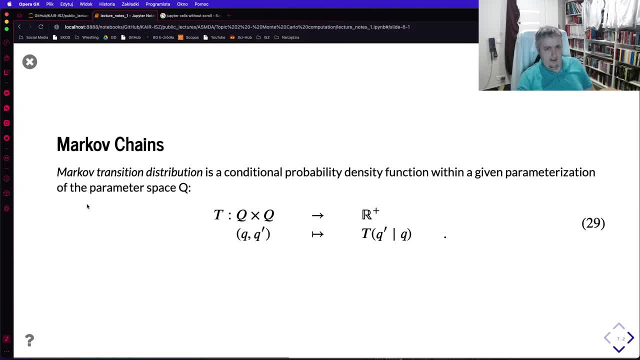 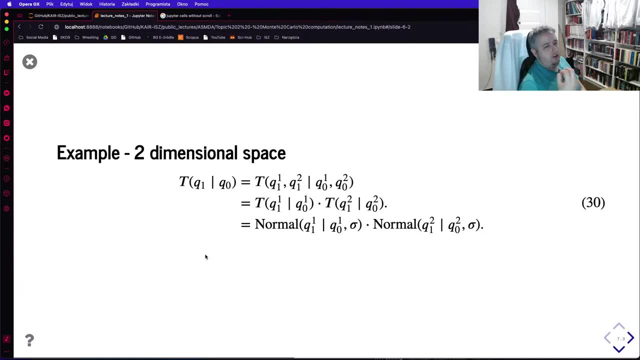 Q And Q. Hat Q Is A Parameter Of Space. For Example, In The Two Dimension Space We Have A Vector, Vector Q One And Q. 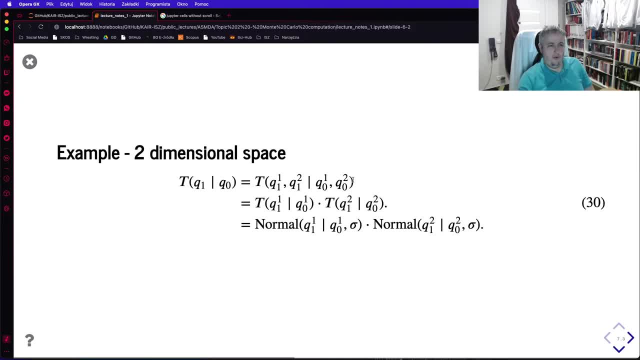 Zero And Assuming Certain Independence, We Can Get. So If The Movement In Both Variables Is Independent, Then Of Course Those Will Be Two Independent Situations. 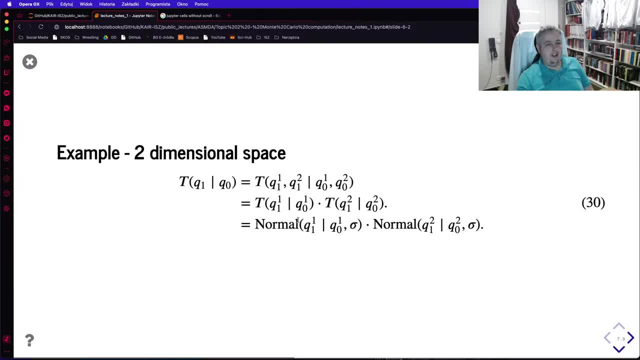 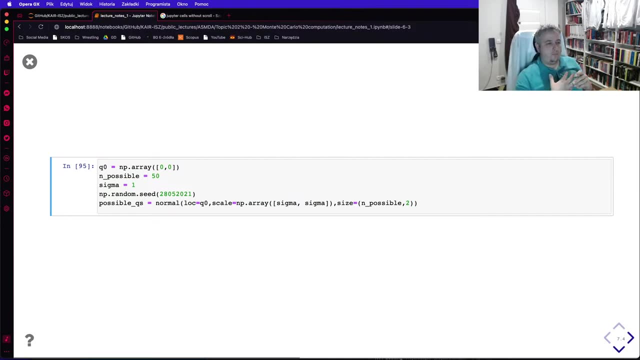 And The Probability Of One Will Be A Normal Distribution Conditional. So Let's Start With The Point Zero, Zero. Let's Get The Possible Movement, Assuming. 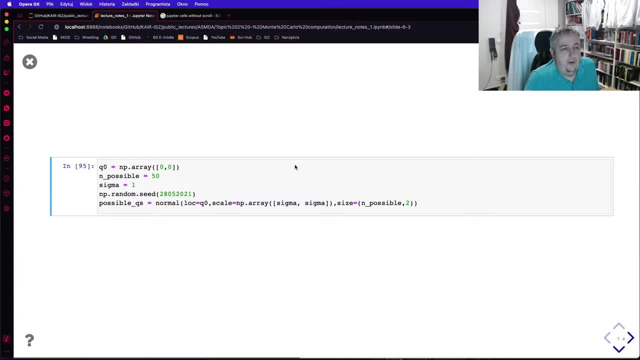 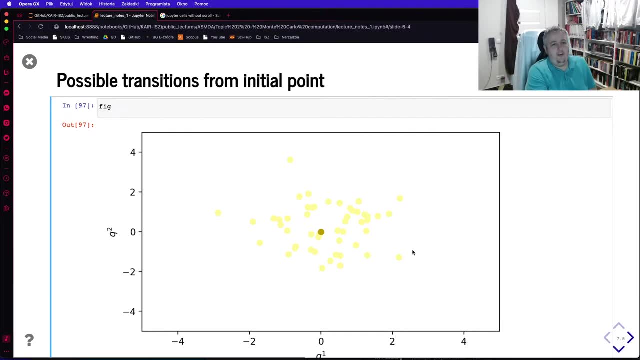 That Sigma Is Equal To One. We've Given See A Random Seed. Let's Start With Point Up Of 50.. Possible Movements: Points That Where. 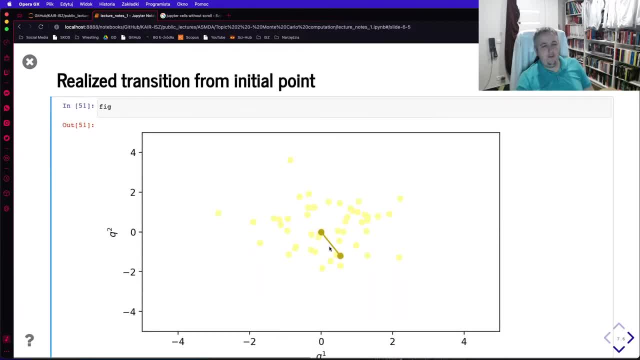 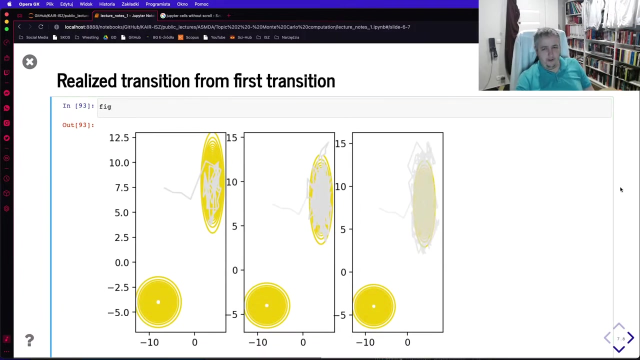 We Can Move To From 0. 0. To Here, Conditional On That Distribution. When We Move The Transition Is Realized. So and something failed here, but generally such movement is possible. 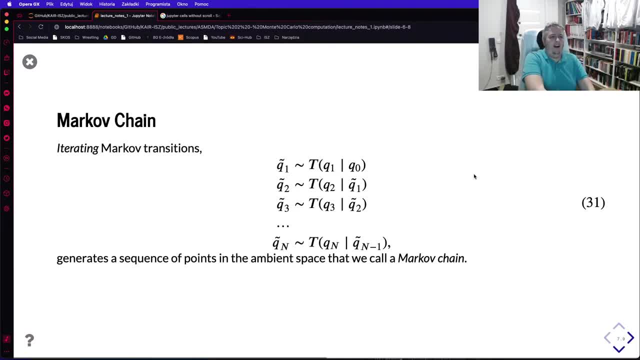 So iteration of Markov transitions is relatively simple. so the Q1 is distributed by probability of getting Q1 from Q0, and similarly, from the point Q1 wave we can get until we can get probability of getting Q2 starting from that point, and so on, and so on, and so on. 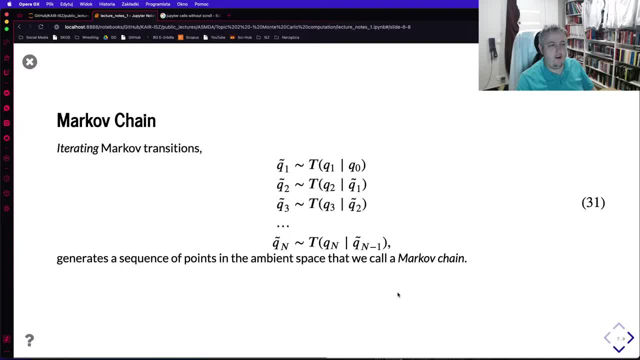 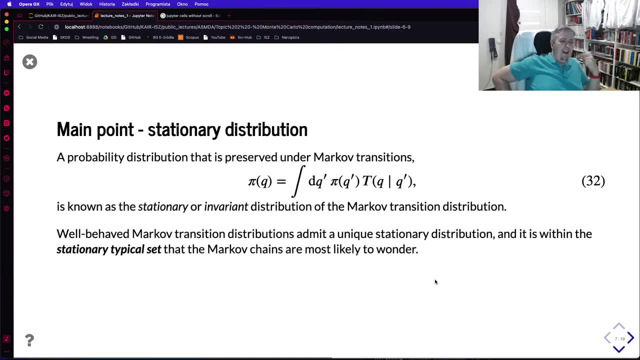 So iteration of Markov transition generates another sequence of points in the space that we can call the Markov chain. The main point here is that, Well, If there is a probability distribution, that is preserved on the Markov transition, which means that if we integrate such 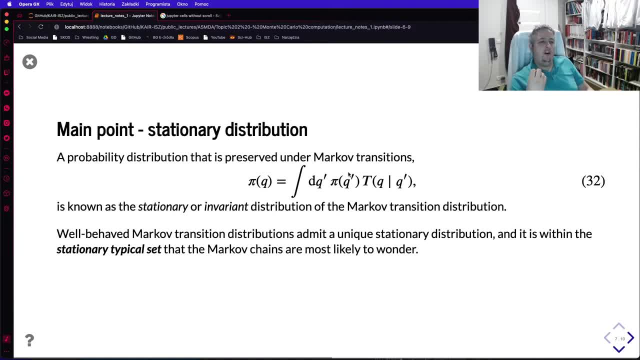 situation We marginalize Q prime from the distribution and we get the same probability. This is callnd as stationary on intert State the probability no longer труБ of the order of the ordination. invariant distribution of the Markov transition distribution And well-behaved Markov transition. 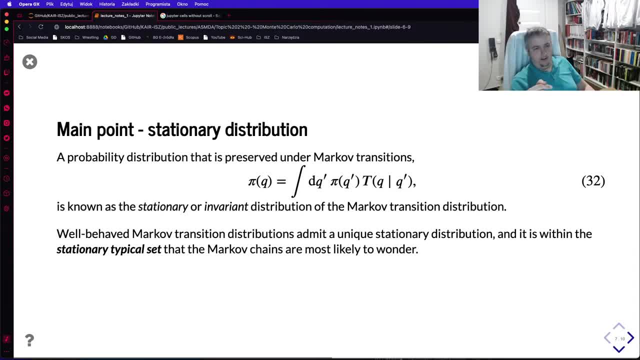 distribution, admit uniquely defined stationary distribution, So it is not possible to find multiple such things for well-defined transition distribution And, what is most important, that Markov chains will wander through the stationary typical set, so the typical set of the stationary distribution. So, as we remember from the previous lecture, typical. 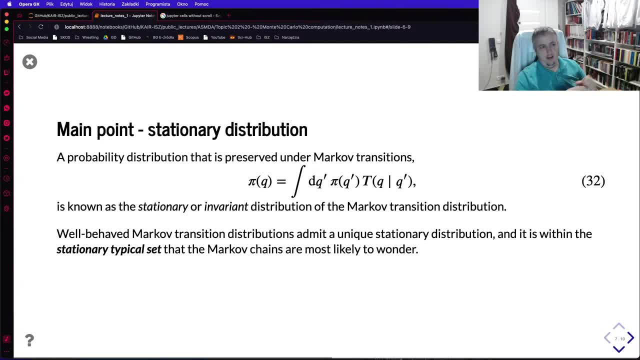 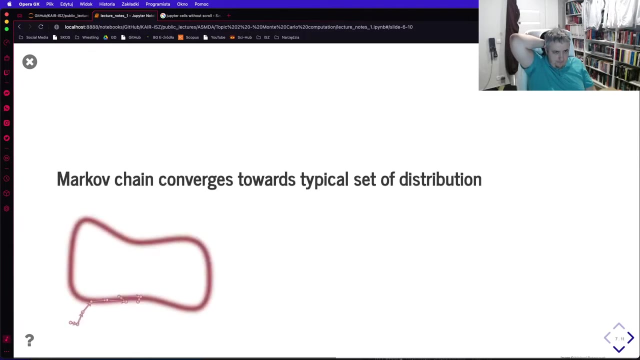 set was the place that most of the expectation happened. This was the places that contributed most to the expectation integrals because they contained a lot of volume of space and not necessarily the places where the density was highest. but the biggest contribution to the probability distribution And Markov chain converges to the typical set of its 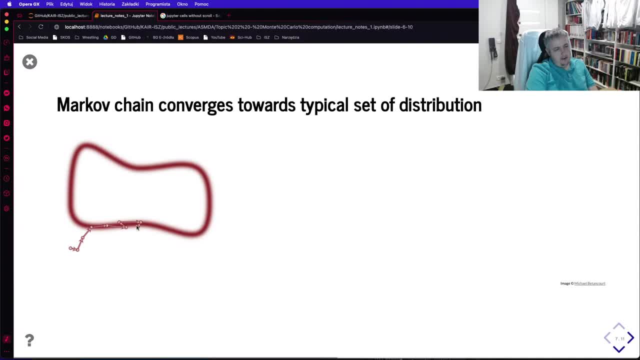 stationary distribution, So it starts away from it, and if this fuzzy set is the typical distribution, then we get a convergence and after that it stays in it, because the other word that we used here is an invariant distribution, So our distribution is an invariant in the 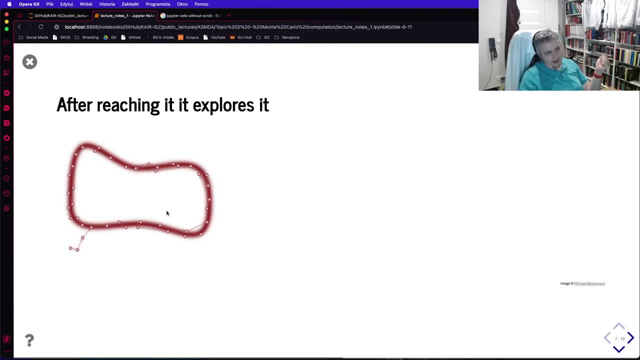 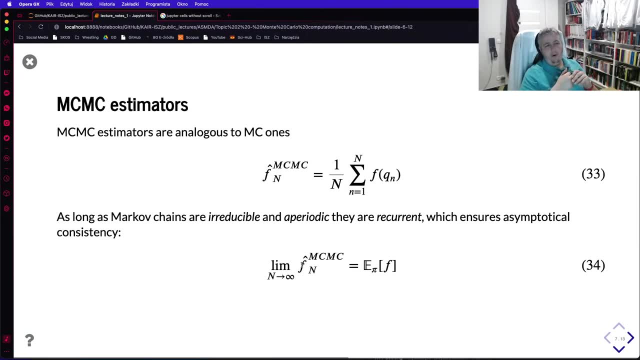 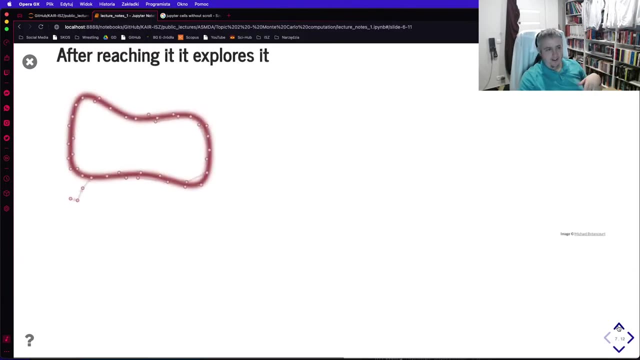 Markov chain, because when we've localized ourselves in a typical set, we are staying in it. And what is important is that Markov chain, Monte Carlo estimators, what we mean here. we mean here that sampling from getting the sequence of Markov changing samples from a sample of aаnex, we can flow between in them. 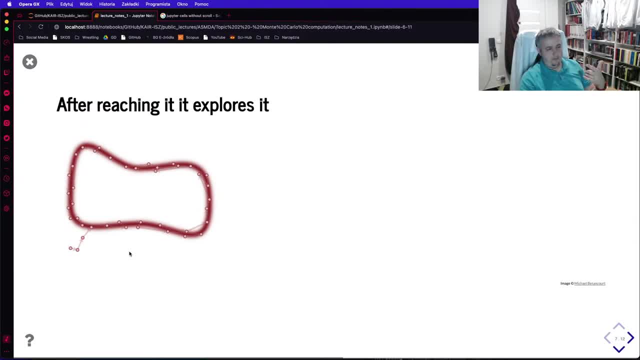 but the sequence may be convenient. This is just an example. One is nearly impossible, but the sum isbuilt to the incidence value of it is much less important. такую ii s, s, vy, t m tariffs. I s, f, ve, I s c? e. 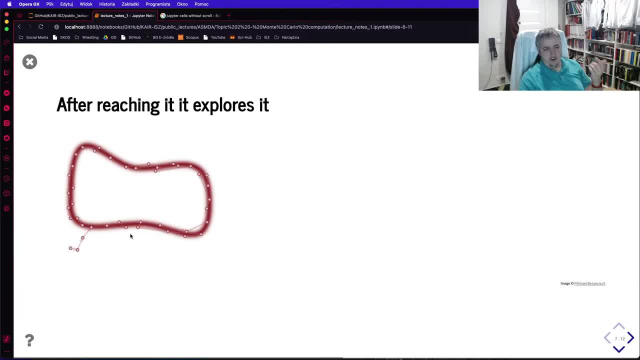 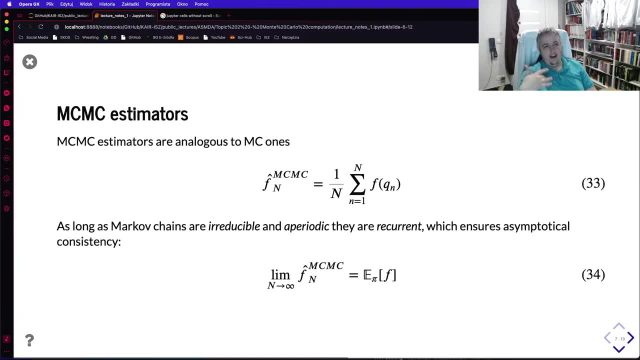 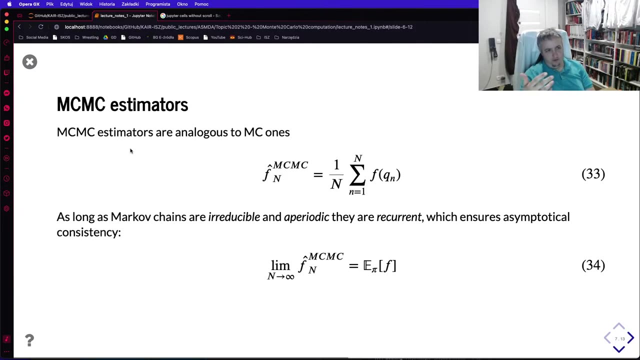 are in the typical set of stationary distributions. So they are samples from the stationary distribution located in the typical set And because of that if we want to create a Markov chain estimator for the stationary distribution, those Markov chain estimators work exactly the same way as. 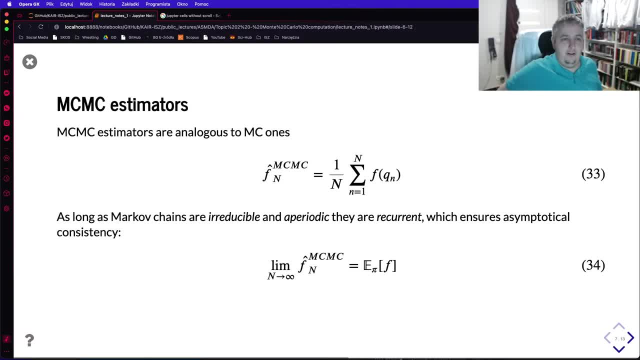 maybe not exactly, but a similar way to the Markov chain, to the Monte Carlo estimators. So again, it's an average of samples of function f And the important aspect is that our Markov chain, with a given stationary distribution, pi, needs to be irreducible and aperiodic. 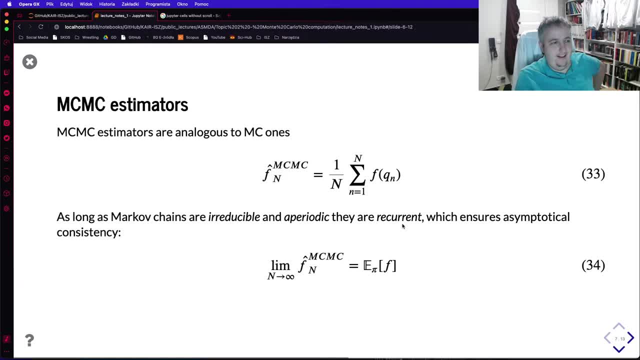 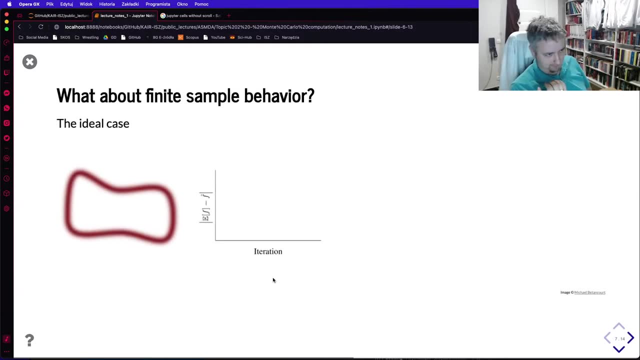 which gives them the property of recurrence, and this ensures that Markov chain Monte Carlo estimator will converge To the expectation as long as n goes to infinity. But this is infinity What? in a situation where we have infinite number of samples, which is a situation also known as life? 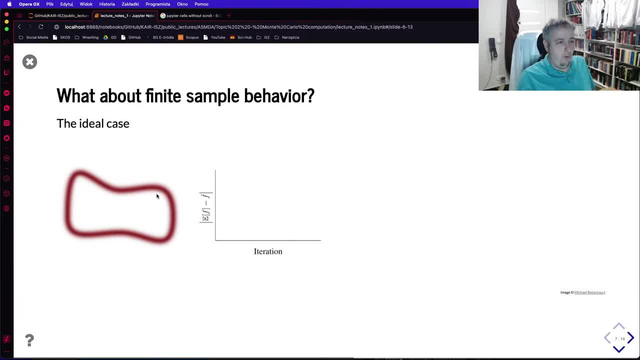 So in the ideal case, considering what is the difference between expectation and our estimate, we can see that initially we converge to the typical set, then we mix it and explore it and finally we get refined values of our expectation, which might take some time after convergence. 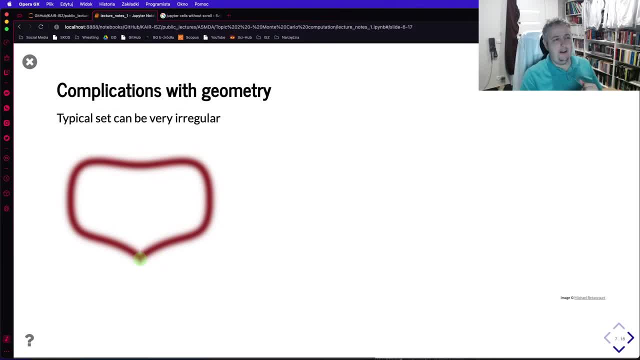 Unfortunately, depending on the problem, the typical set can be very irregular. For example, there can be some cold funnels or places where where the geometry of the typical set is very, very not nice And that issues a problem in a transition. 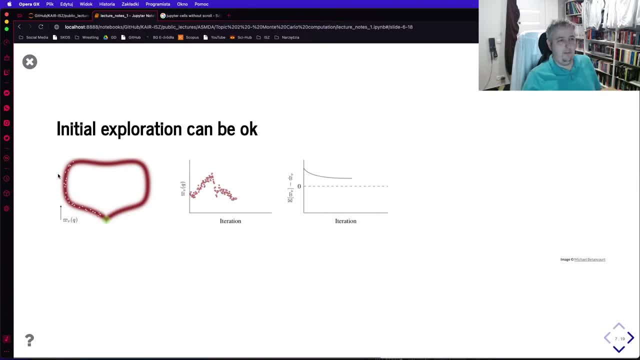 because, starting from sampling the distribution with Markov chain, we can get some kind of convergence to the expectation. However, when we get to the difficult shape, then the transitions might get complicated because, for example, we might have a lot of difficulty to leave that transition. 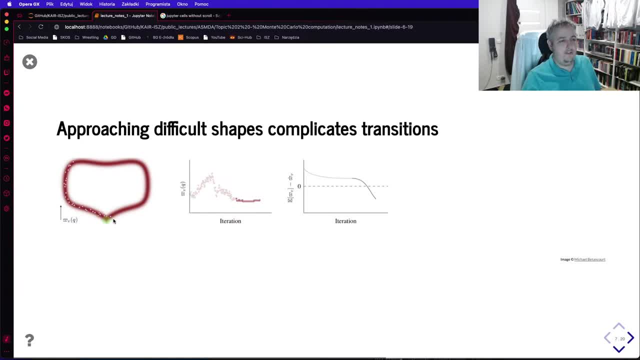 so we get an over-representation of samples in here, And even we escape this irregularity, we still have too many samples here, so we got the bias that might be difficult to correct. Also, the problem is that in finite cases, if the typical set of the distribution is not necessary, 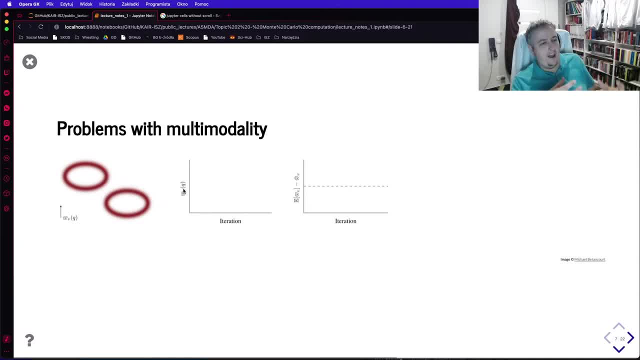 a connected space or general distribution is multi-modal, then one mode can draw the Markov chain totally and ignore the situation. And if we are not careful we may think, okay, we've explored the set and we do not know that. 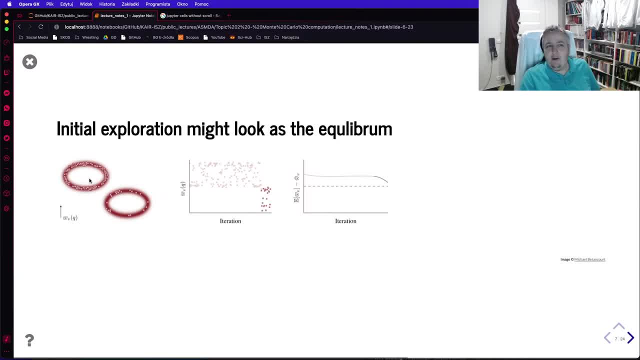 We do not know how it will look like, because the expectation is much more complicated, The analysis of the set is much more complicated, So we don't know that. So we may stop too early and after some time we might move away from the equilibrium. 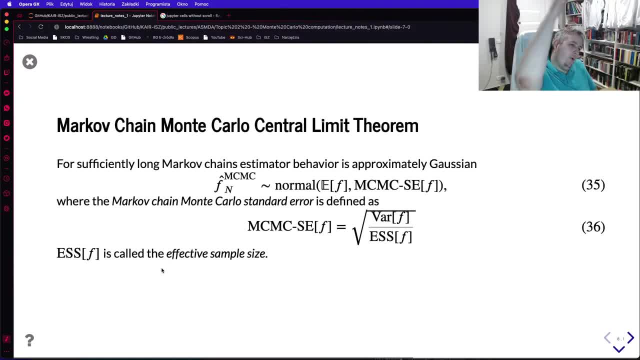 So, moving that, we move to the so-called Markov chain, Monte Carlo central limit theorem, because, in a similar situation as with the Monte Carlo standard limit theorem, here we have, however, averages of random samples, So they should behave approximately Gaussian. 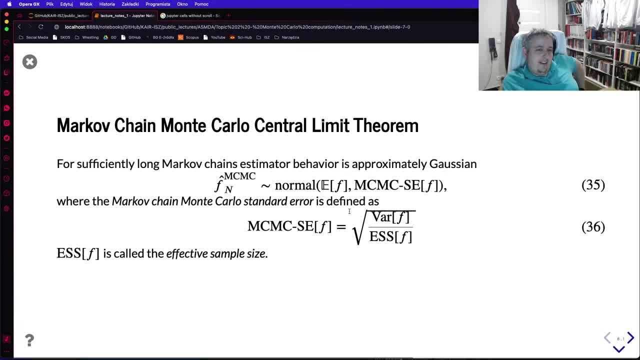 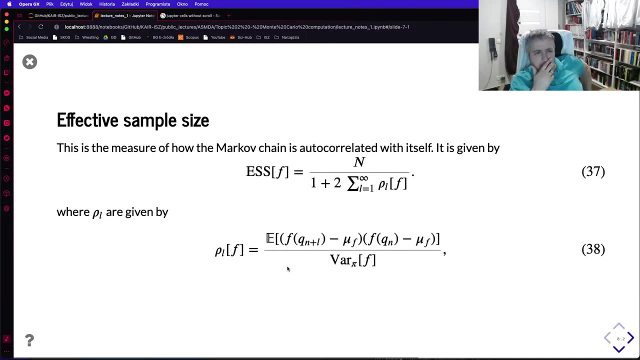 However, we have a problem that in case of Monte Carlo standard error, we have so-called Markov chain, Monte Carlo standard error, which, instead of number of samples, includes something called effective sample size, And effective sample size generally is a measure of how. 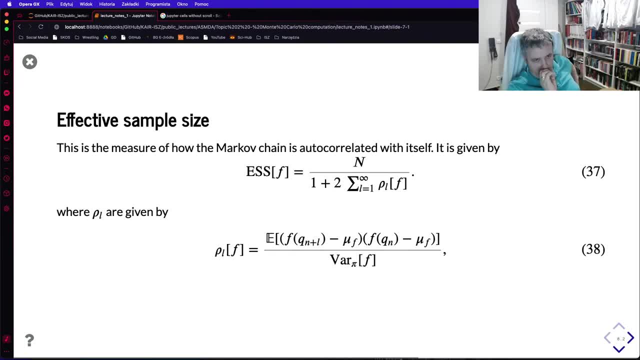 a given Markov chain is autocorrelated with itself, So of course we would like it to be equal to n. So we want to have no autocorrelation, And in that case we get n divided by 1.. 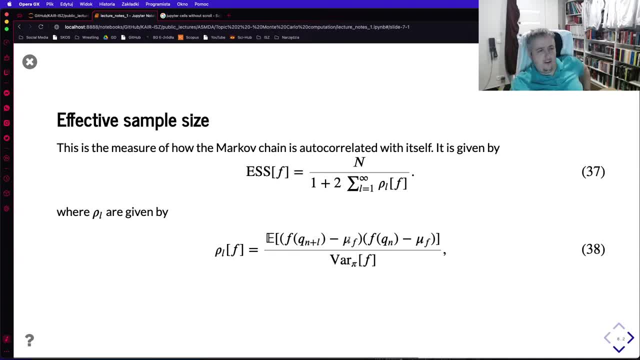 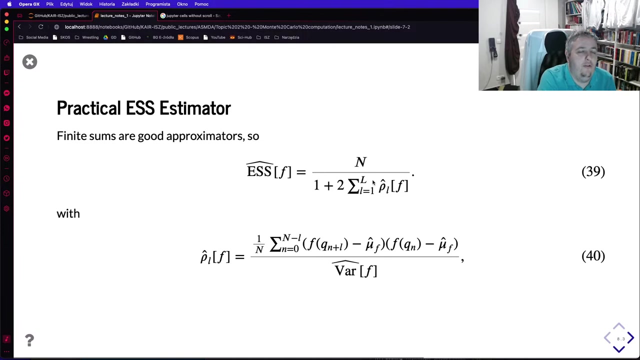 And autocorrelations are of course given by the cross-correlation between those two samples divided by sample variance. Practically, the problem is that here we have to test for infinite possibilities of autocorrelation. In practice, we get up to certain level of autocorrelations. 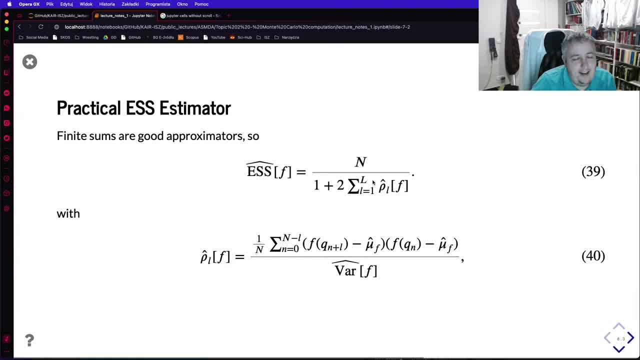 that we can expect to be reasonable. And again, if those will be 0, it will be great. If they will be large, then we have a small estimated sample size. And what can cause those autocorrelations, For example when we are in the 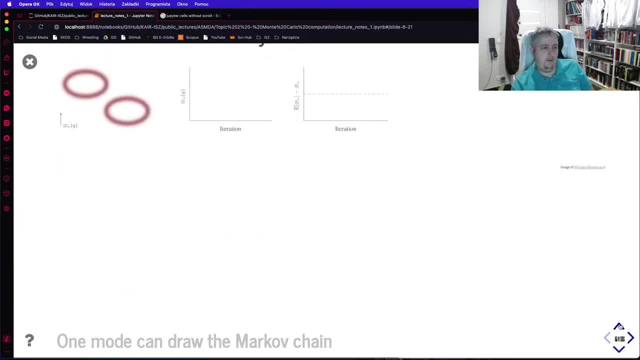 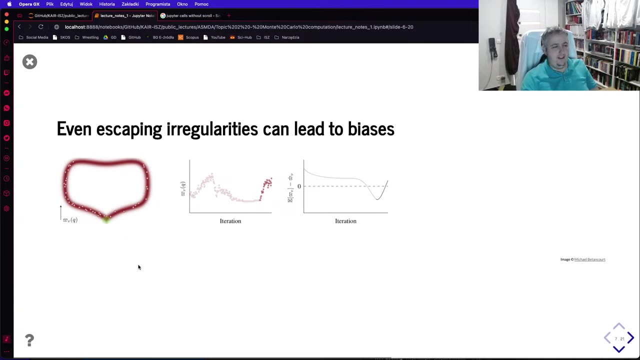 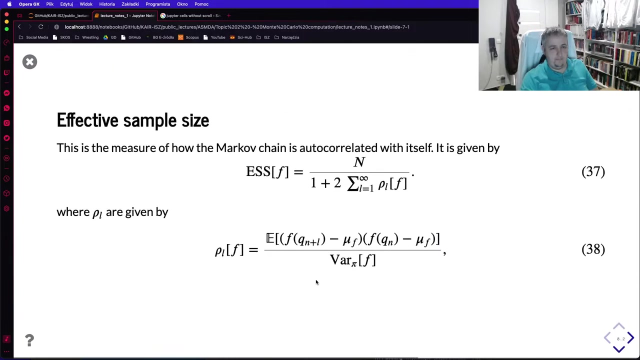 funnel here, so we are getting samples very close to one each other. they are strongly autocorrelated with each other. So autocorrelation in our sequence is significant because all of them stay very close to each other. So there is a very strong autocorrelation. 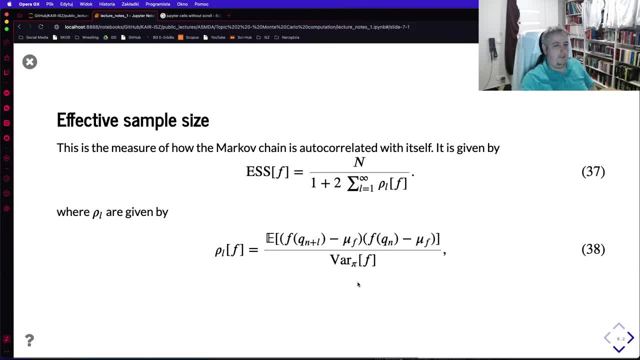 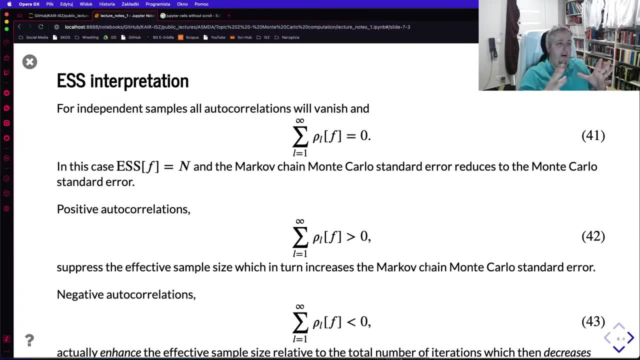 So getting that will be very important And now we have to try to think about how do we get some problems and drop the effective sample size And generally if we have independent samples, all of the autocorrelation will vanish. Estimated sample size is equal to n. 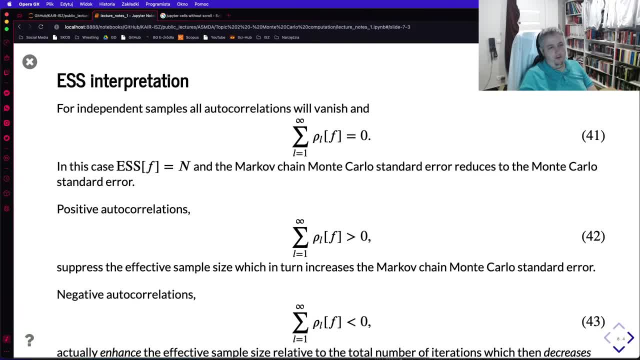 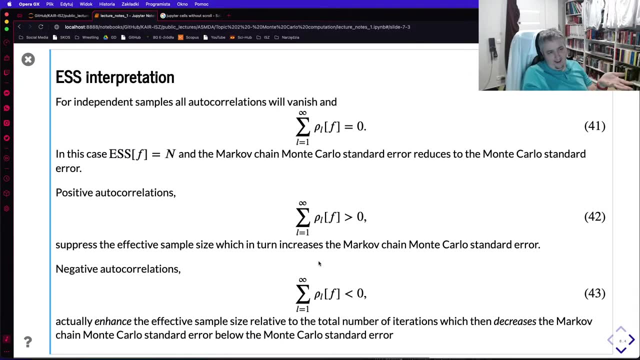 A Markov chain, Monte Carlo standard error reduces the Monte Carlo standard error. Second case is when we have the, when we have, when we have some kind of positive autocorrelations. So in that case the effective sampling size is smaller because n Monte Carlo stop-data rises, because in that case n is divided by something greater than. 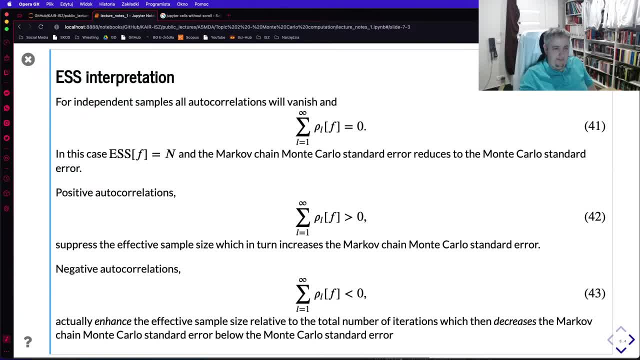 and so it will get larger than, because ASS will be smaller than n. In a very special situations we can have negative autocorrelations which can actually enhance the effective sample size relative to the total number of iterations, which then decreases the Markov chain. Monte Carlo stop-data error. 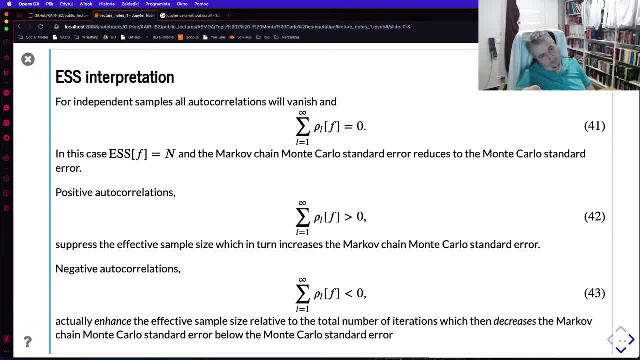 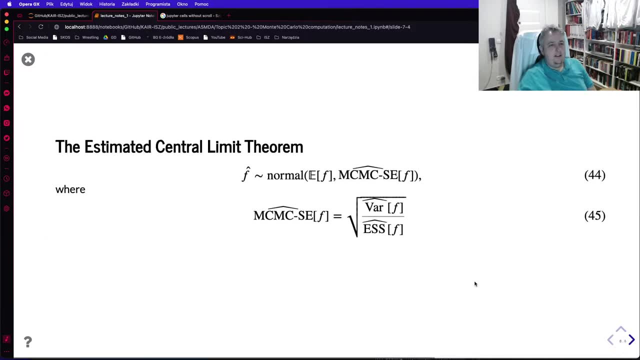 below the Monte Carlo stop-data error. but this is unreliable. It might happen for one initialization and not happen for the other. You cannot design another algorithm that will ensure that. So we get so-called estimated central limit theorem, which gives us the error quantization as the Monte Carlo Markov chain standard error given. 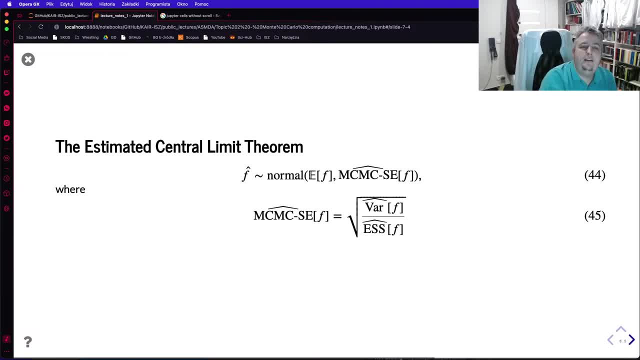 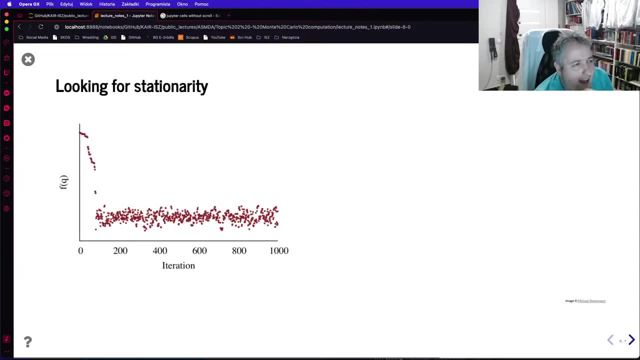 by square root of sample variance divided by the estimated sample size, And that's one method of diagnostics. The other thing is that we how do we verify if our samples are coming from the typical set? So we, for example, look for stationarity. 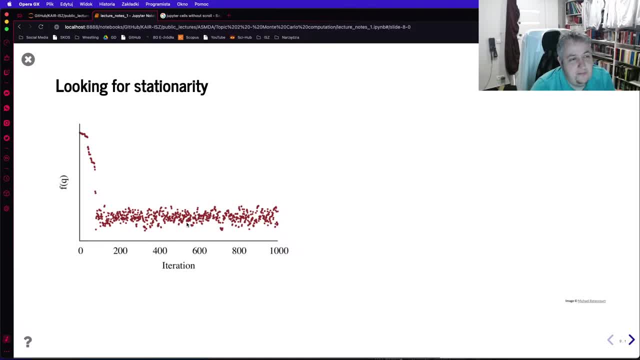 So we look for the situation where the exploration of of individual variables is consistent. for example, they are located in one neighborhood. however, we can get such situation that is very complicated, like freezing, that what I've shown before: the samples are staying close to the funnel, so they are not moving and that introduces biases later because there's 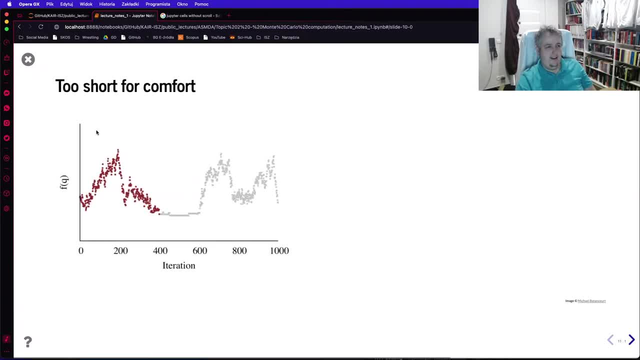 very, very little movement around it. if we cut our chain too short, then we might not observe that situation. we just get wrong computation- and this is a very difficult case in case of Bayesian computation- is that if we are not careful, our computation can be wrong and it won't scream at us about it. that is. 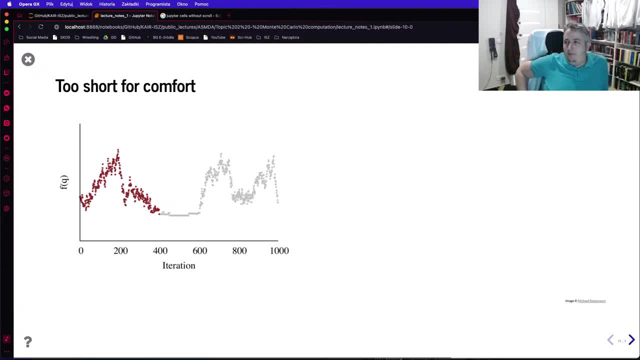 why Hamilton Monte Carlo is very good, because it's true matters that we did something wrong and we'll discuss it next week. and observation of that, might we the changing the initialization. if you have a multiple distribution, we might get a chain that will look differently, so it will get stuck on the different levels. 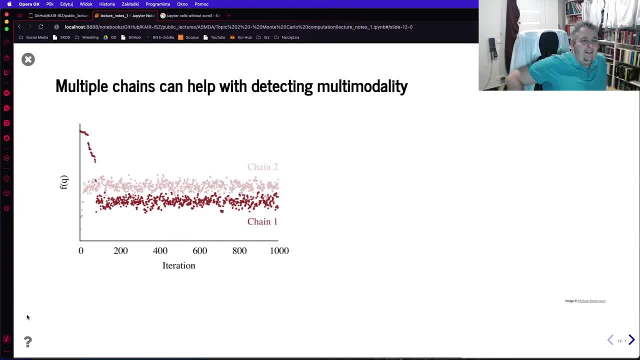 so we get stationary at the different levels and that's why it is very often- to you been very often- we use multiple chains, because multiple chains will get us some information, will may give us some kind of independence of this initialization point. if we started in initial point here, then maybe starting from multiple 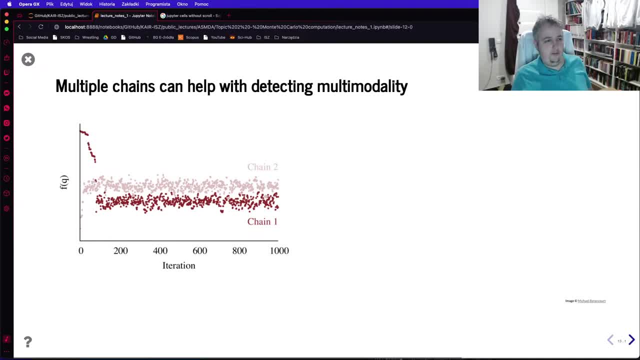 points will give us to get us to different results, and getting us to different results will be beneficial generally and also having multiple chains. we might find some problems that we would observe earlier because, for example, some chains might not freeze in the short number of samples that we are. 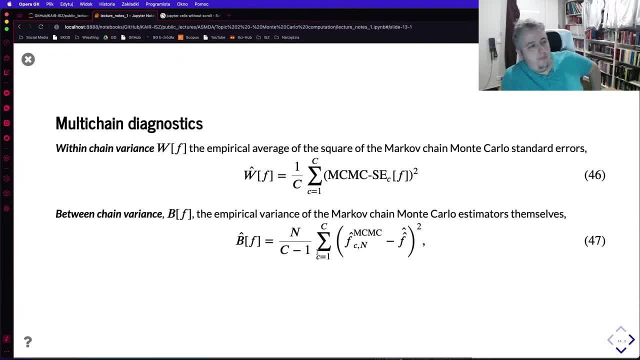 considering. of course, observation of chains is a very good method generally, when we can look at figures and we can understand what's going on them. this is a very good situation. unfortunately, we would. it is not always practical and that's why we want to get some kind of matters for diagnostics that will just give us a 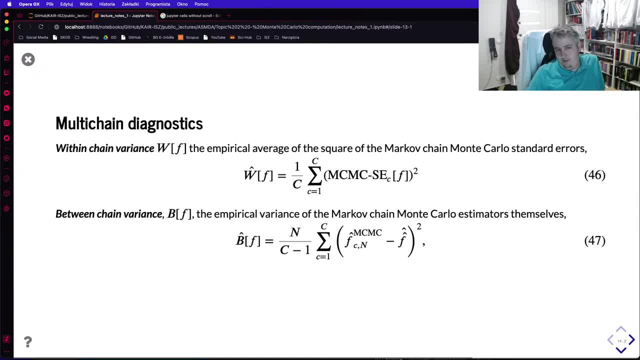 number, good, bad, to optimize something, to operationalize something, and for that we use such a quantity like, for example, within chain variance. so this is an just a value of empirical average of the square of Markov chain, Monte Carlo standard errors, or we can use between chain variance so we get the empirical variance of each chain. 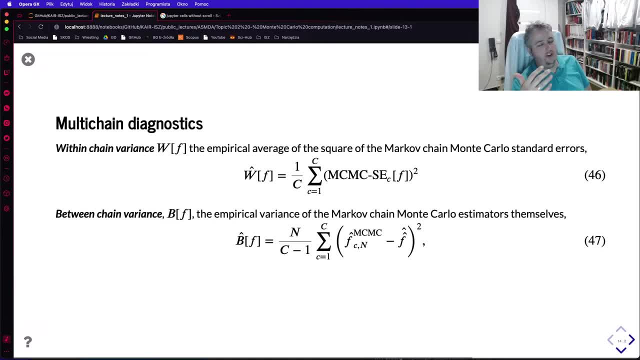 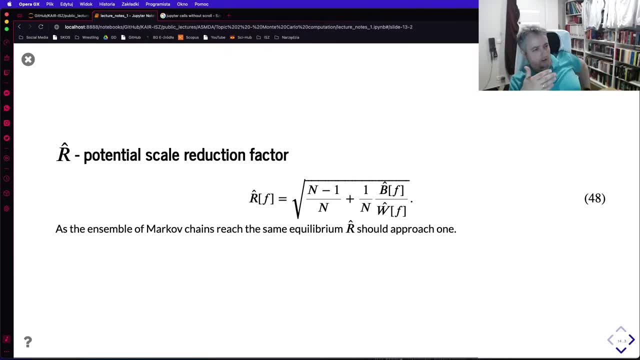 between estimators each other so we can see how much each chain differs from one another, and those two are useful. or a very important diagnostic tool, which is an R hat potential scale reduction factor, which actually is now computed in a bit different way because certain rank statistics methods are much more robust. however, the R hat generally says is like: 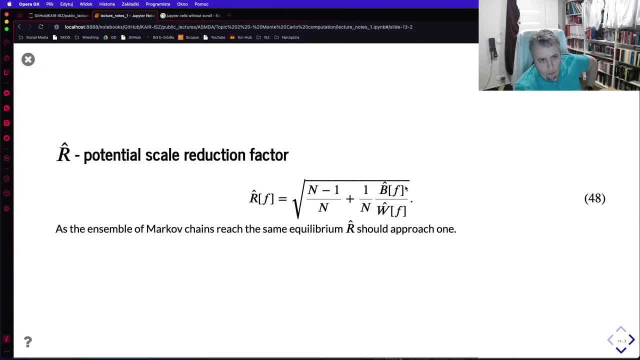 this: if within chain variance and between chain variance are equal to each other, so each chain mixes itself as all those together, then in this case R hat becomes one. if between chain variance is larger, then we have a different situation. if, but if between Chinese is smaller than actual, 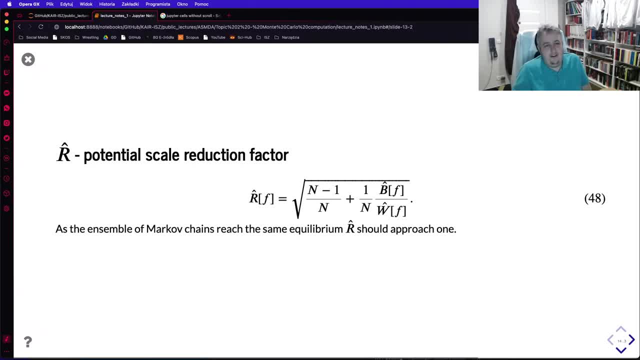 is actually different is actually kind of kind of weird. but generally this situation: if between chain variance is larger than within chain variance, then in this case we have a larger number here that will make our R hat greater than one if all those Markov chains reach the same equilibrium. 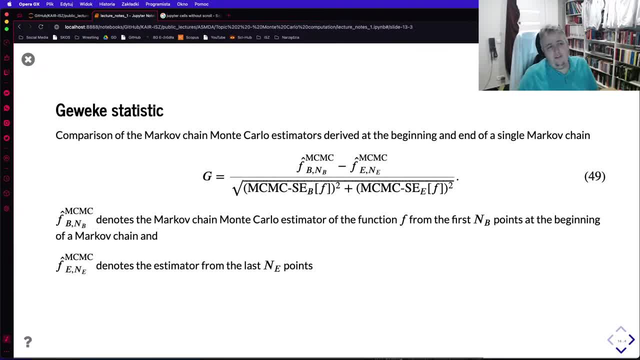 R hat should approach one and different ways are, for example, Giwicki statistic, which is a comparison of Markov chain, Monte Carlo estimators from there at the beginning and the end of a single chain. so we get an estimator from the first points and from the end points to get a better estimate how it will work. and 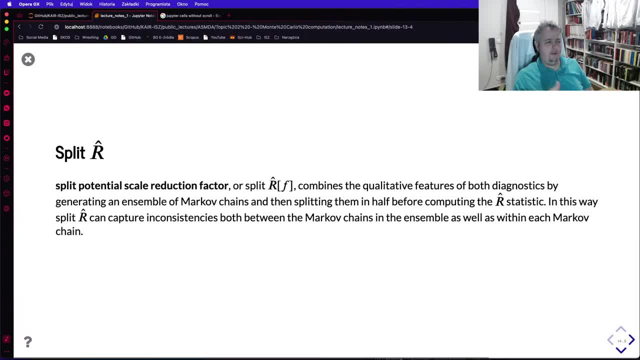 generally idea that once connects those two is the split R hat, which is a modified version of a R hat which is called a split potential scale reduction factor, which generally gets our, instead of doing R hat between all the chains, it splits all the chains in half and 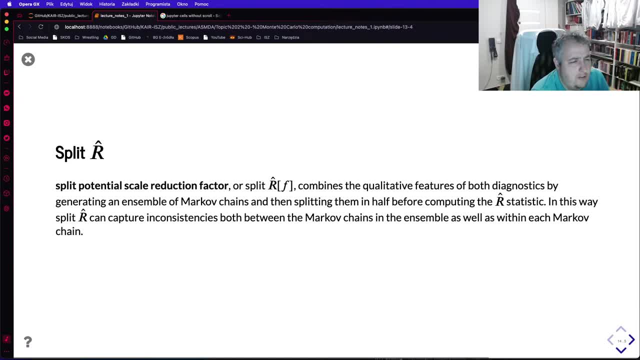 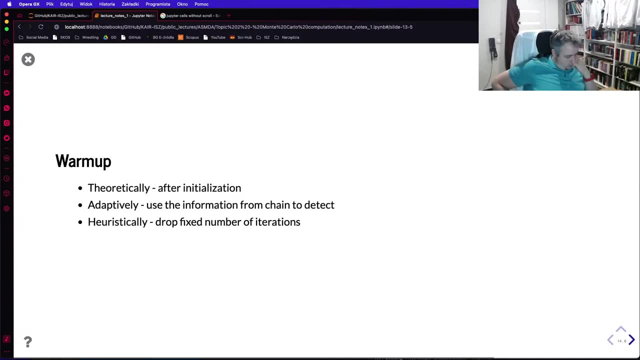 takes half of and instead of, for example, four chains, uses now eight chains to compute a hat, so it can get also some inconsistency within chain itself and not only between chains one another. so how is that? nice, but, and we can diagnose it. but of course there is in one problem. this problem is that when 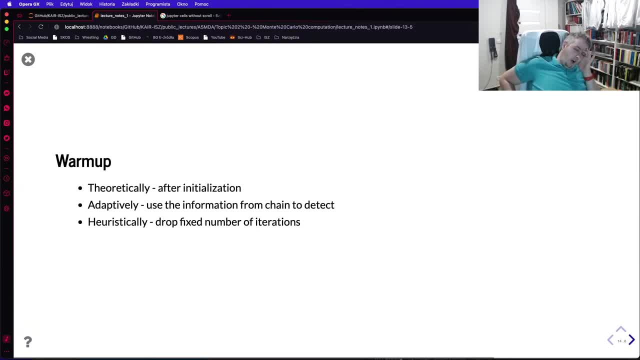 we start sampling, we don't necessarily are already in a typical set. so this typical, this approaching of the typical set, will introduce some bias. so we need to handle it in a way and well. originally it was being called burn-in, so like just with burning, until that we are into chain. now it's called warm-up. so the algorithms. 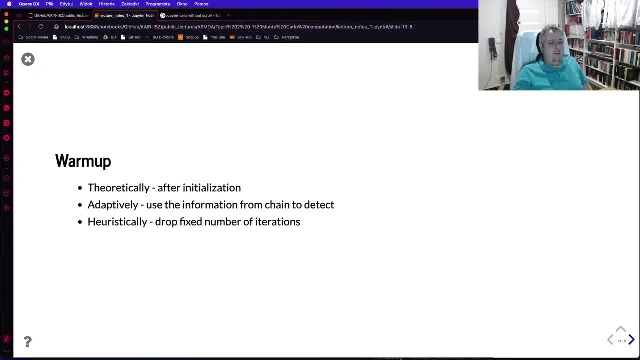 getting improved some, and there are three ways to get it. theoretically, after we initialize, we could use these samples when we get into the typical set, but how we get into because that well, that's a problem, so so we don't use it. and if we just start from initialization, we get the biases which will 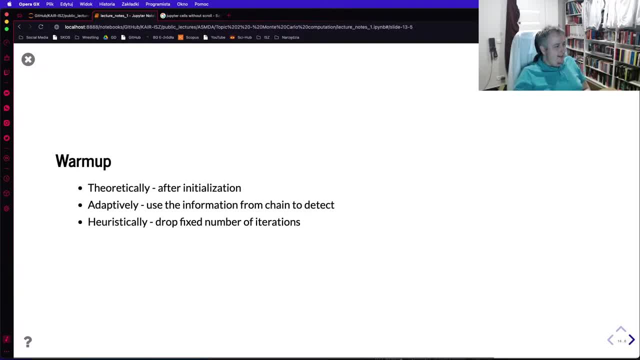 need more samples to go to the code. there are ideas of adaptively uh deciding that, oh, we're in. unfortunately it is not that very reliable. we can use some information from chain but we can get problems in it because practically there's a heuristical approach, we just drop fixed number. 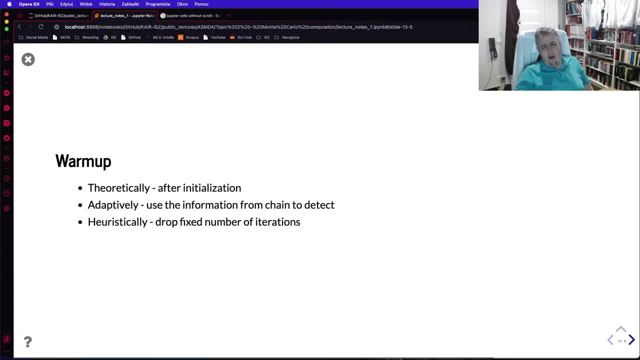 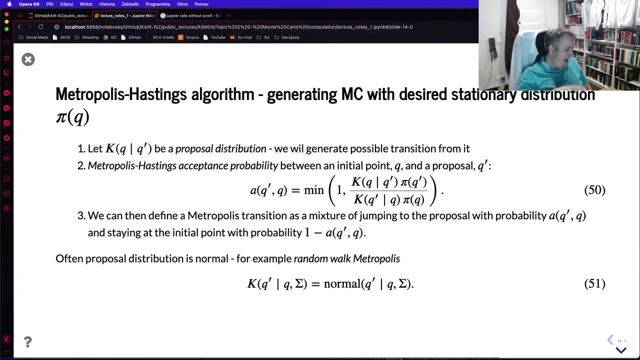 of iterations, usually for for a 1000 sample chain. we drop 1000 samples earlier, so we get after a half. this is a default, for example in stan, which is a good, good approach to to get started, and we now go to the conclusion of this discussion. so how to get my mark of chain with a desired 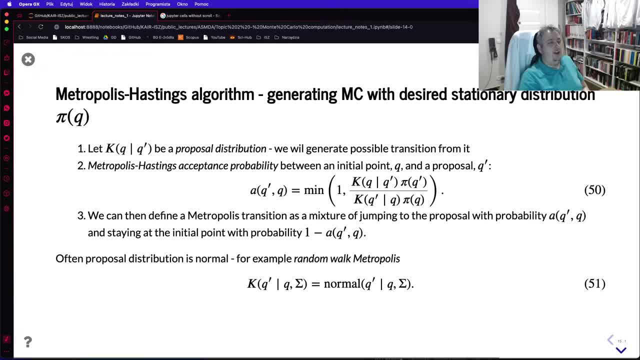 stationary distribution, because we know that markov chains can have stationary distributions as long as we provide them with certain conditions. but how to get a recurrence mark of chain with a given distribution? and that was solved by metropolis and hastings, so-called uh, which is one in an 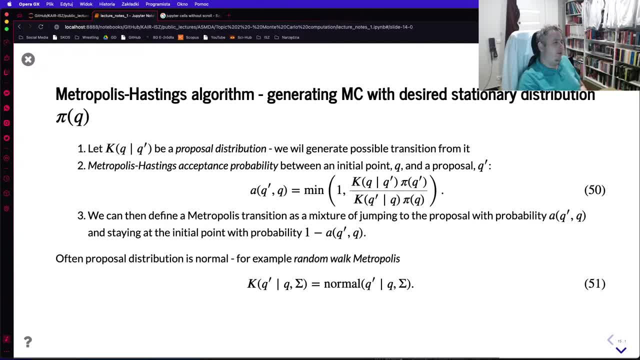 algorithm, which was called one of the most influential algorithms of the 26th century. it was created in los alamos laboratory, the same one where the project manhattan was was done, and generally the idea of the algorithm is as follows: first of all, we get some kind of proposal distribution. 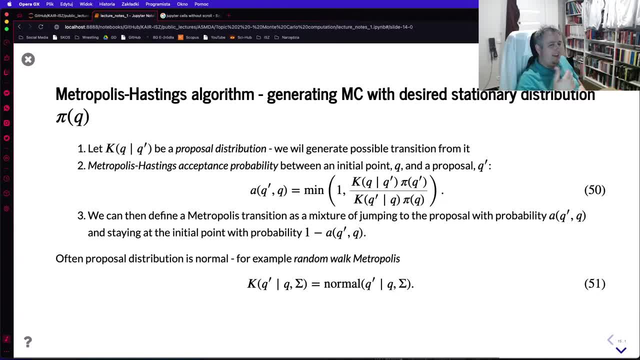 this proposal distribution is a distribution that we can generate samples from, for example a normal distribution. normal distributions are nice because we know how to sample them, even in multiple dimensions. if we get the sample sample from the proposal distribution, then we compute something called acceptance probability between the initial point and the point sampled from this proposal distribution. 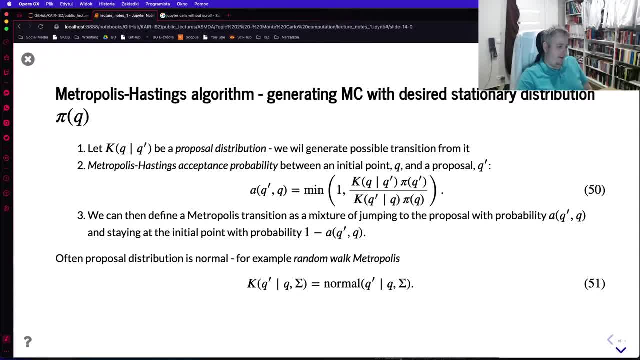 And this is computed as a minimum between one- so we cannot get greater probability than one- and certain correction term which contains both the proposal distribution terms and the desired distribution terms. So when our samples are different from each other, we need to know how to get the probability distribution. 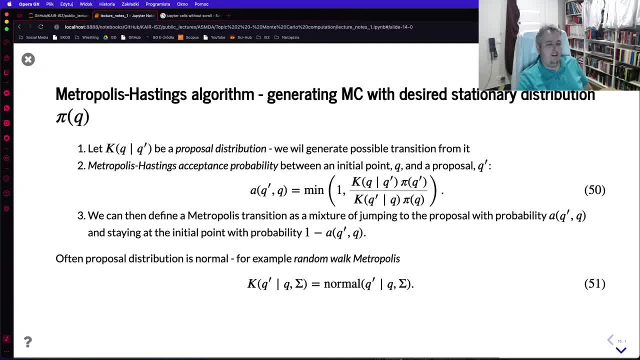 And then we can define the metropolis transition as a mixture of jumping to the proposal with a probability equal to a, from q prime q and staying at the initial point with a probability of 1 minus a times q minus q. So when our proposals lead us to points of high likelihood or high values of density, 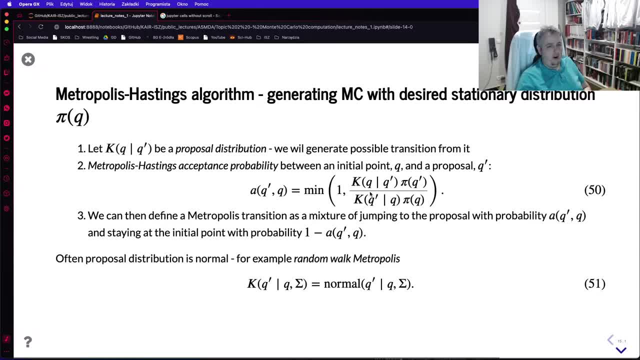 then our numerator becomes larger and, depending on the other terms, we can solve the problem. So when our proposals lead us to points of high likelihood or high values of density, see that so, like if we go towards the larger values of probability, then we get the. 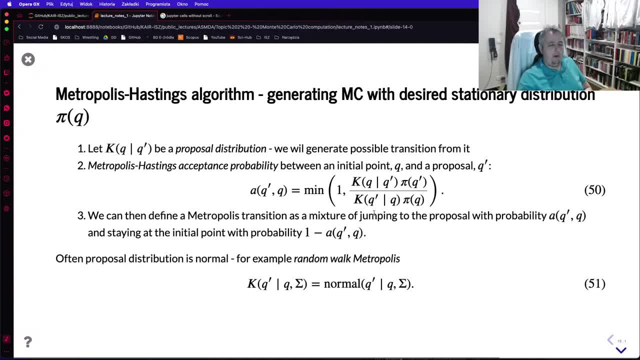 of this the function, then we can get a bigger probability to move there if we move to the areas of small probability than previously. so q prime is p of. q prime is less than q, then the priority is smaller, however, because we allow ourselves always to get some kind of probability of 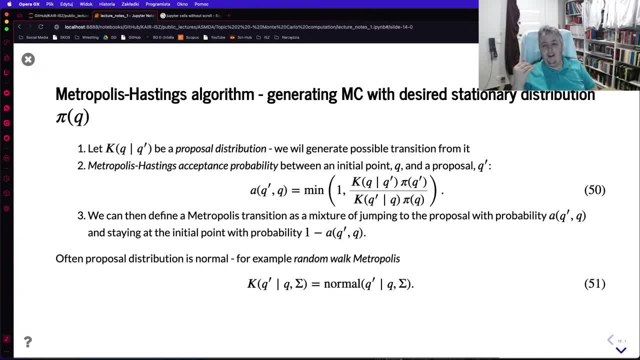 transition, then in this case, uh, there will be no risk of getting stuck in some kind of minimum of the function, because there's always chance to move away and, as i said, the proposal distribution can be normal. in case of the famous random walk metropolitan algorithm, you get the proposal. 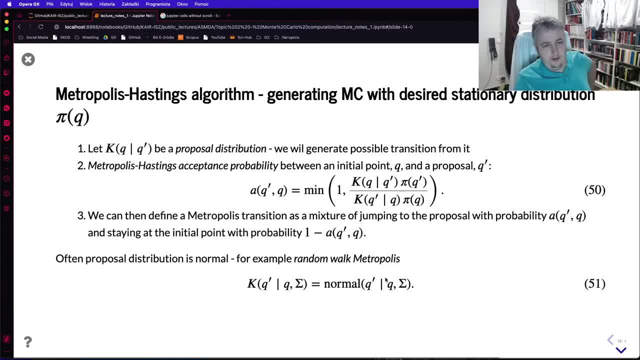 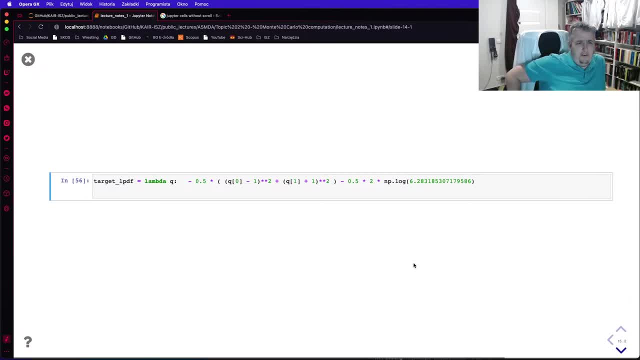 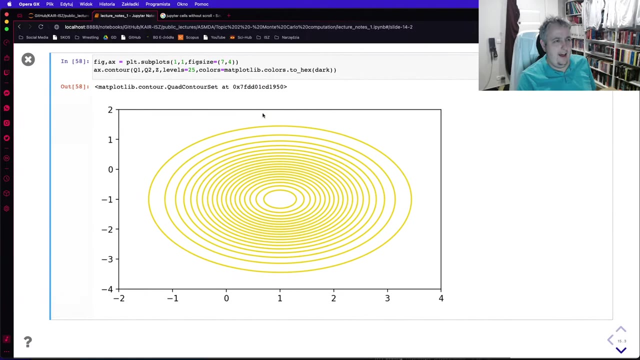 distribution as a normal multivariate function distribution with some kind of covariance matrix signal. some examples: let's start with a very simple function which just is a a normal function. this we consider a logarithm of the probability function, and just it's so. it would be much, uh, easier for computation and of course we can plot that using the. 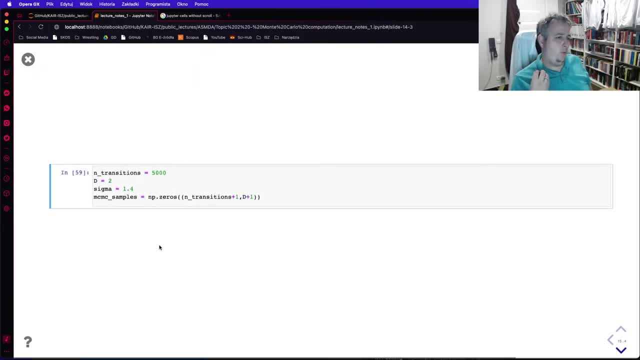 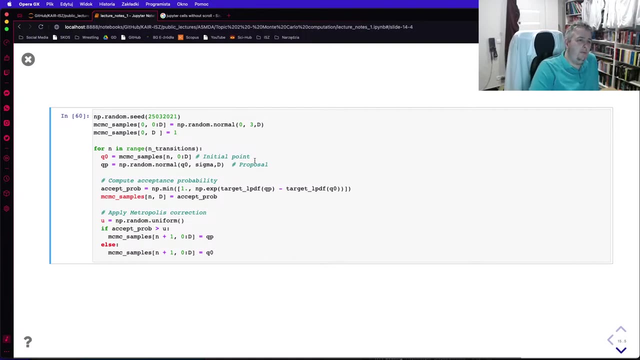 the contour plots and we can start doing transitions. so we start from our proposal distribution, we get the proposal distribution and we get the equal and at the end of our transition we will get the solution which is independent unit size, which sigma one point four, and we get in our algorithm. so, starting from random numbers, we 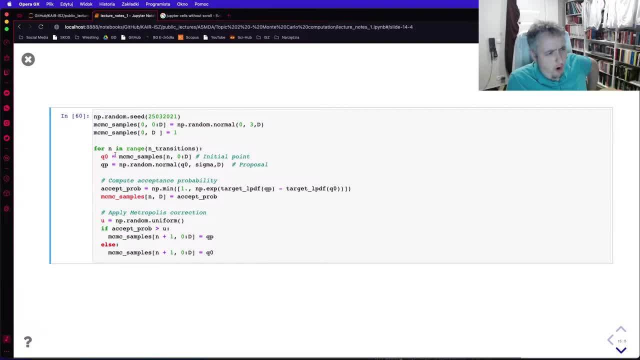 get. we will generate those random normal uh numbers, and so for n in our number of transitions. we move from point q, zero, uh, we get the proposal, uh probability, and then we get the proposal and we get the acceptance probability, which will be, of course, minimum between 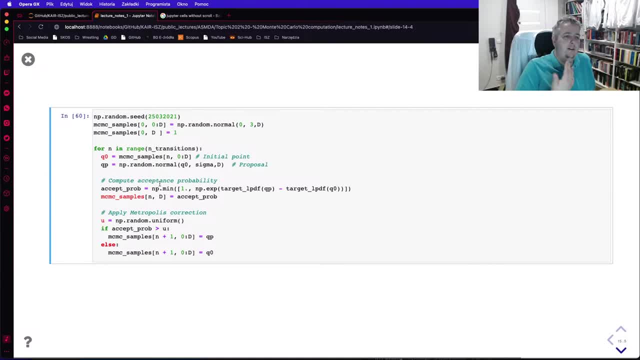 one and our distribution function. Why such construction? To avoid numerical errors. Instead of dividing two normal distributions, we just get the exponent of their division, of their logarithm, difference of their logarithm. So this will allow us to avoid potential numerical errors when computing values entails- And this is a popular practice- in the probability. 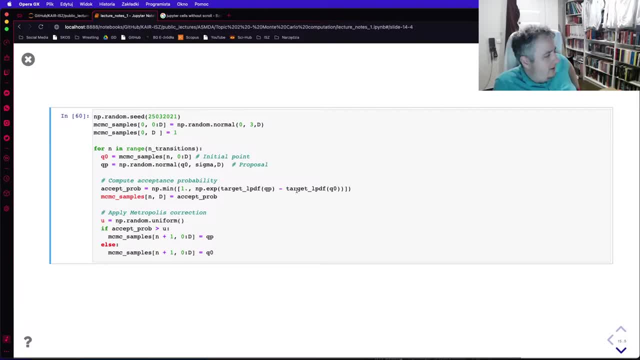 computation to work on logarithm densities, because most of densities are in a form exponent of something or most popular used And in such case those that entail values. you get very, very small values of probability density function which can be lost in rounding errors. 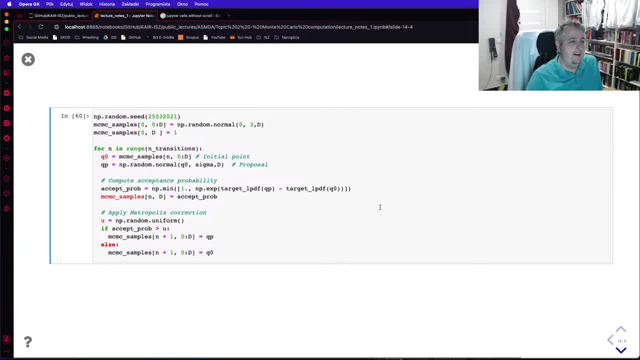 And if you want, If you want to work on logarithm, that situation won't happen. So you save the acceptance probability. and then what? Using the acceptance probability, you get a random number and if this number is lower than acceptance probability, then If it is lower you stay here. If it's lower, 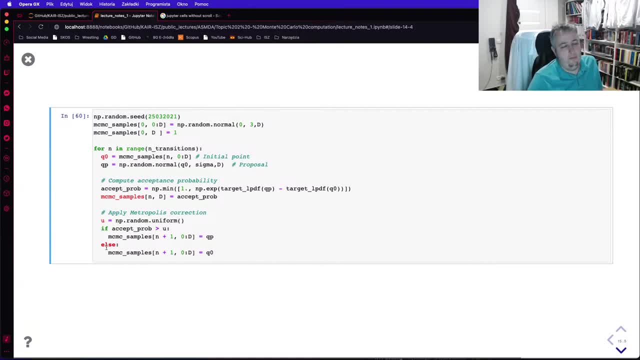 then you work and then the number is: If this number is lower than acceptance probability, you'll move to a new transition. if it's higher, then you stay in the situation. So this is a mixture of moment: you move to a point or stay, depending on the probability. 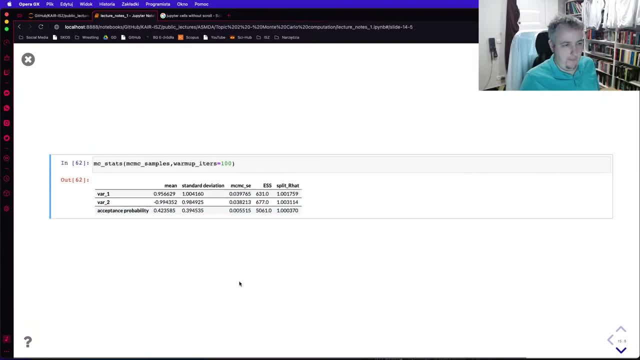 threshold which moves step after step And, as we can see, we can get multiple stats from that. So, from our distribution with mean of 1 and minus 1, we get the And that's all. Thank you very much for being here. 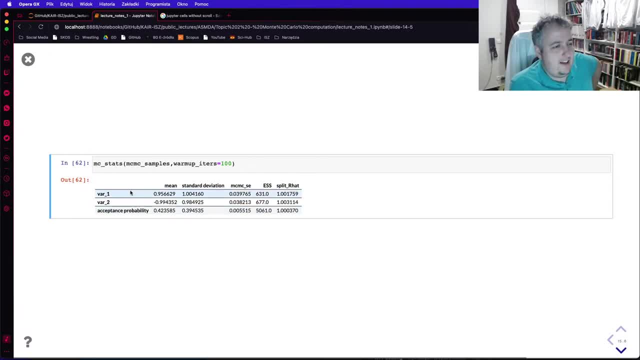 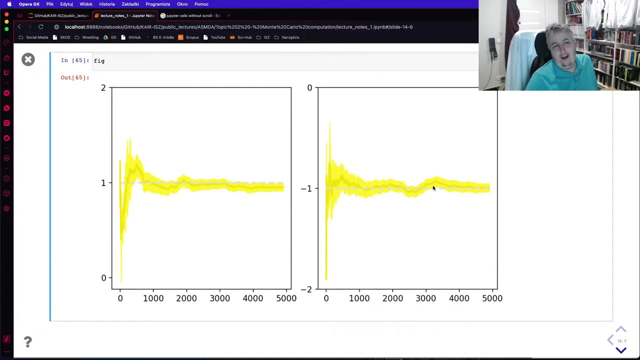 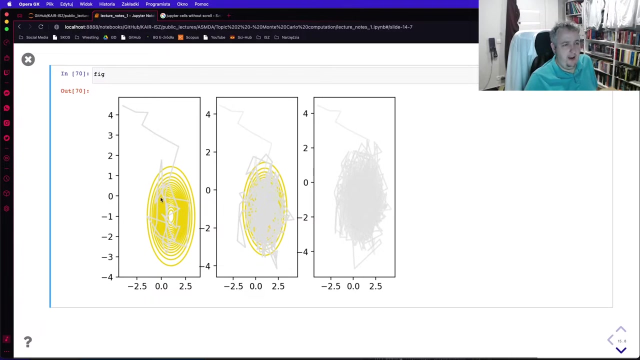 uh, our viruses with significant standard deviations which are justified, and we get the uh, our very small moment across the letters with reasonable expected uh sample size, with splitter hat approaching one and, as we can see, uh, we have rather nice convergence to the expected values in a two-dimensional space with first get this transition initial, to get to the neighborhood of. 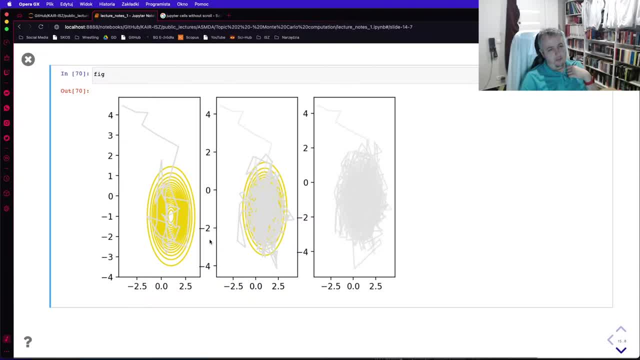 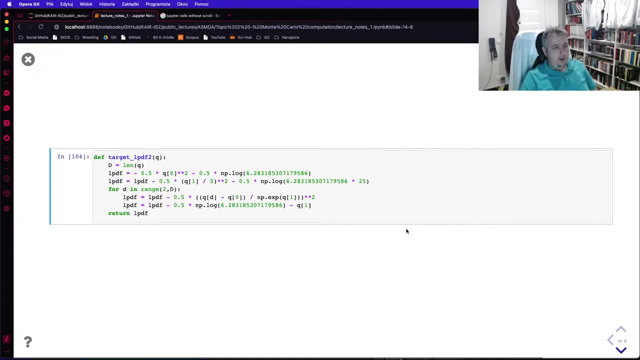 the uh of the typical set and then we start to covering it, moving around, moving around, again covering it. if we get more complicated example, we will get an example of multi-dimensional distribution and this very specific distribution in which the first two variables are influencing the shape of other ones. So our first two variables are just given. 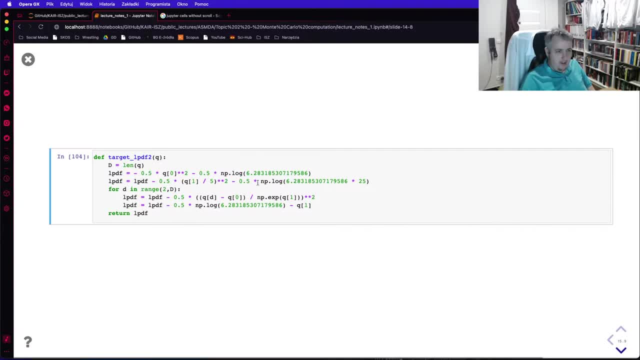 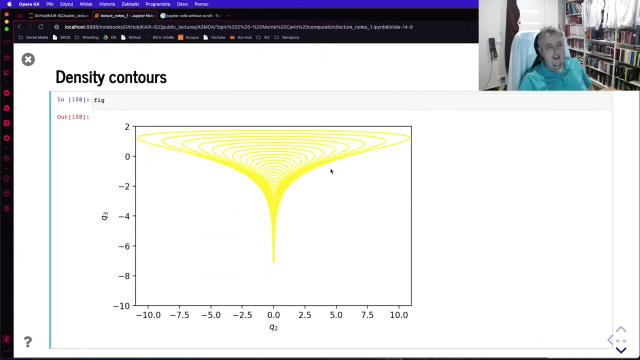 by the normal distribution. However, the further variables are modified by them. in this specific situation of twisting the shape of distribution, And the distribution, for example, between second and third variable, looks like this: that when q changes into small values, then we have an. 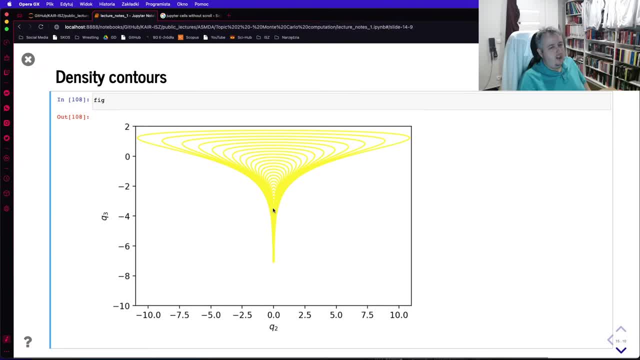 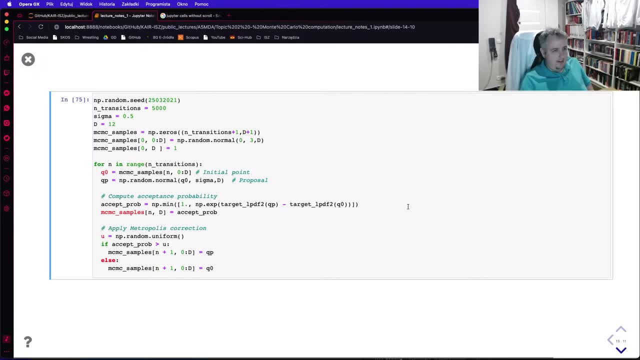 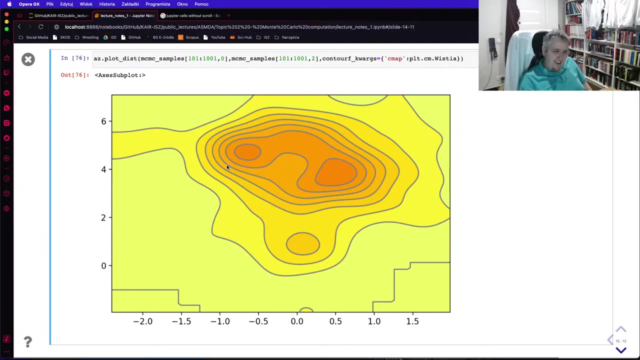 issue with moving of q2, because changes in both ways would be problematic. And again, we do the same: Metropolis transitions to get the samples. this is exactly the same code And we can plot the distribution that we get, which we can see. we kind of got what we wanted, or not. 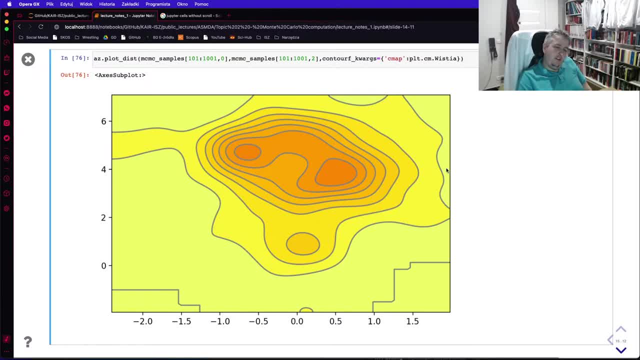 So we can plot the distribution that we get, which we can see. we kinda got what we wanted or not, because we didn't get this shape here. this is kernel density estimator here using the histograms in 2d is more difficult and so we use the. 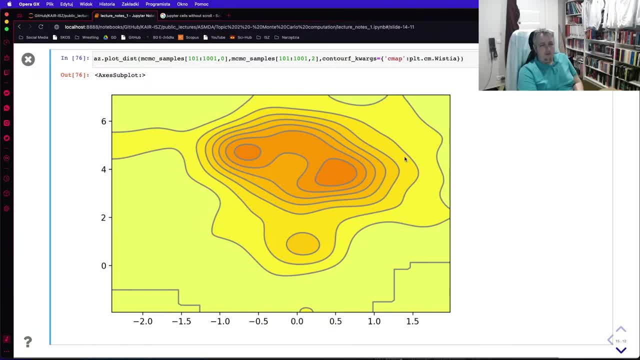 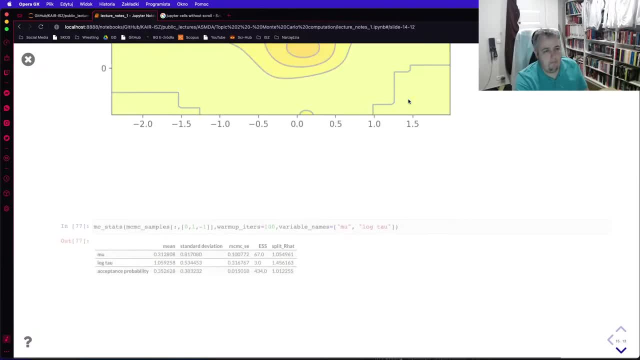 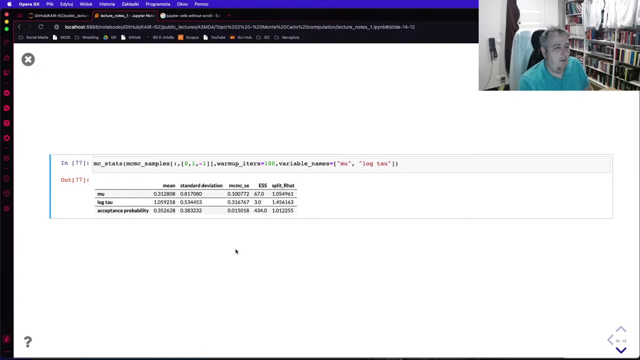 two-dimensional distribution relation using kernel density estimator and, as we can see, like: oh, there are two maxima or something like that, there are some problems and when we look at the stats then we can see that our expected value is we are getting large standard deviations. here we have very 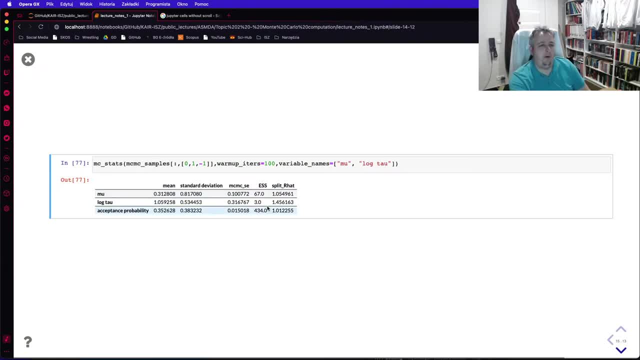 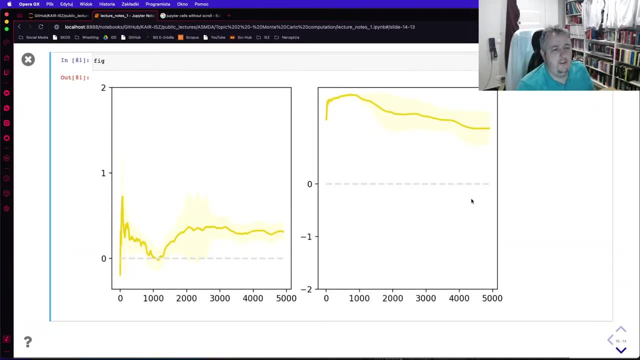 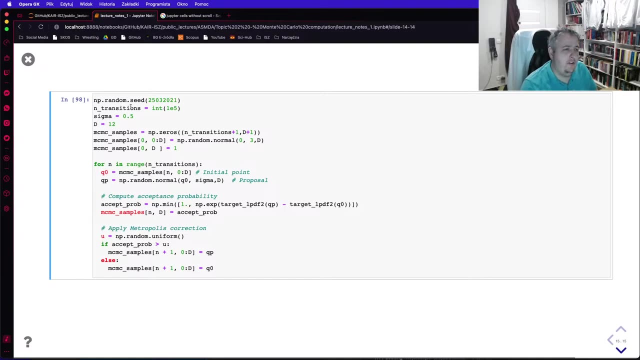 small standard expected sample size. this is a problematic situation. R hat is especially problematic and, as we can see, the convergences instead of going to zero values, it goes somewhere and if we increase the number of samples to try to cover it. so we have instead of 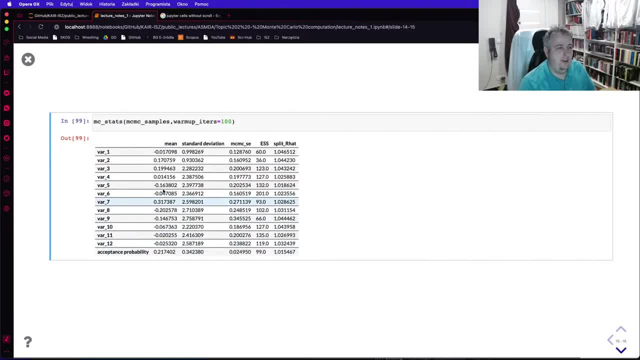 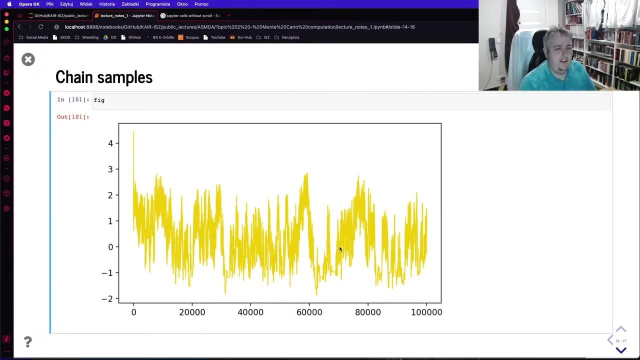 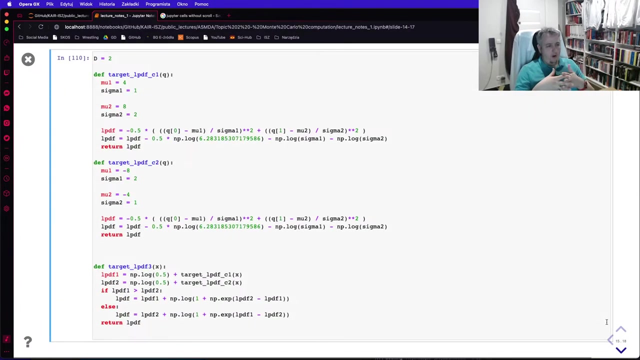 thousand, we have will get 100,000 samples and look over all the variables. then, as you can see, from 100,000 samples we get the. we don't getting anything good. we get a very small expected sample sizes and chain samples also not necessarily very informative in this situation. so this is a problematic 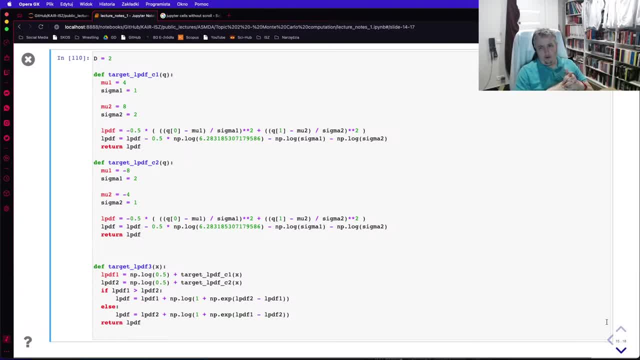 situation that needs special handling in order to cover and Markov chain. Monte Carlo might get stuck in difficult geometry that we've mentioned. Third example will be a metastable or multimodal distribution, which is generally a mixture of two distributions. We have two normal distributions, one with and and the 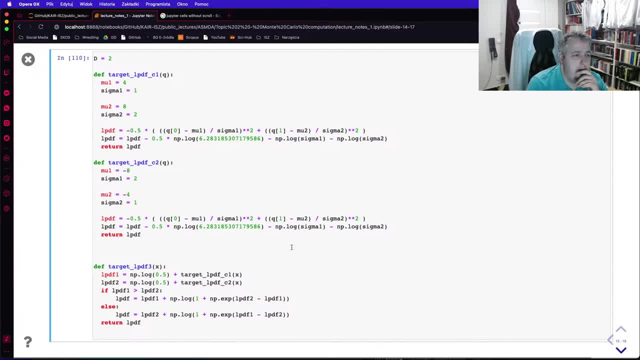 other one with the same standard deviations but with different, no inverse standard deviations and inverse mean. So we have the mixture of two distributions which has a simple covariance matrix structure which is not skewed. just we have two independent, two normal distributions with not correlated variables And we have the our log probability. 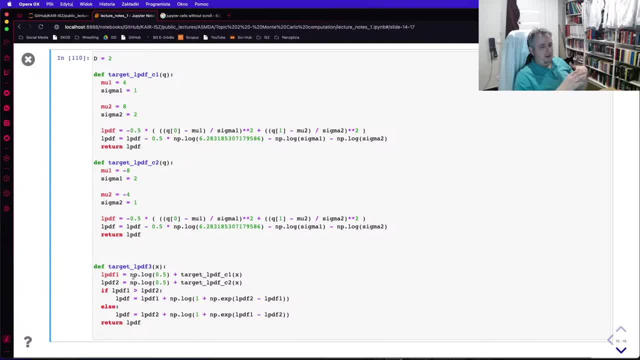 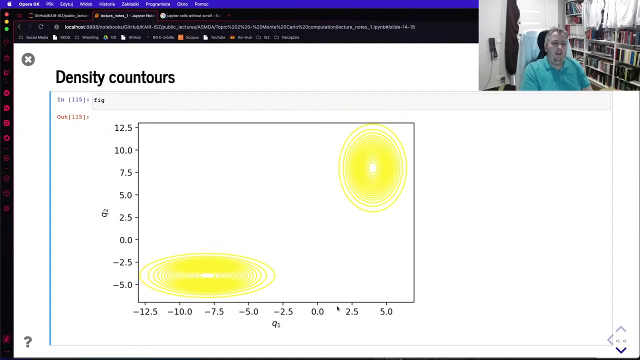 distribution and we have a probability of getting- I mean a mixture of probabilities to get. the insert value is either this one or this one, And the density controls look like this. so, as you can see, we have independent situations in both variables, here and here, so nothing really changes. And 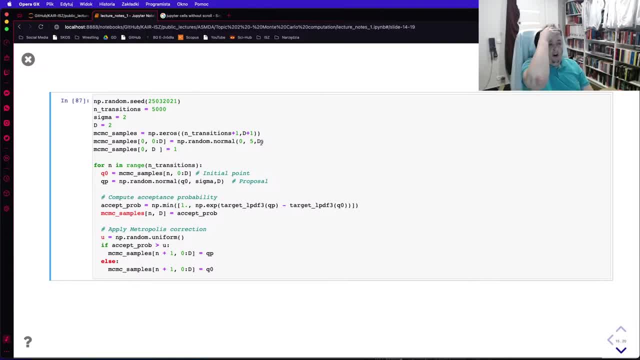 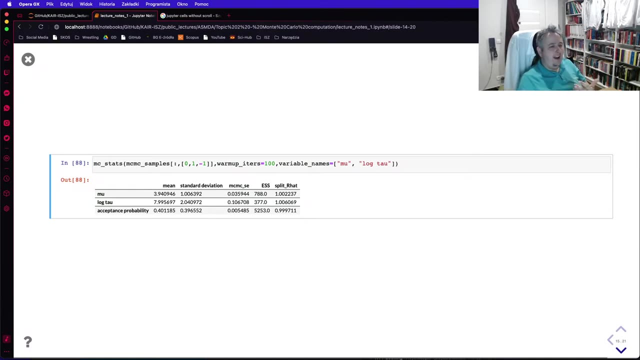 again same situations, same algorithm. We compute the expected probability and then apply Metropole corrections to get the proper transition And we get a situation that we get some kind of expectations from our distribution which have reasonable expected sample size and reasonable splitter hats. 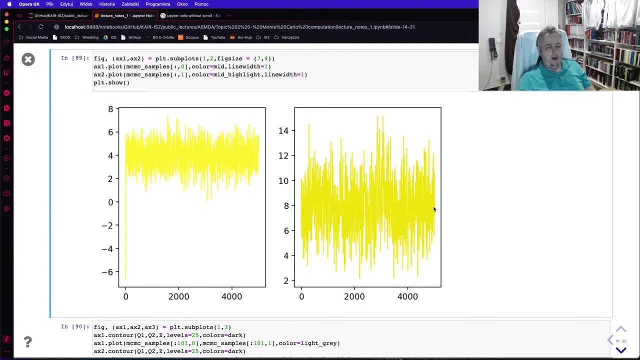 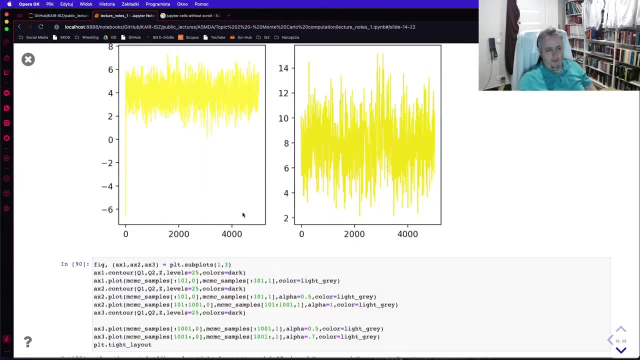 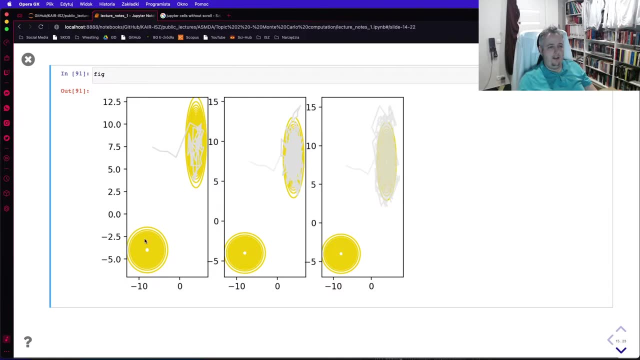 And the problem is that what we can see here, we've followed only one of the modes of distribution. As you can see here, moving to this mode completely avoids sample from here, so we do not get the proper coverage of the situation. 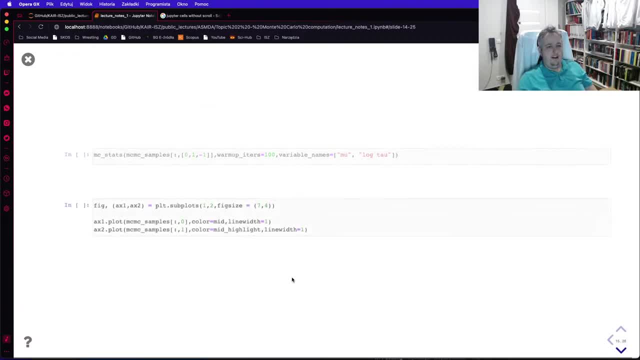 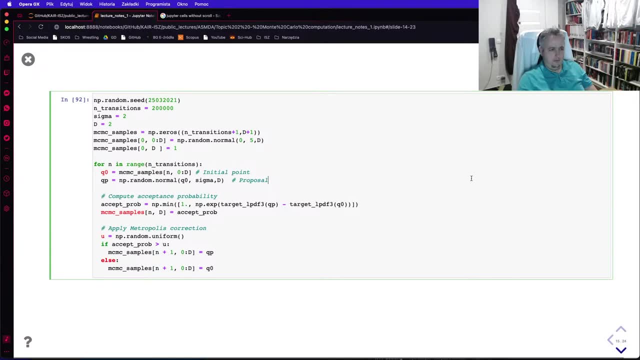 Increasing the number of samples of course gives us the Oh, I think I haven't run that one, This was, Let's run it again. So, as you can see, it takes some time because we need to do a fall of 200,000 samples to see if it will help us moving away from the transition. 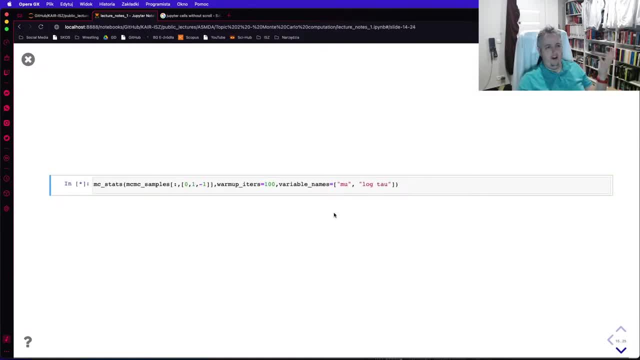 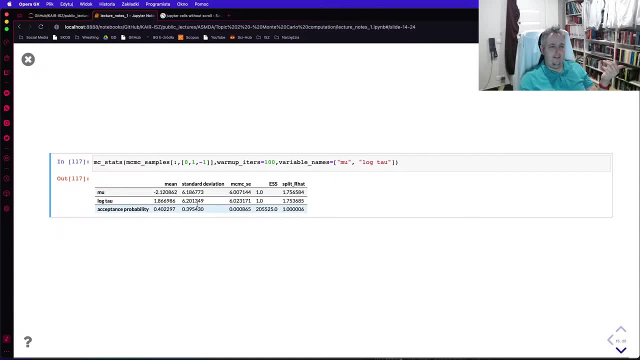 So when we move here, our statistics show that Again we have, We've got a lot of samples. Well, here we get the mean and And, as you can see, the expected sample size is weird. It is very small. 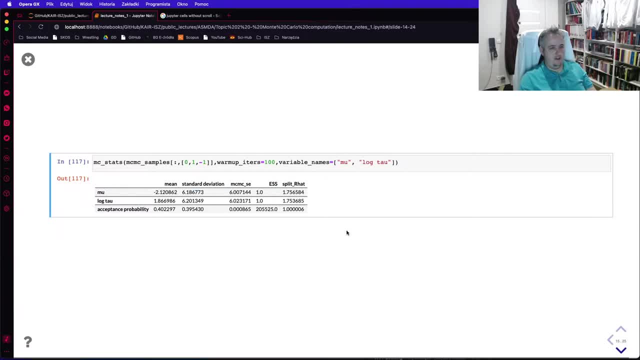 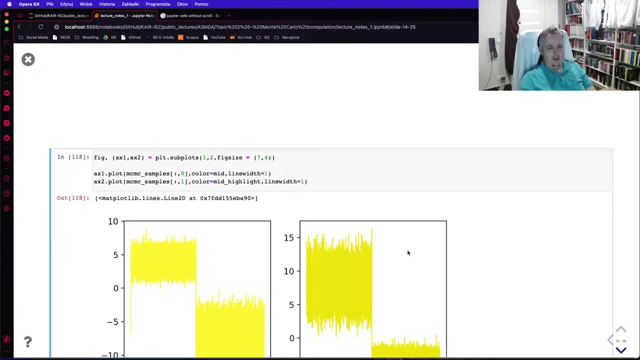 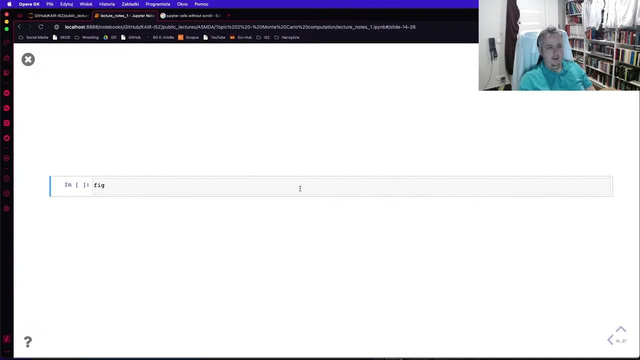 Very small, Large, Large standard division. There are genomes ahead. Why? Because, of course, our chains are not mixing, So in this case, our chains are just switching from one mode to another, Which I think I need to move to the code here. 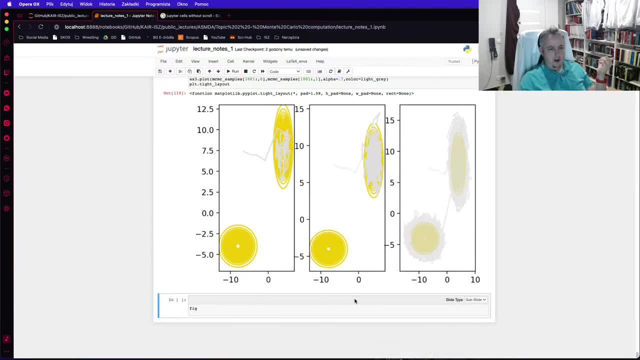 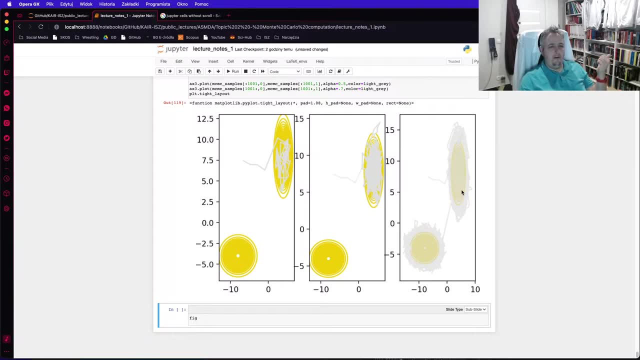 Because otherwise the contours won't be visible. Okay, As you can see, it starts here in covers And finally, after some large number of transitions, it finally moves to the, To the second mode. So this was a terribly sample situation. 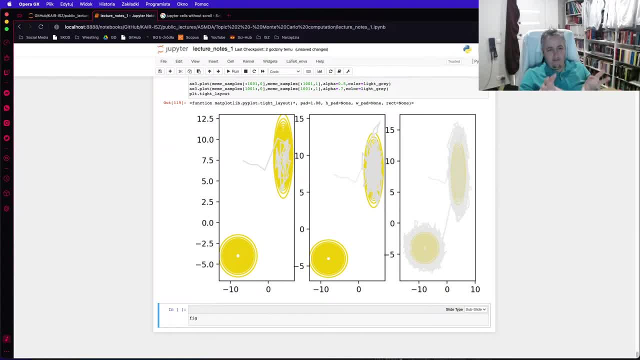 That we just didn't have a coverage of it, And this is a very complicated situation. And this is a realistic situation. The realistic situation that comes actually not from computation but from ill-defined model, Because generally, in almost 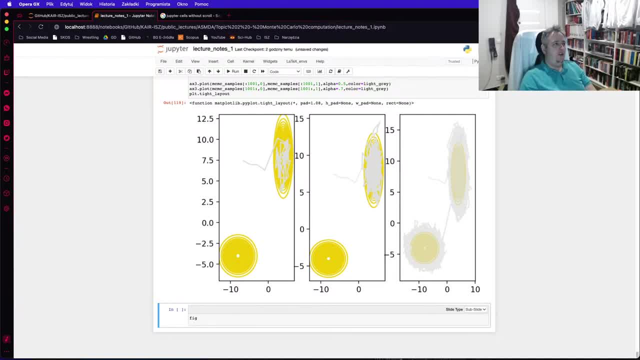 In most situations, when we have two models that are really likely, we should be able to remove them some way, For example by a specification of different prior distributions Or changing something else, And getting such situation is very difficult And, moreover, representation of them. 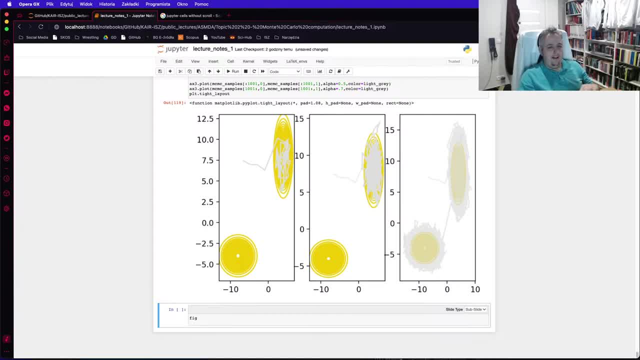 You cannot summarize such values, Because even if you compute expected values, it will be somewhere here And that says nothing. That's the problem. And in higher dimensions visualization will be much more difficult. This is not the case in, for example, machine learning. 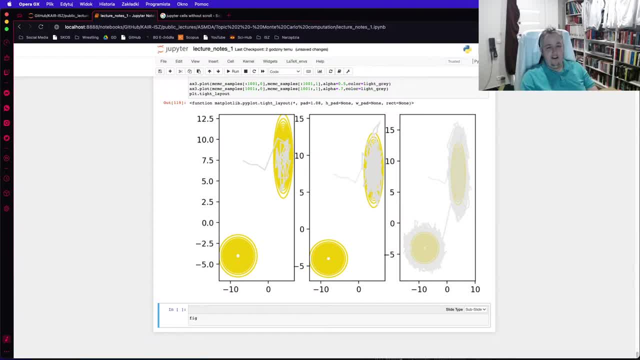 Where in deep learning networks you have very similar minima to each other. That finding one does not necessarily make it That it's worse than possibly others, That even global minima are not significantly smaller than the local ones. So here, just getting the representation. you don't have the information about the parameters of the system right way.